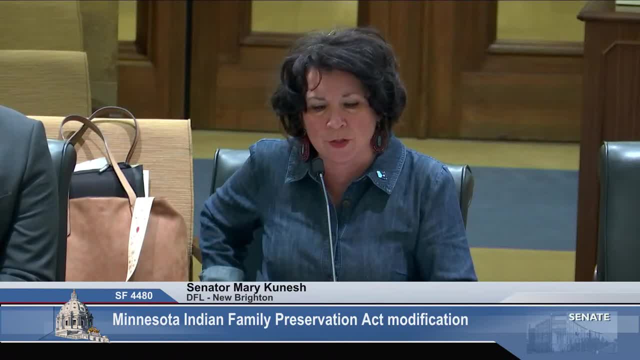 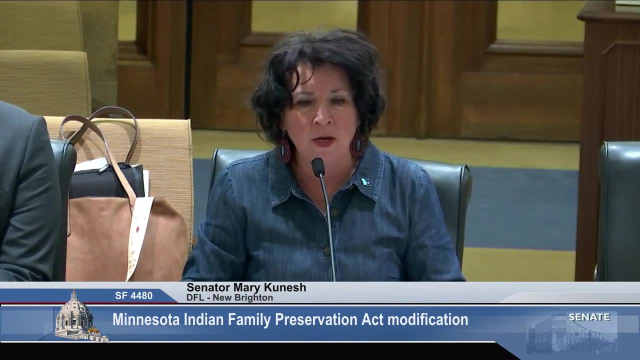 That was an urgent need here in Minnesota to ensure that, should ICWA- the Indian Child Welfare Act- go away at the federal level, our Minnesota native tribes and families have the preservation and the ability to keep an eye on what happens for their, their children. 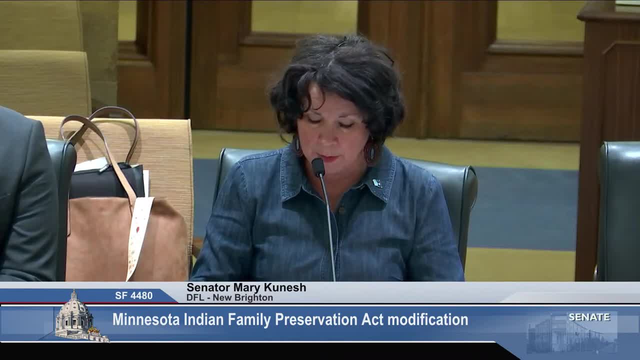 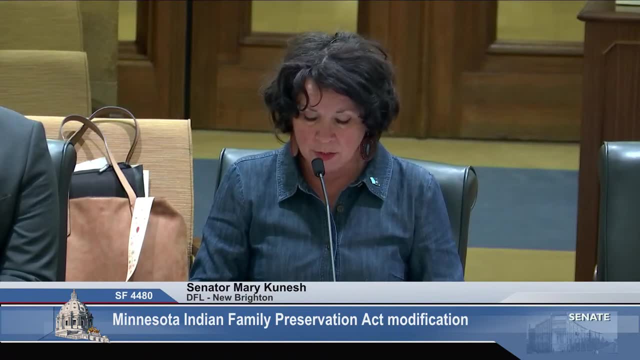 The federal Indian Child Welfare Act established procedures and requirements for child custody proceedings that involve an Indian child. The Minnesota Indian Family Preservation Act, or MFPA, was originally enacted in 1985 to strengthen and expand upon parts of ICWA Indian Child Welfare Act. 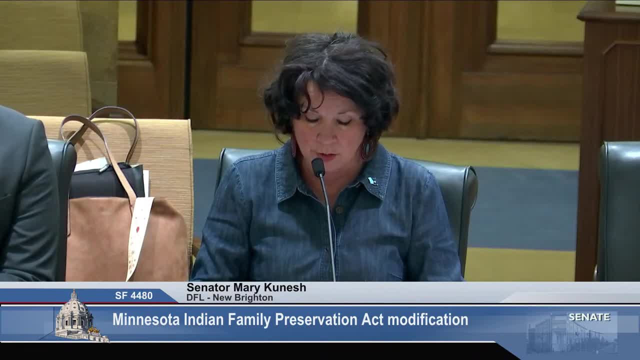 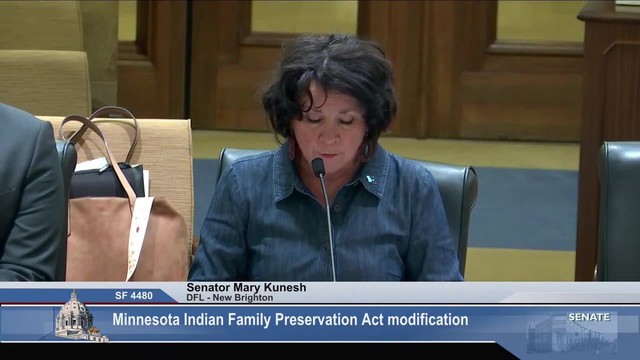 In the 2023 legislative session, the legislature codified ICWA into the state MFPA statute, Adding a purpose statement, and added additional definitions and clarifications. This bill in front of you- Senate File 4480,- further modifies MFPA by amending definitions and making technical and conforming changes. 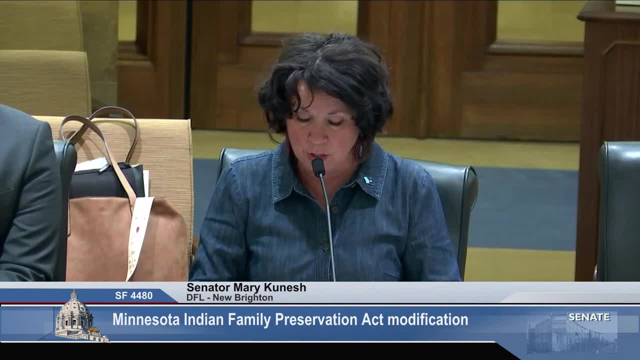 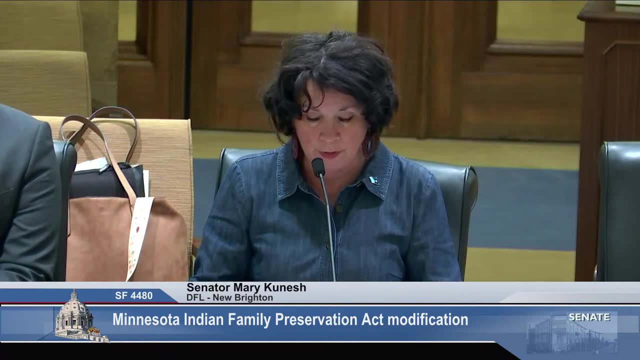 Additionally, the bill modifies notice requirements for child placement proceedings, inquiry procedures and the appointment of counsel in child placement proceedings involving an Indian child, And there's There's three different, There's three different areas that it makes the major changes in. 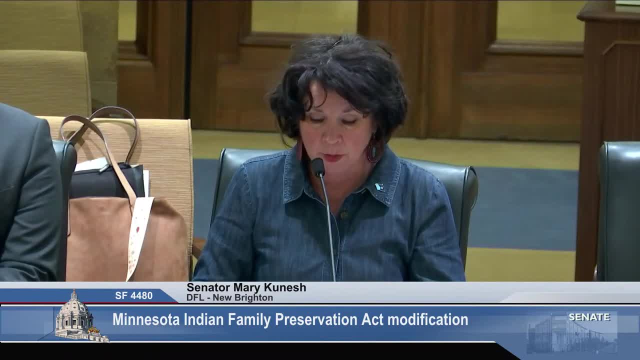 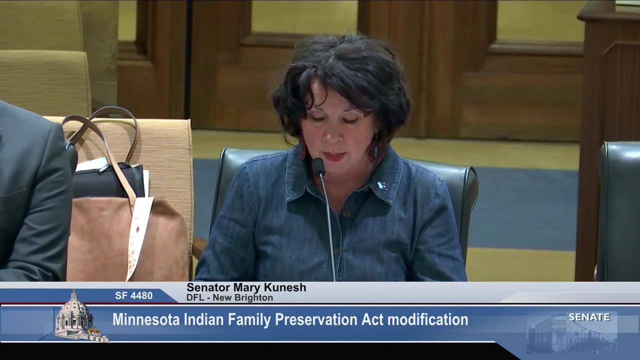 The first is changes to facilitate compliance with ICWA and MFPA. An often overlooked issue is compliance with ICWA at the federal level and then at the state level. MFPA in child custody proceedings involving an Indian child that are not coming into court system as a child protection case. 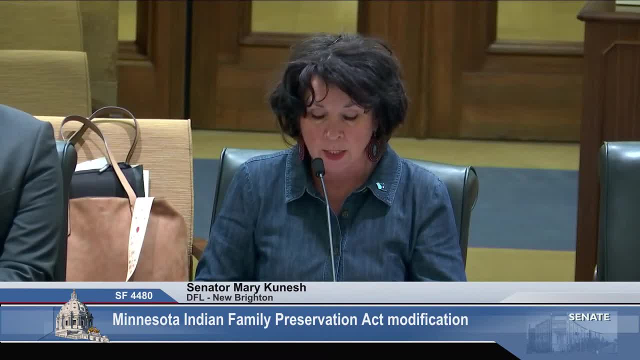 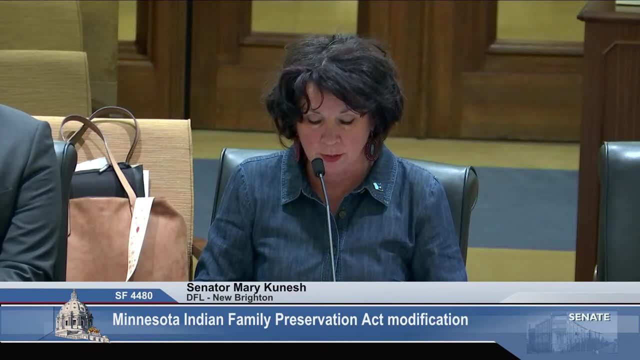 Finally, between the state and state law. the state law must apply to all cases where a child defined as an Indian child is or may be removed from care, control and custody of the Indian child's parents or Indian custodian, who cannot have the child returned to their care simply by asking. 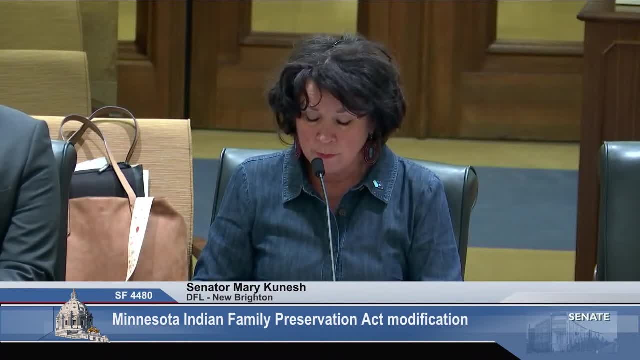 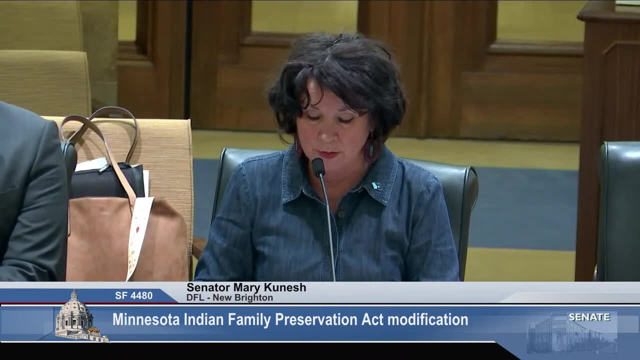 This does not include custody between parents, Custody between parent and Indian custodians or juvenile offenses that are not status offenses. Any other situation that may result in the child being released from custody is not a public offence. The purpose is to ensure that this is not a public offence. 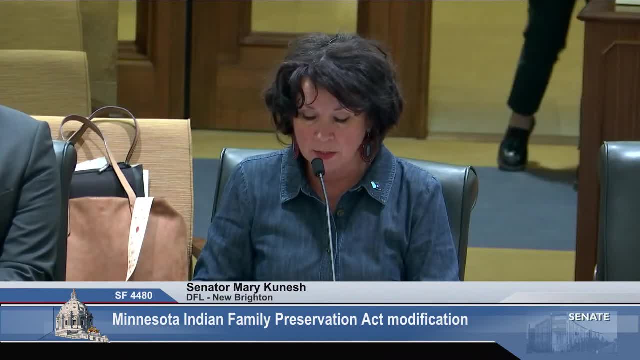 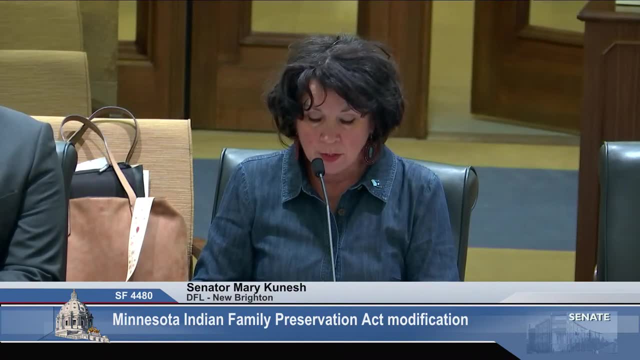 Okay. in the child being removed from the care, custody and control of the parent or Indian custodian are cases where ICWA and MIFPA apply. The 23-24 MIFPA Phase 2 work focused on making compliance with ICWA and MIFPA. 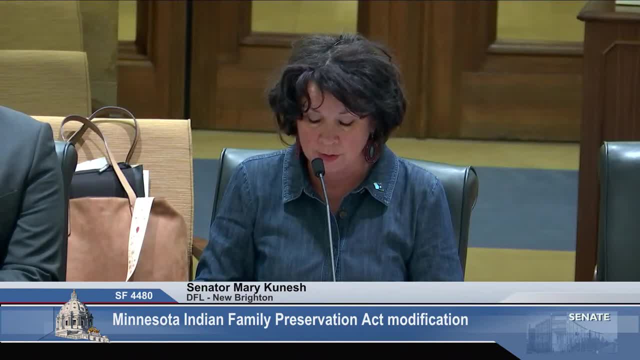 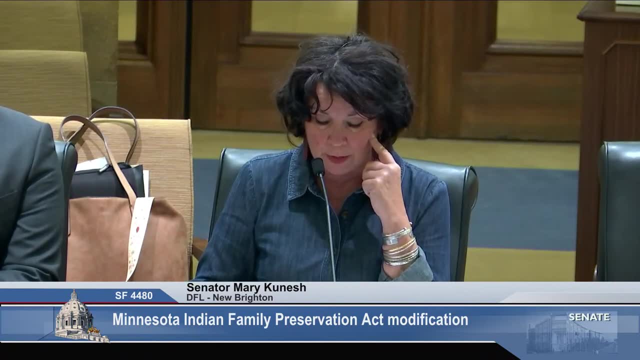 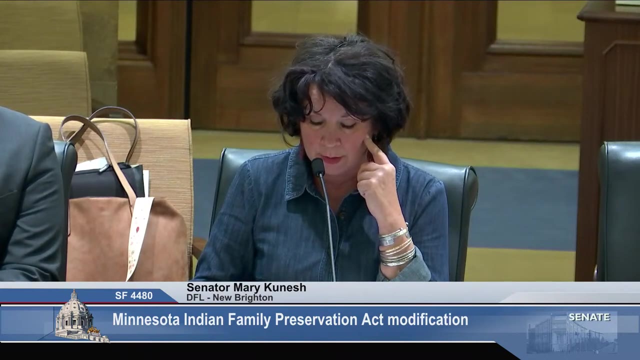 more clear and easier to understand for practitioners in areas of law where compliance with ICWA and MIFPA are often overlooked. So specifically, Statute 260.761B requires courts to inquire into lineage possible membership on the record during the hearing. 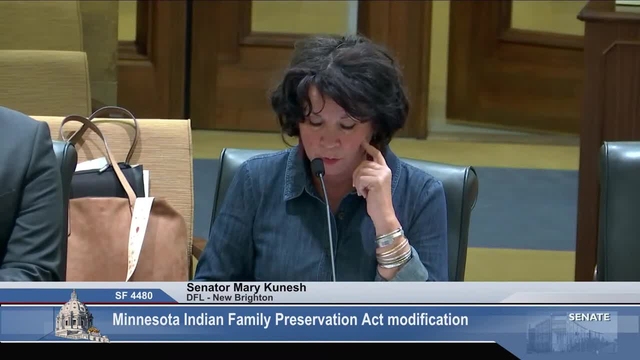 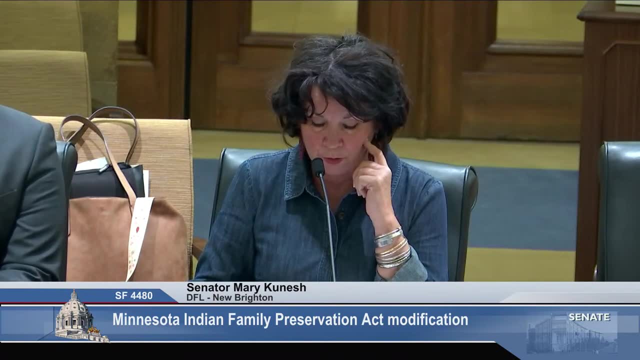 260C.178 requires compliance with placement preference during emergency removal. 260.761 clarifies notice provisions. 260.762 clarified active evidence. 260.763 clarifies effort provisions, especially for voluntary placement. Then it goes on to others that clarify jurisdiction. 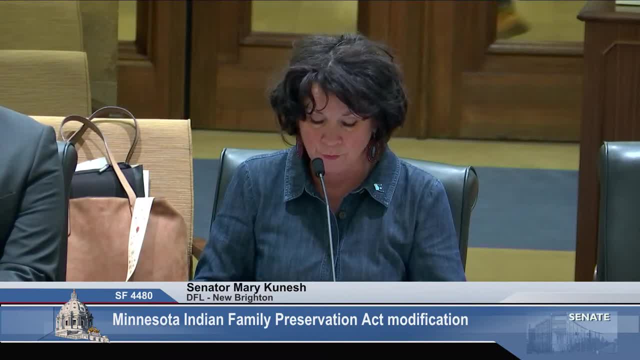 including transfer to tribal court, good cause to deny transfer and deference to tribal. determination of exclusive jurisdiction. appointment of counsel for parents, Indian custodians and children in non-CHIPS cases. the return of out-of-home placement costs to parents. 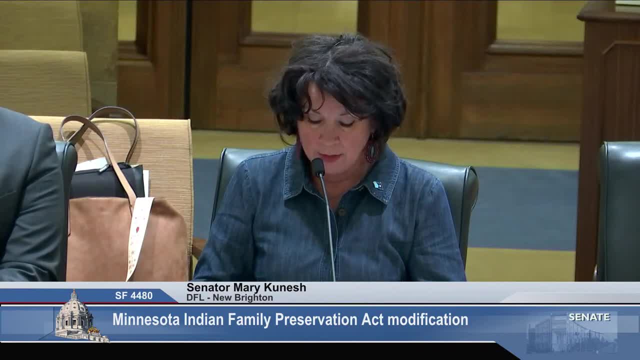 if anywhere proceedings have been invalidated, and then allows court to impose sanctions and costs where proceedings are invalidated, where appropriate. That's all under changes to facilitate compliance. Then they worked on improvements to facilitate tribal participation in hearings, which is really, really important. 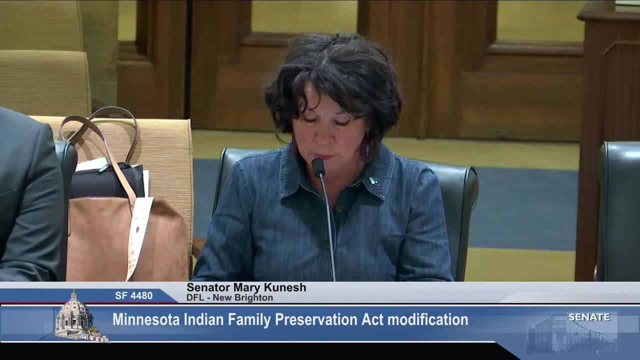 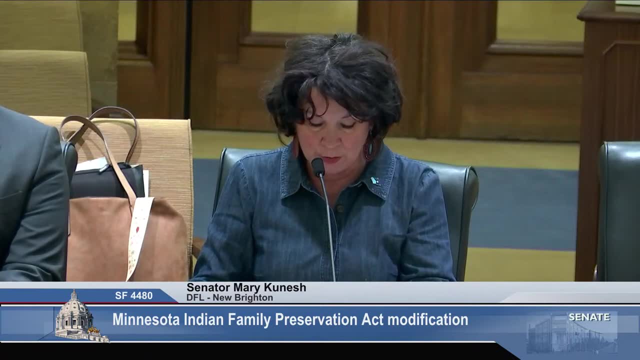 And we learned that there are a large number of struggles that tribes, especially those located out of state, face when trying to participate in hearings. The following changes were made to facilitate triage tribal participation in hearings. So under 260.775, subdivision 20A. 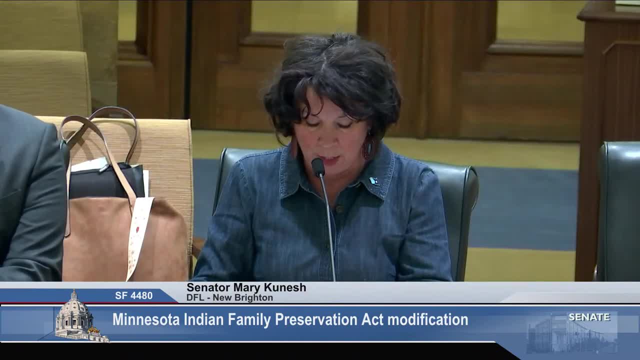 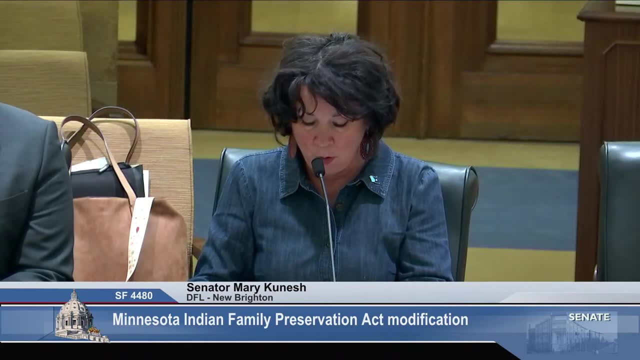 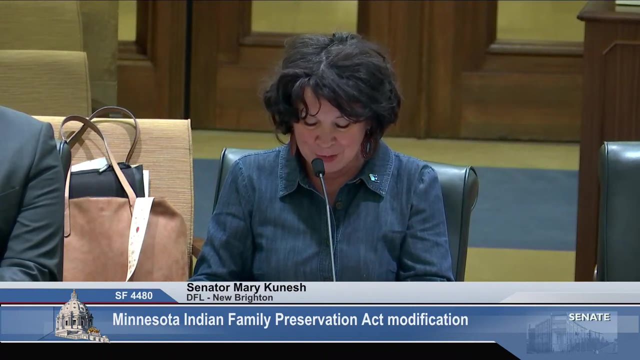 tribal REFs are not engaged in unauthorized practice of law. And then in 260.771,, tribal REFs are exempt from pro hoc vice, no filing fees, do not have to use FE file and service systems and may appear remotely. And then the third part. 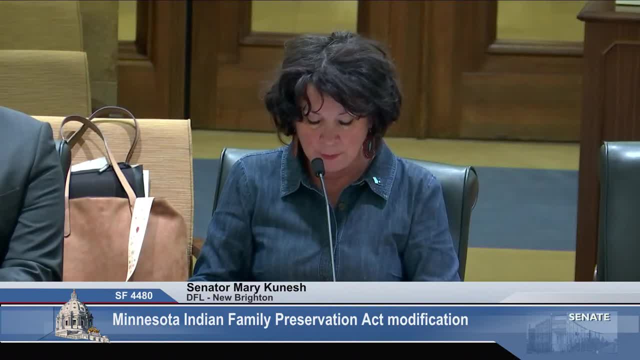 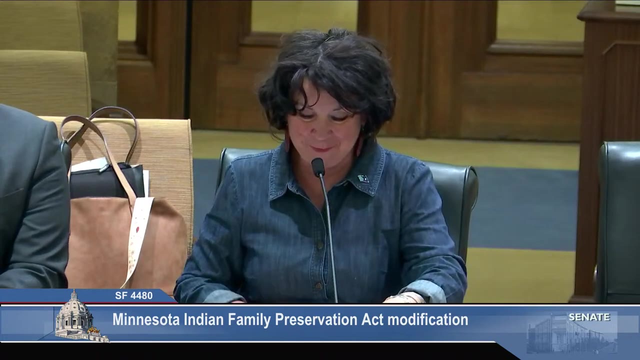 is the study of child placement and permanency. A multidisciplinary team will evaluate what permanency, timelines and practices in child welfare proceedings will be looked at. And, Mr Chair and members, that is the bill. Thank you, Senator Kunish. 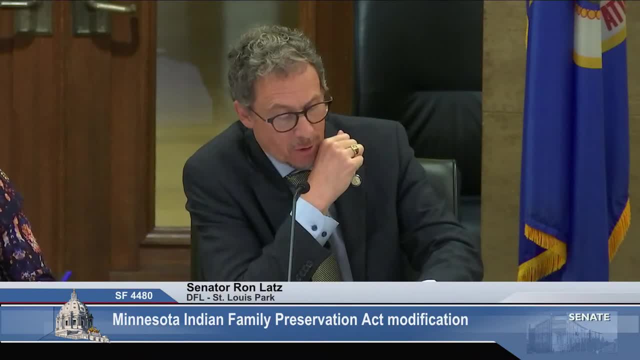 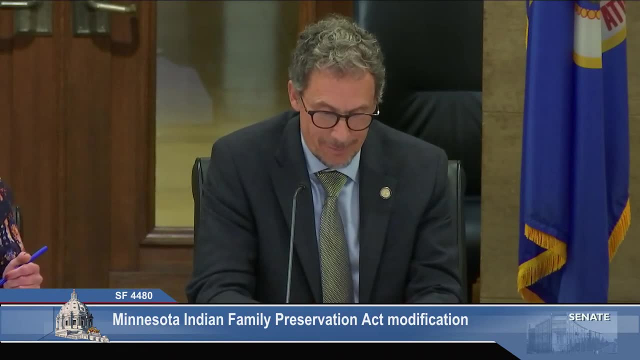 Counsel, can you identify for us if there are any particular parts of the bill or all of the bill that are within our jurisdiction? Ms Primo, Mr Chair and members, it's the whole bill. Thanks for narrowing it down for us. 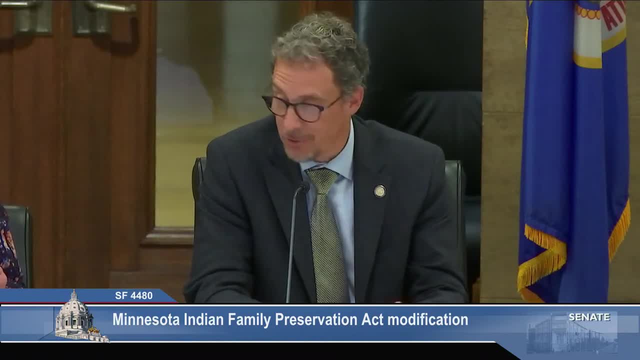 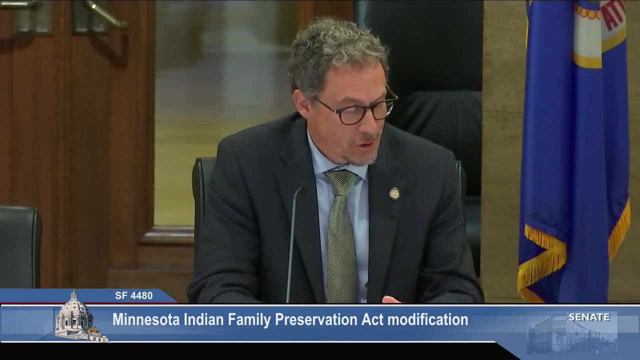 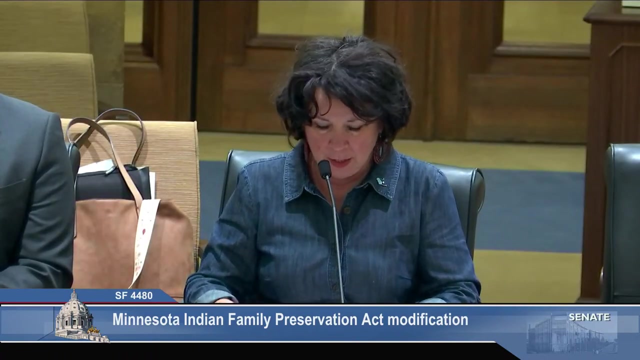 Members, you got 30 seconds to read 47 pages. All right. And Senator Kunish, could you give us a brief description of the A3 amendment then as well? All right, The A3 amendment, as I said, does provide for clarification. 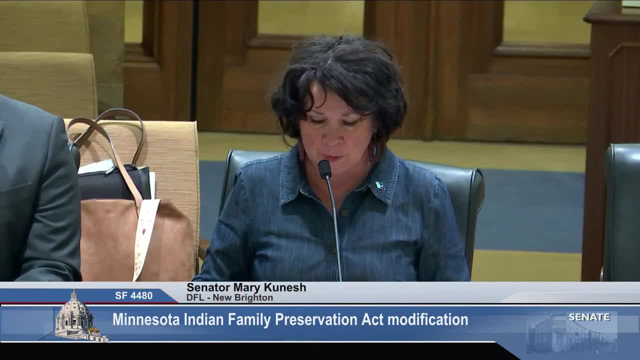 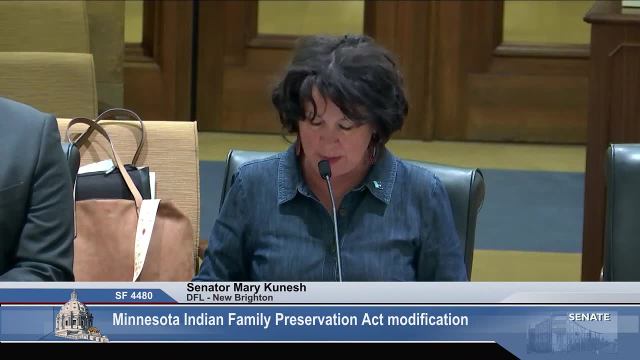 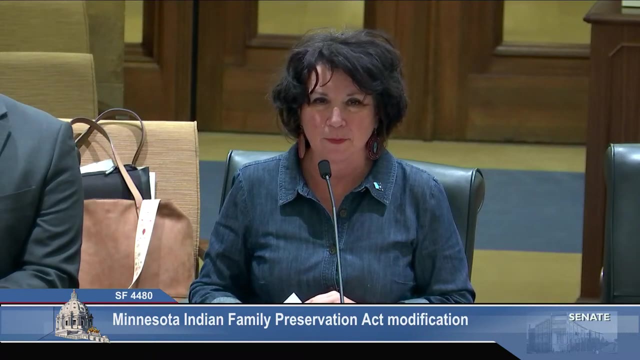 and use of specific words Within custody and placement And just puts the bill in the order that it needs to be in. Thank you, Before we take on the amendment, we'll hear from the testifiers that are here: James Ryan from the Mille Lacs Band of Ojibwe. 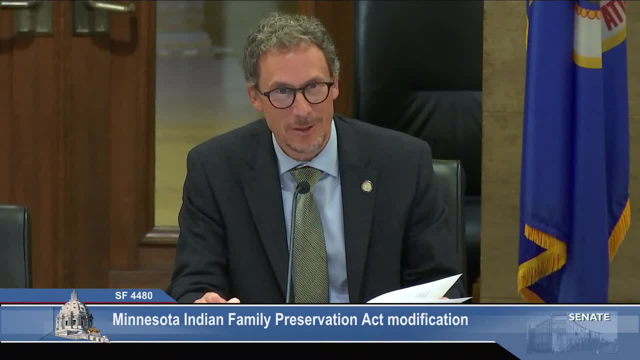 Deputy Solicitor General. Mr Ryan, welcome to the Judiciary Committee. Thank you, Mr Chair. Good afternoon. I am James Ryan, Deputy Solicitor General for the Mille Lacs Band of Ojibwe. Thank you for having me. 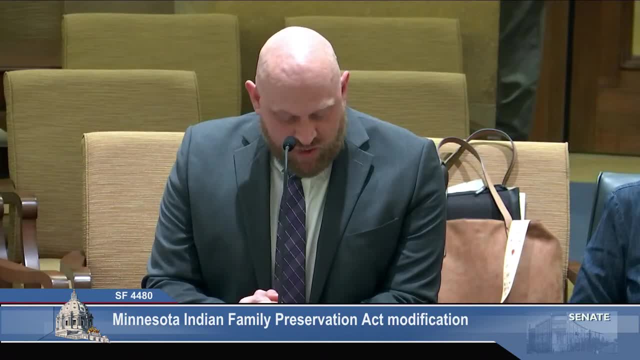 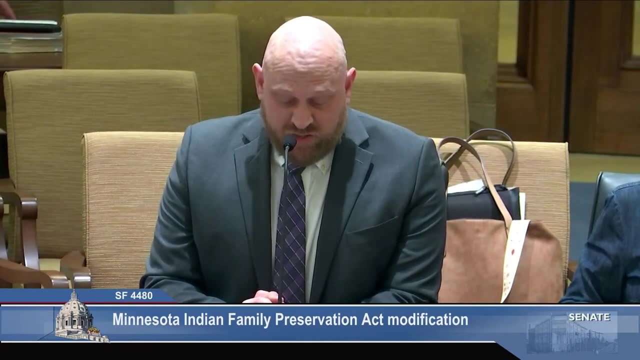 Thank you for having us And thank you for consideration of this bill. Minnesota law recognizes that the best interests of the children, or Indian child, are interwoven with the best interests of the child's tribe. Why is that? The child's tribe is where a child 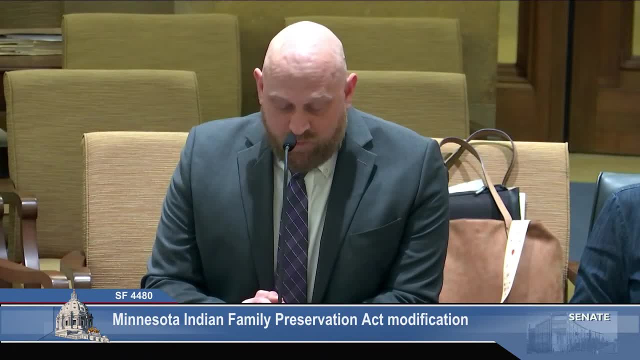 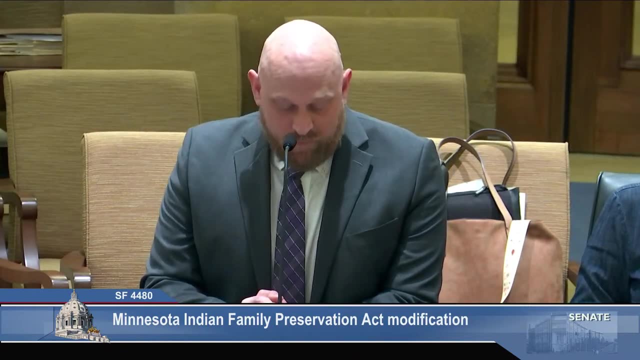 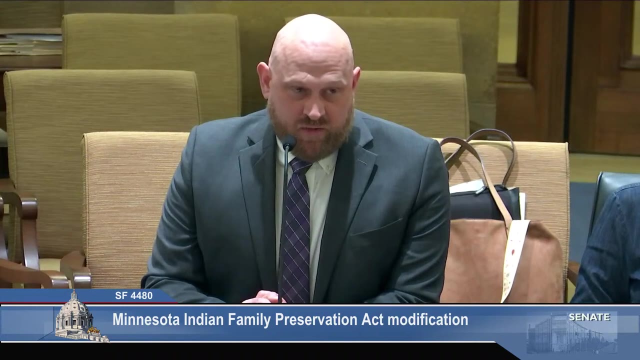 can find a sense of belonging. It is important for the child's sense of identity And it is where the child feels at home. Knowing of one's culture is not the same as living in one's culture, And so the Mille Lacs Band. 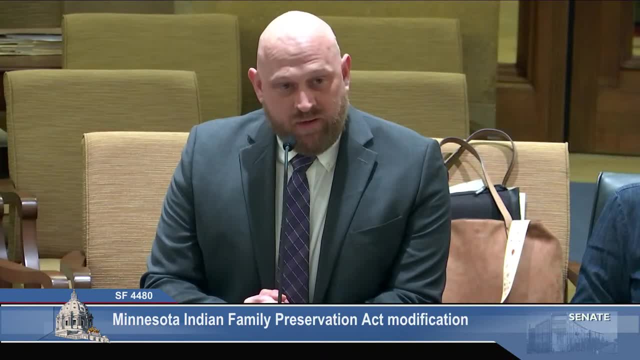 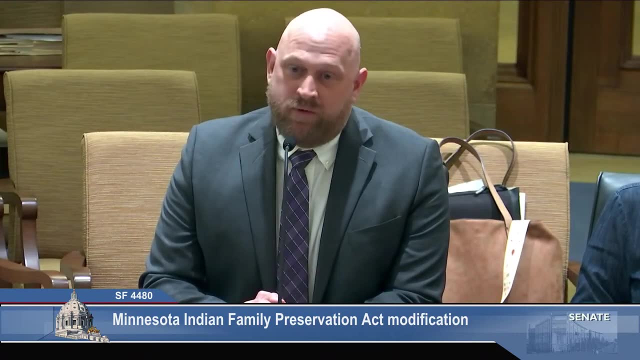 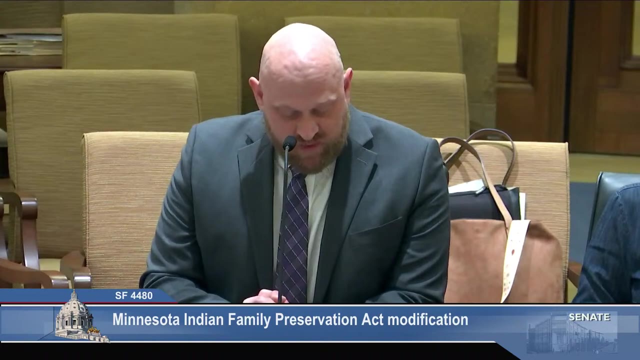 has worked very hard to keep their children with their families and in their communities. Thank you to all of you that have helped with the Mille Lacs Band and other Minnesota tribes to accomplish those goals, especially to Senator Kunish for her tireless work. 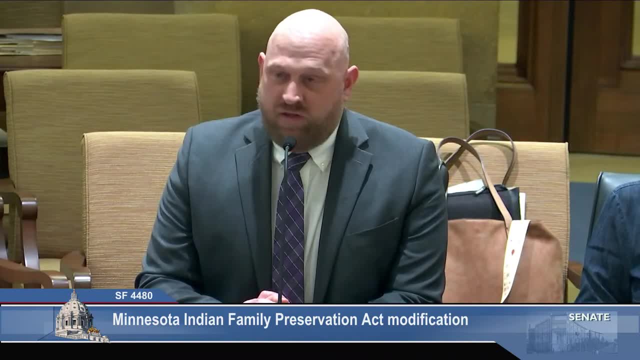 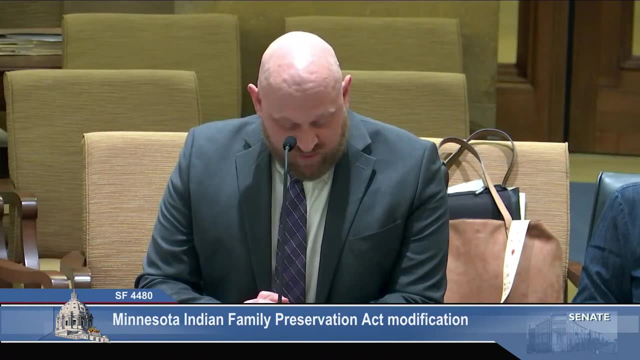 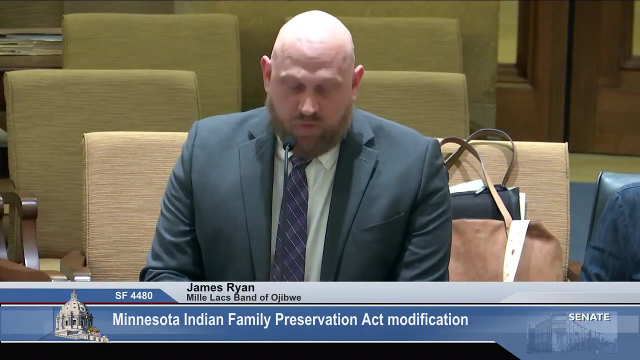 on behalf of tribes. Thank you also to the work group that helped draft this bill And thank you all for your consideration of it. Last year, when federal protection for Indian children and tribes were at risk, Minnesota stood up and said: no matter what happens. 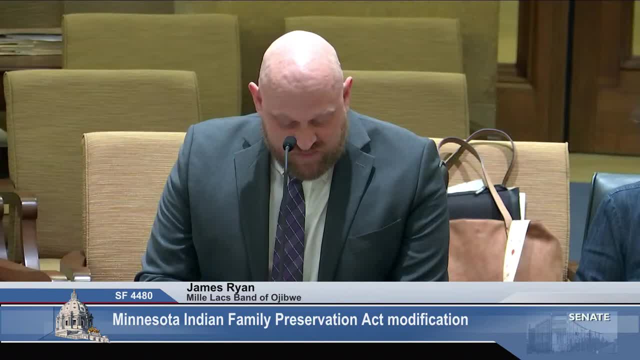 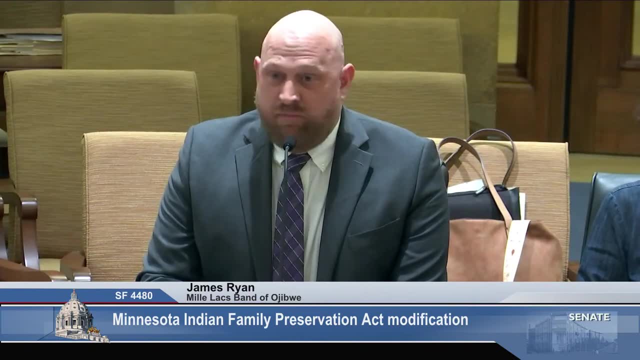 in Washington DC, Minnesota, will respect the needs of Indian children and tribal sovereignty. Thank you for that work that was done in MIFPA last year. Because of the hurried nature, there was a lot of things that we were not able to get to. 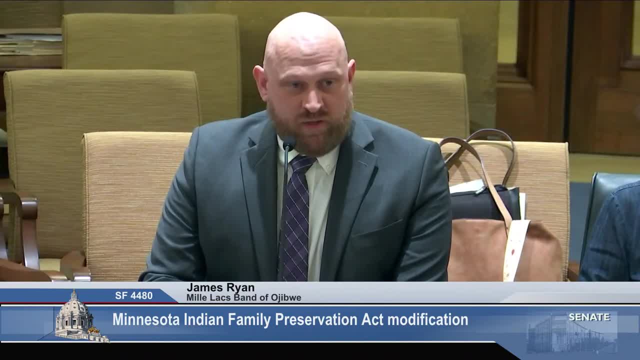 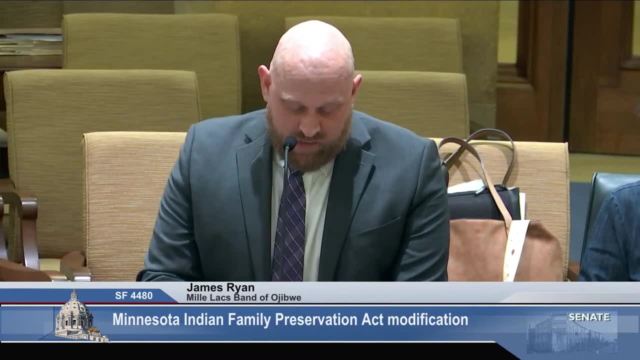 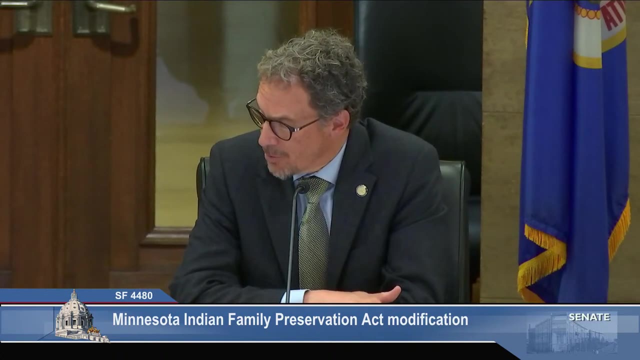 but are still vitally important for Indian children and tribes. The Mille Lacs Band asks that you support this bill and thank you again for your consideration. Thank you, Mr Ryan. We have some other testifiers, I think all of whom now are on Zoom. 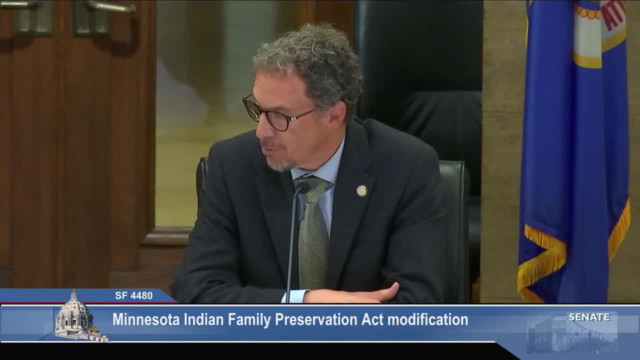 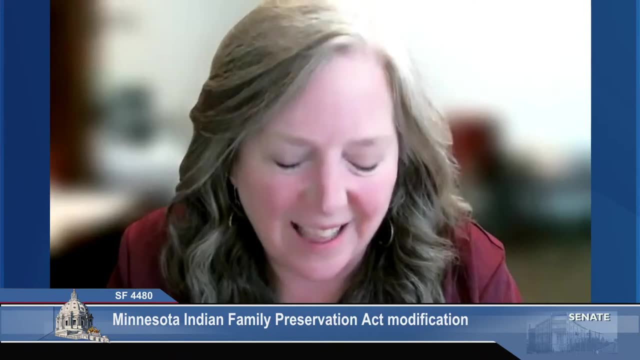 Rebecca McConkie-Green, Chief Judge of the Leech Lake Band of Ojibwe Tribal Court. Welcome Judge. Thank you, Mr Chair and committee members. It's an honor to be here and thank you for taking the time. 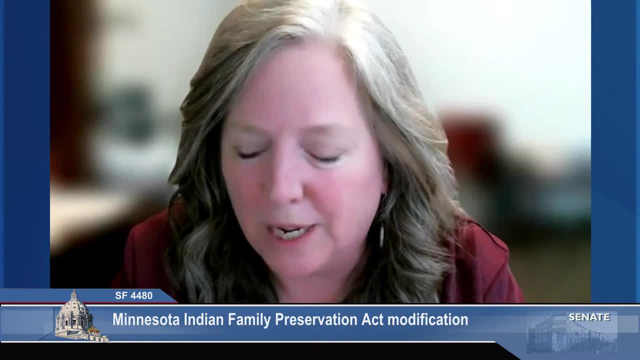 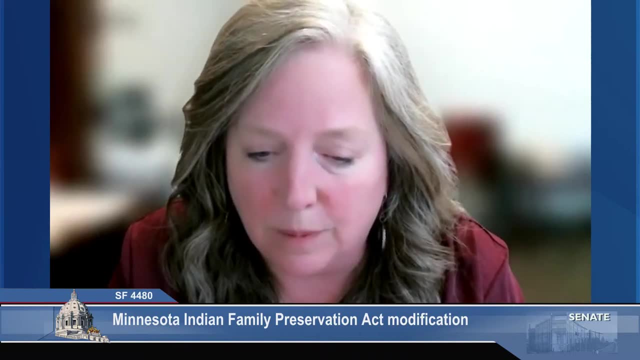 out of your very busy schedule this week to hear this bill. We truly appreciate it And I want to start, as Mr Ryan did, by expressing gratitude for this committee and for the Minnesota Legislature in general, led last year by Senator Coon. 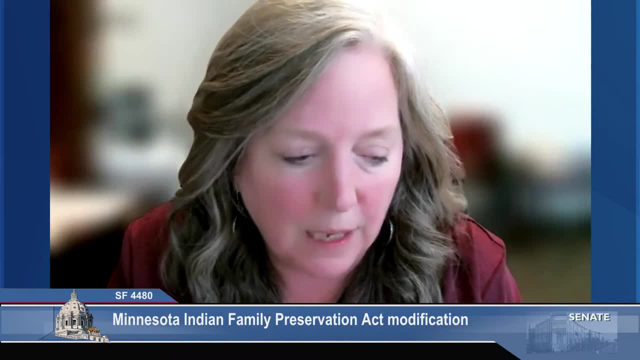 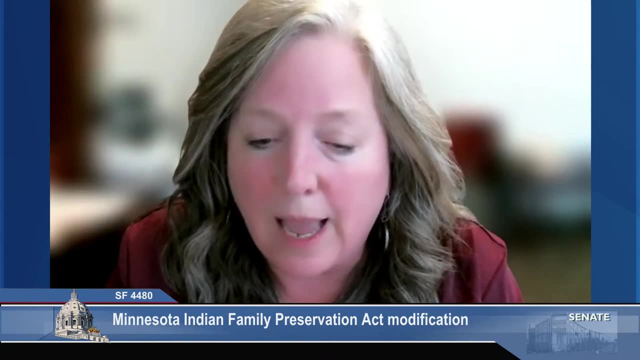 and I want to thank Senator Coonish on our MFPA bill that we brought, and Representative Keeler to keep the protections of the Indian Child Welfare Act in play in Minnesota. Happily we had a good outcome in the Supreme Court decision. 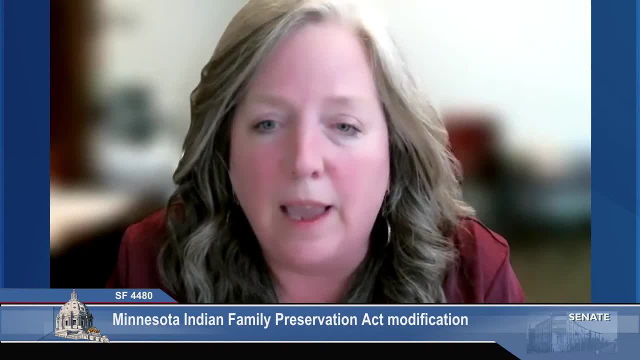 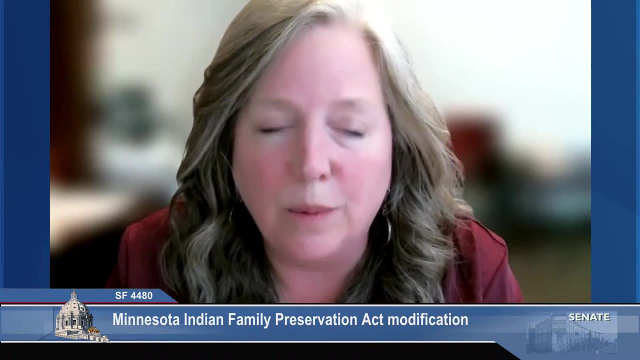 but it was a huge relief to know that the state of Minnesota listens to the Indian people and was willing to step up and ensure that those provisions remained in place, As we talked about last year when I testified, I believe I told you that we would be back. 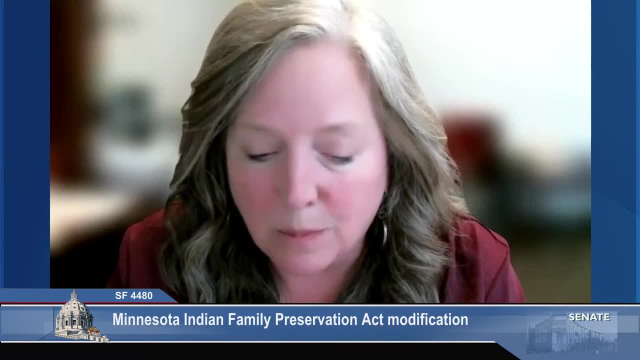 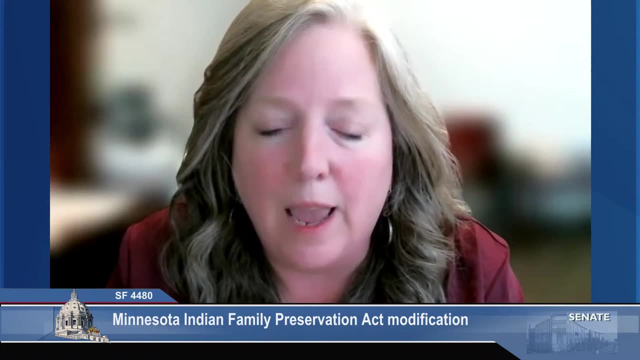 And I had said that we would be back because when the testimony came from members of the community and tribal leaders there was a lot of pain. that was difficult testimony to hear And unfortunately there was difficult testimony from community members who were testifying in their 80s. 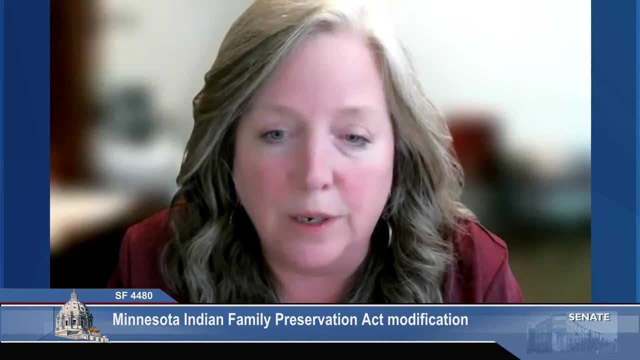 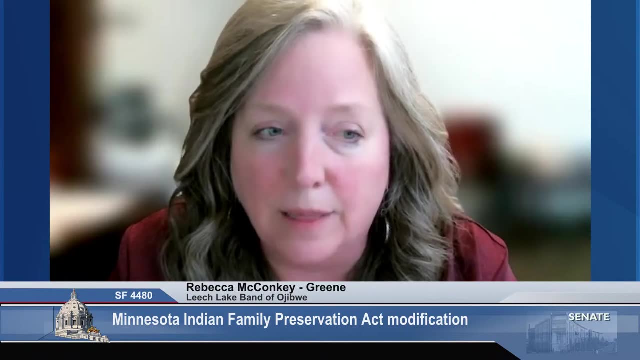 and community members who were testifying who were younger young adults and teenagers. So we knew when we were hearing this testimony that we would need to come back, that, while the Indian Child Welfare Act and the Minnesota Indian Family Preservation Act, as they currently stand, are extremely important, 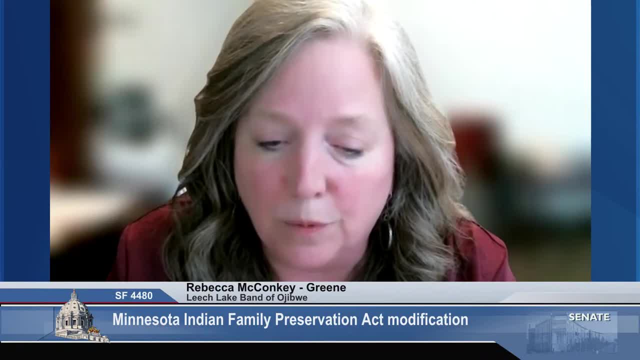 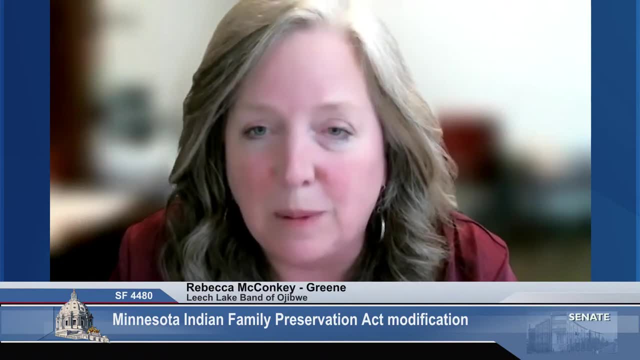 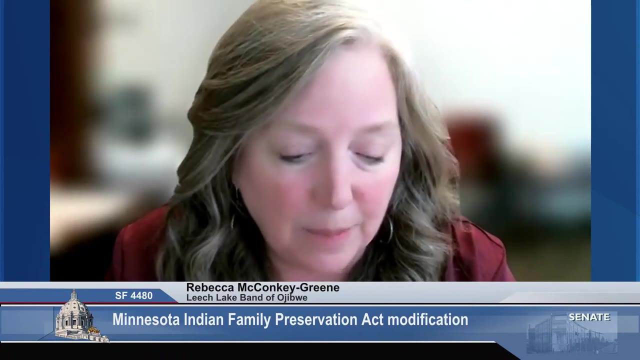 we need to do better. There are areas that we can improve. So we started right away after the legislative session last year and we had 187 people on our larger working group. Not all of those people came all the time, but everybody got the updates. 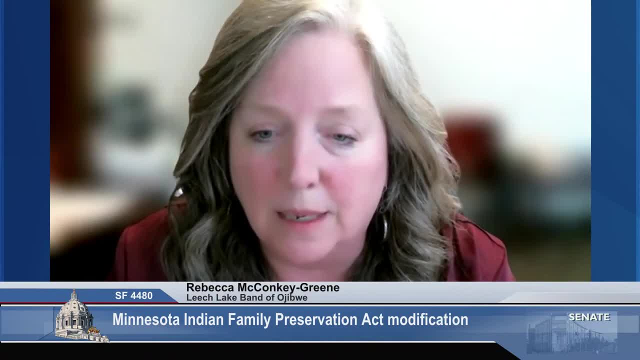 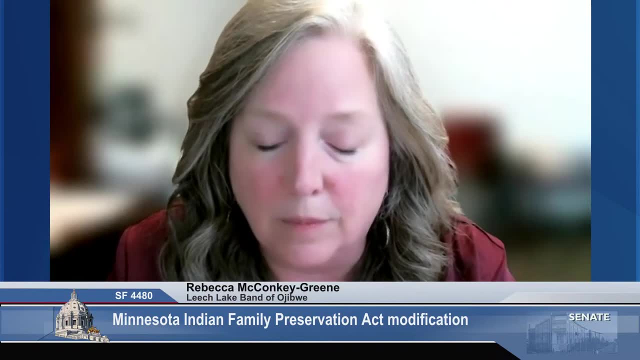 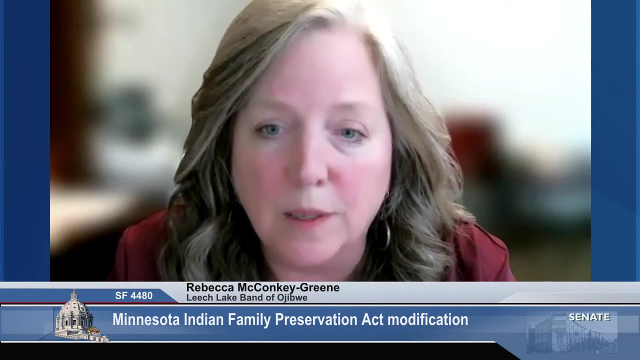 and we broke into 10 subcommittees that drafted the work that is before you. Of those 187 people, we had a number of people from the Minnesota County Attorneys Association, from MACSA, from AMC, from Minnesota Bar Association and then, of course, 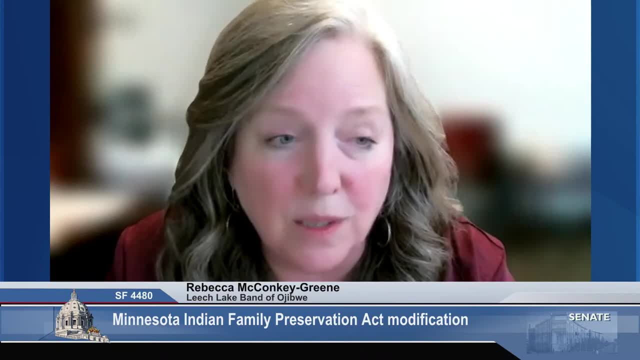 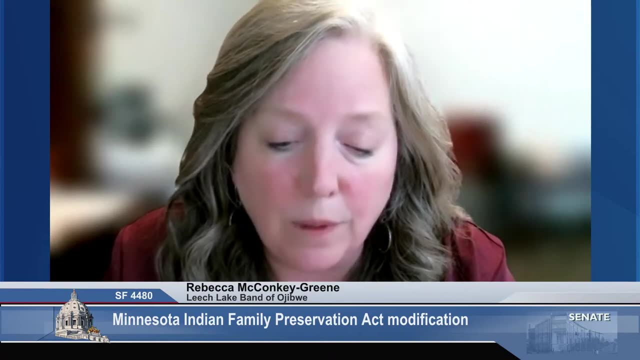 from all of the tribes in Minnesota and the organizations that serve Indian people throughout the state of Minnesota. We sought input from all of those people because one of the things that we were working on this year is making sure that, while the Indian Child Welfare Act and MFPA 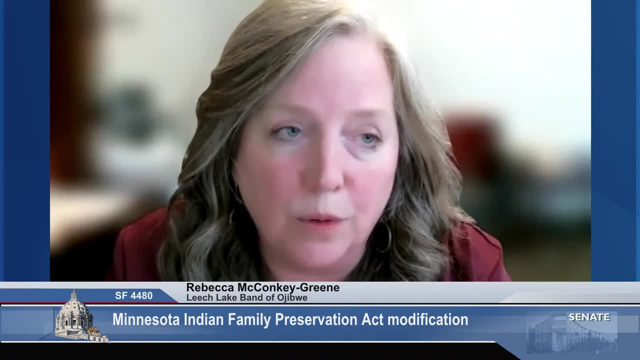 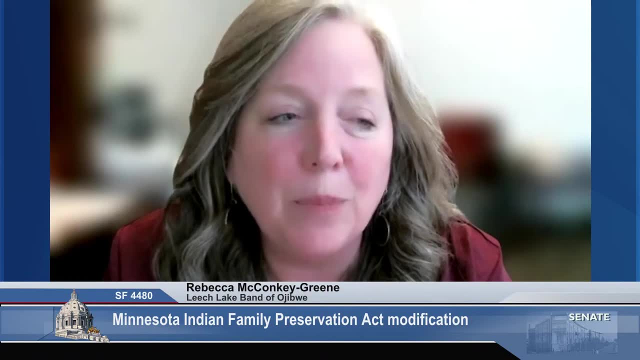 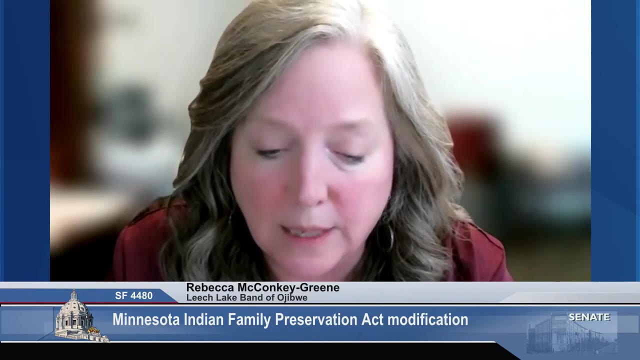 have always applied to any proceedings where children could be taken from the care and custody of their parents, so other proceedings besides child protection. law and practice has tended to focus most on child protection and we need to make sure that families are protected in other types of proceedings. 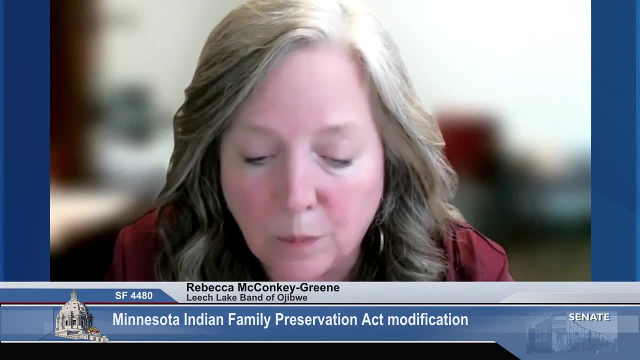 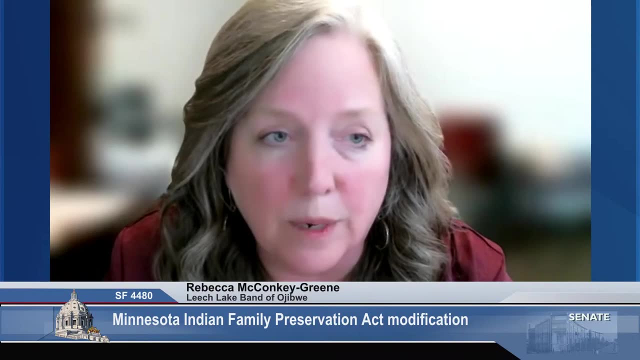 like third-party custody and probate proceedings. So we wanted to make sure that we had adequate input to see the struggles that the various people that come into contact with the system would have and to make sure that we were relaying things adequately. So the bill before you, I believe, does that. 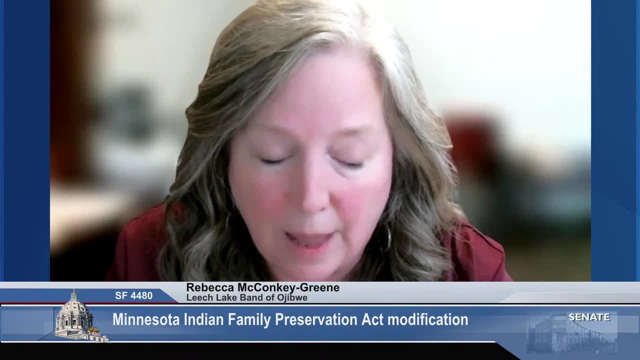 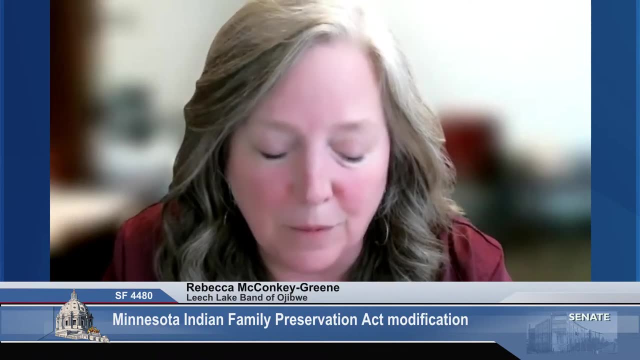 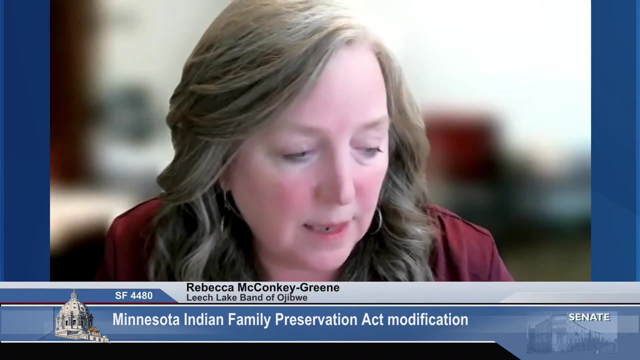 We have a number of provisions that we're very happy to have in the bill and believe will go a long ways towards making things better in the future for Indian families and clear for the people that practice in state court proceedings so that there will be less question. 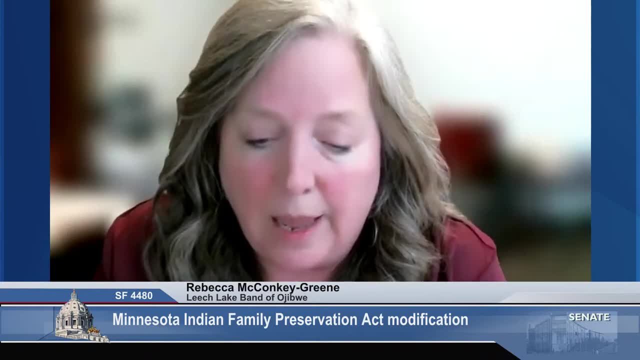 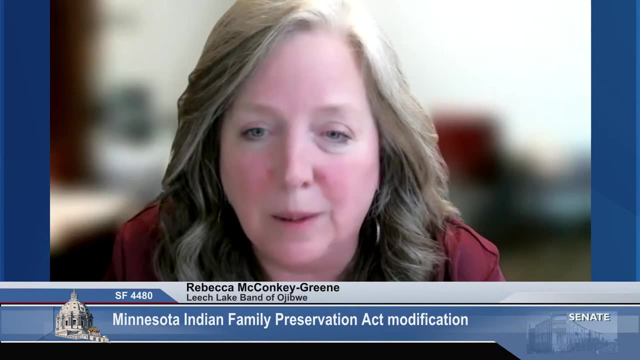 and it will be more obvious what needs to be done With that. unfortunately, there were a number of things that we didn't, we weren't able to bring forward this year. They need a little bit more work. So I'm going to say once again: 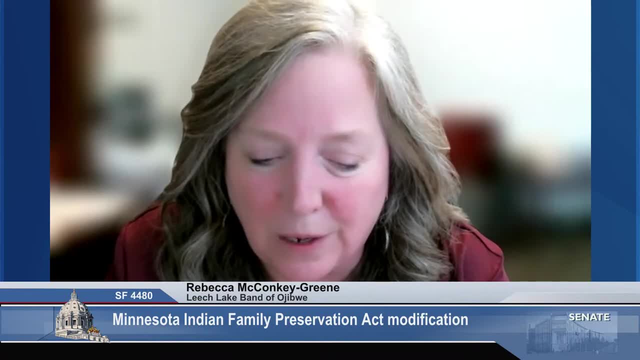 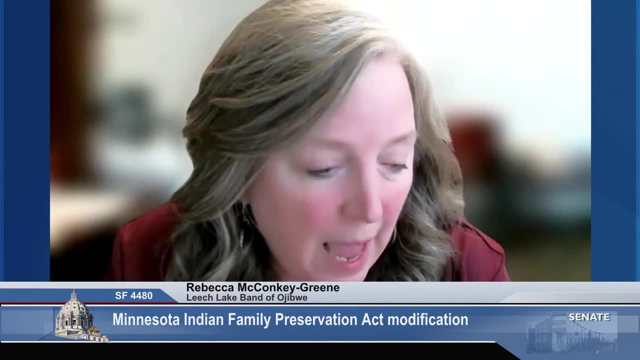 we hope to be back in front of you next year and probably in the years to come, as we continue to work with all of the people connected to the system to make sure that we have good practices in place, And so I am certainly prepared, when you're ready, to go through any portions of the bill. 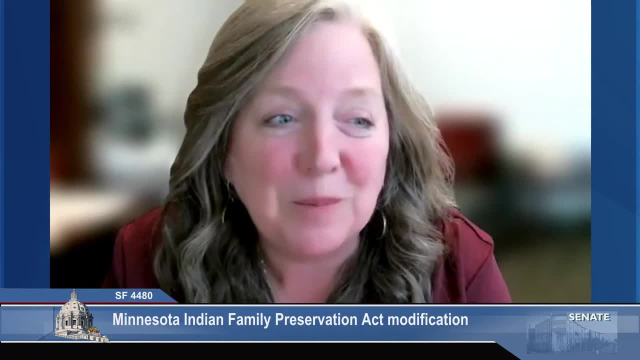 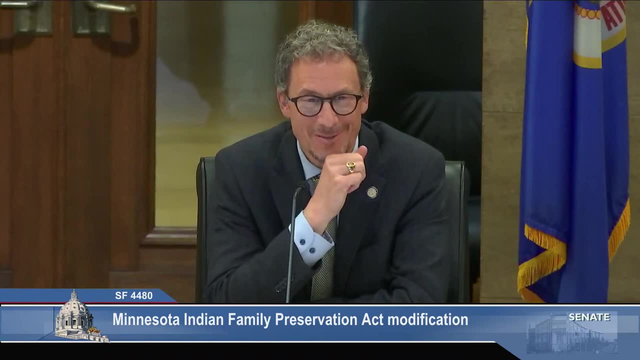 that you'd like to discuss, Thank you. Thank you, Judge, for your testimony. Our next testifier is Lori York, Executive Director of the White Earth Nation. Director York. Good afternoon Chair and committee members. So, as you recall, 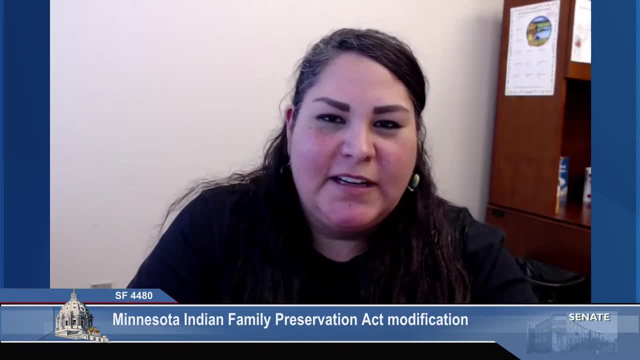 last year, under the threat to the pending US Supreme Court decision, the Minnesota legislature had passed amendments to MFPA that ensured all protections of ICWA would remain in Minnesota. We just wanted to take a little bit of this time to thank you and thank the Minnesota legislature. 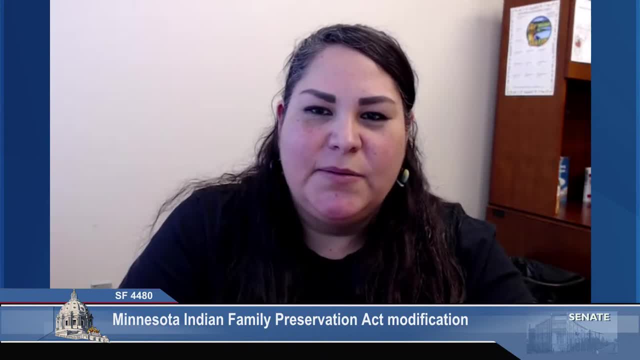 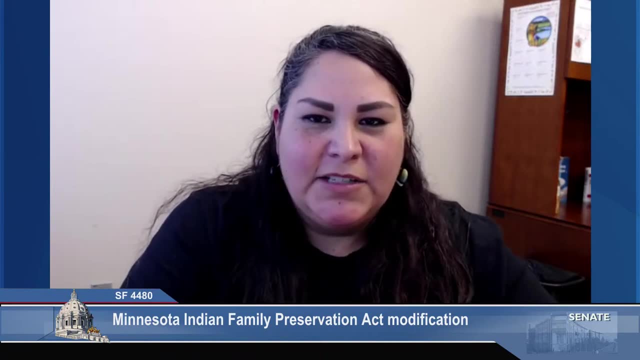 for your leadership, ensuring those protections. Your responsiveness to the wishes of the tribes and the testimony of tribal leaders and Indian people set an excellent example for our nation. This year's bill authored will improve practice in a manner that ensures greater protections for Indian children. 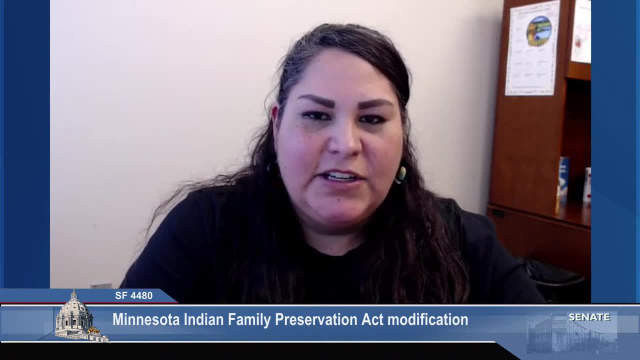 their families and tribes in the following ways. This legislation provides many practice improvements as it inserts language into several areas of law where ICWA and MFPA apply but are often overlooked. It provides a mechanism for appointment of counsel to parents and Indian custodians. 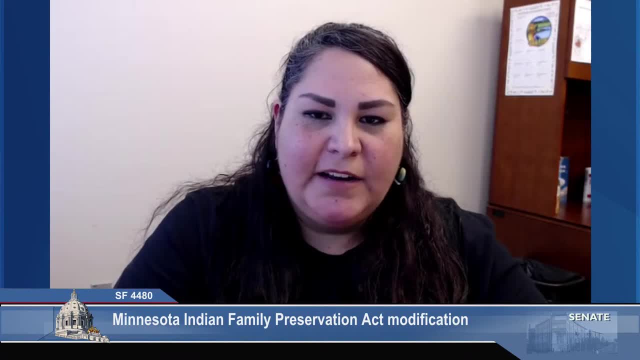 and Indian children in areas of law where counsel is already provided for them is not already provided for them. It clarifies notice provisions and improves access for tribes. It also ensures that tribes are able to provide input to the petitioners and the courts about what it is truly in the best interest. 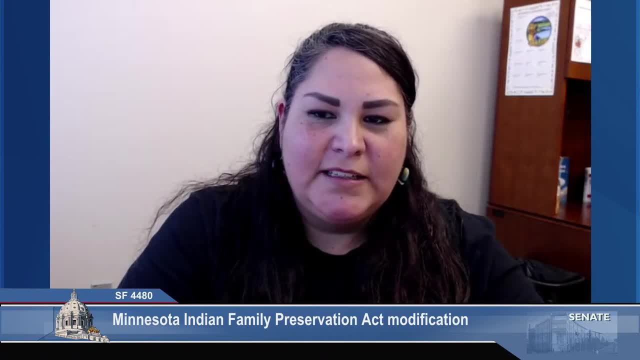 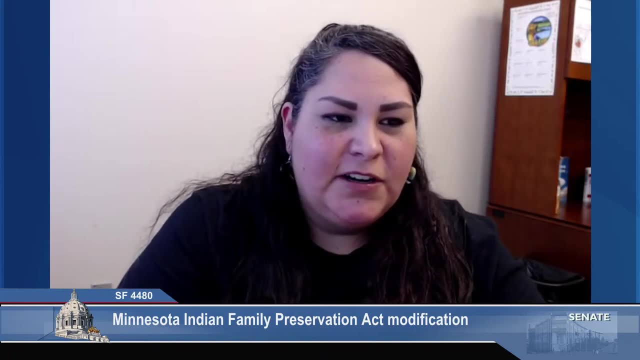 of Indian children, And it allows courts to award costs and sanctions where appropriate, when the court has invalidated proceedings based on violations of the law. So, as you've heard earlier today and if you recall from last legislative session, there was a number of folks that came together. 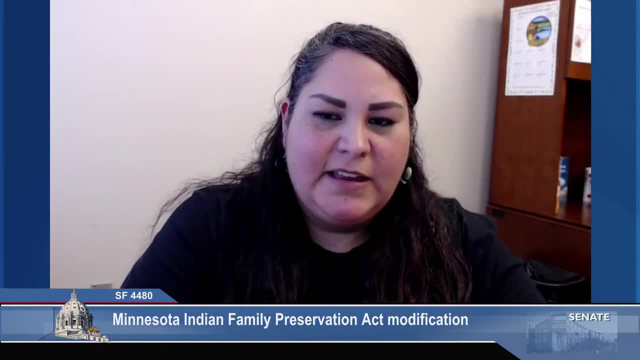 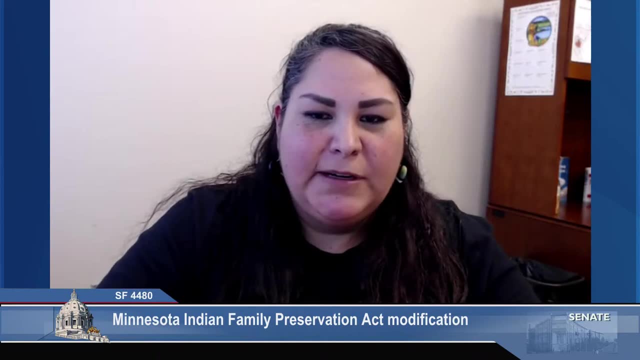 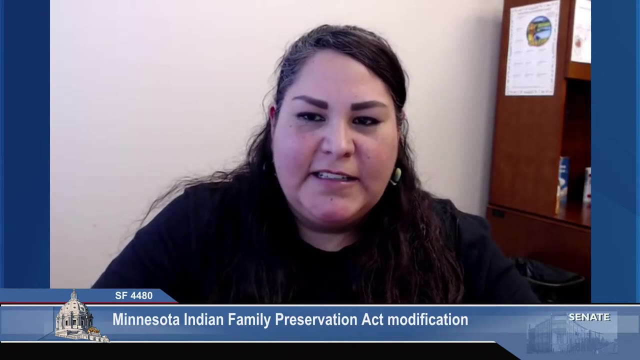 and this was known as the Tribal MFPA Work Group. Just wanted to thank all of those folks that had put their time and effort in moving forward with the language on this MFPA bill and proposal this year. There's still many practice improvements that are necessary. 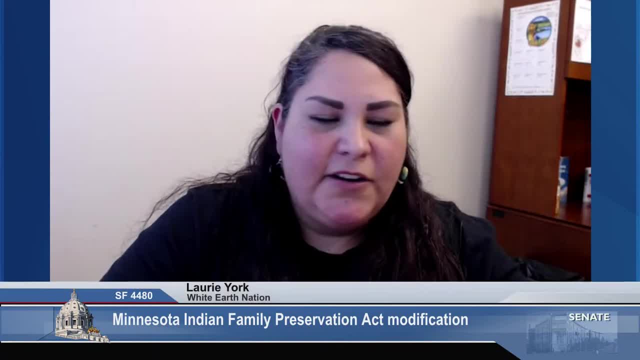 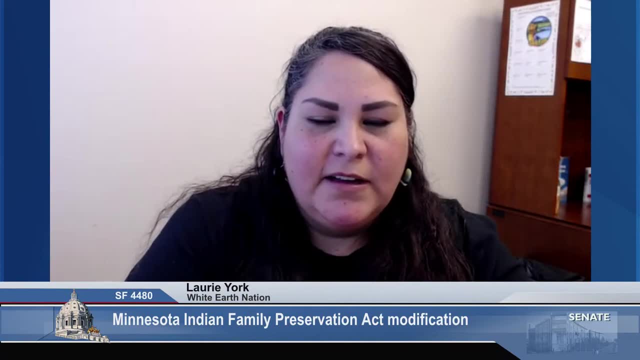 and the work will be ongoing now and into the future. as Judge McConkey-Green has indicated, There were letters of supports and or resolutions that were submitted from the Minnesota Indian Affairs Council, American Indian Child Welfare Advisory Council, the Minnesota Chippewa Tribe. 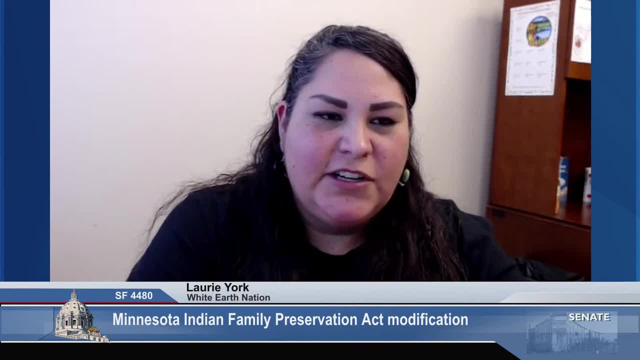 Fond du Lac, Upper Sioux, Leech Lake and White Earth Nation. In closing, we appreciate any consultation efforts extended by the Minnesota legislature with our tribal nations and thank you for working in partnership with tribes. We look forward to the continued discussion and we are requesting your support. 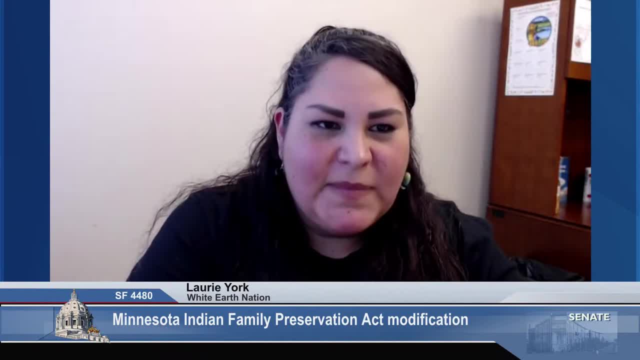 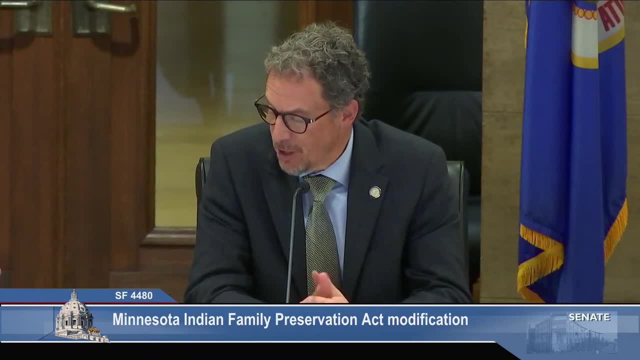 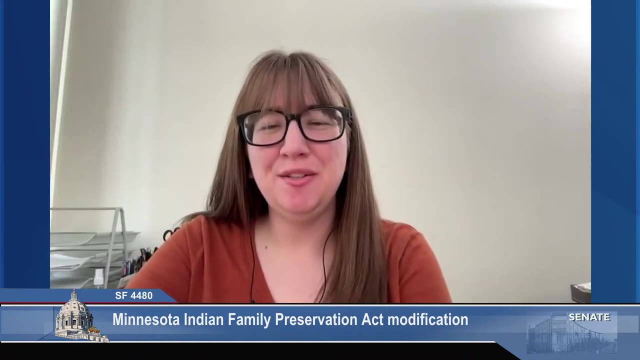 and approval of this bill proposed before you today, Thank you. Thank you, Director York, Appreciate your testimony. Our last testifier that has signed up is Sadie Hart from the Ainda Young, Our Home Center. Welcome, Thank you, Good afternoon. 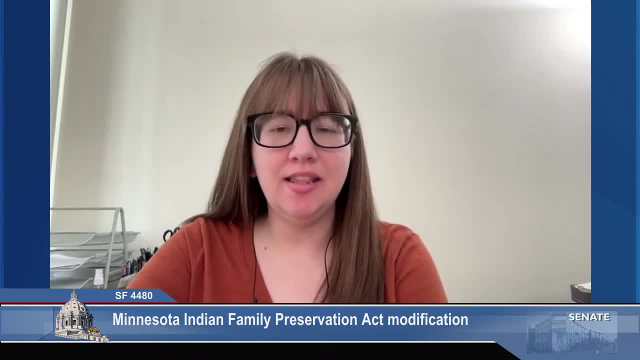 My name is Sadie Hart and I am the Indian Child Welfare Compliance Monitor at the Ainda Young Center in St Paul. Ainda Young means our home in Ojibwe and we provide a healing place within the community for American Indian youth and families. 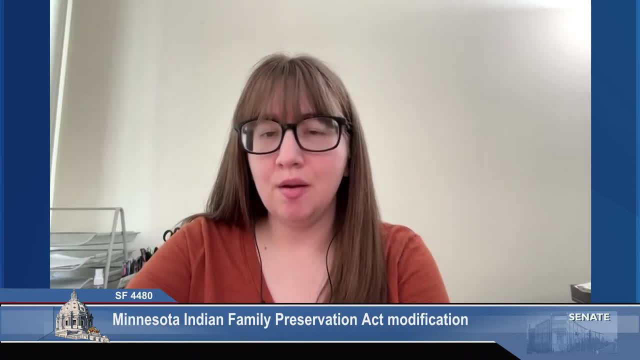 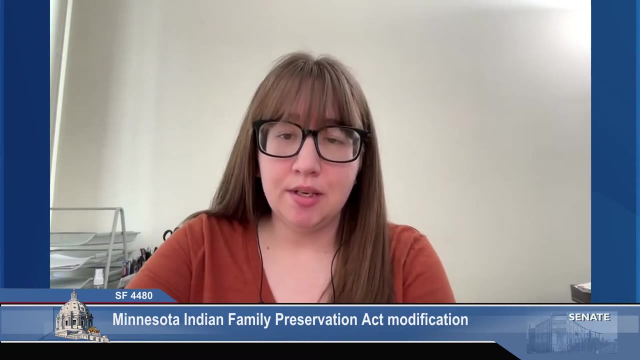 to thrive in safety and wholeness. I also chair the Ramsey County ICWA Advisory Board, which advises the 2nd Judicial District in Ramsey County on issues relating to Indian child welfare, and co-chair the Metropolitan Urban Indian Director's Family Preservation Committee In my role as the ICWA Compliance Monitor. 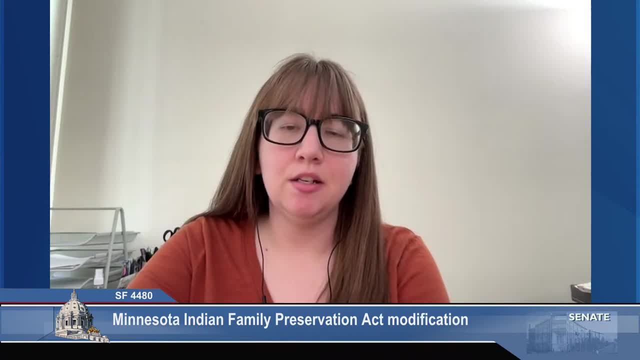 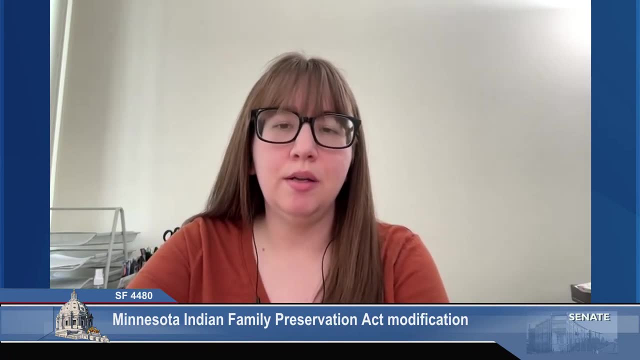 I work with judges, attorneys and other justice partners to make sure ICWA and MFPA are complied with and implement best practices, specifically in Ramsey, Anoka, Dakota, Washington, Carver and Scott Counties. I want to bring your attention to two issues. 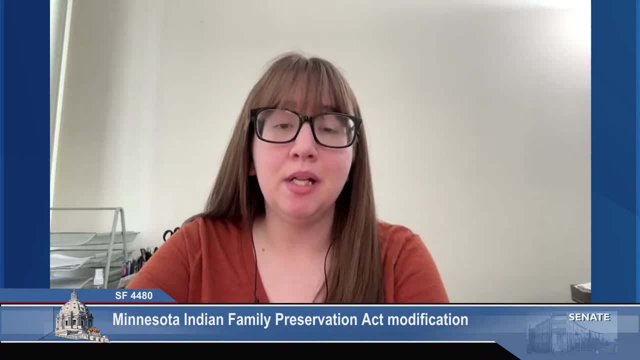 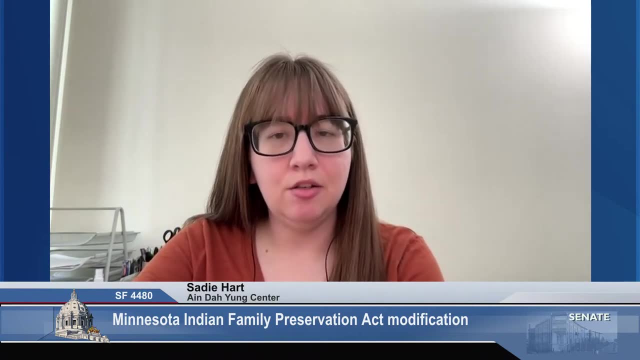 that I commonly see that this MFPA bill would address. The first issue is clarifying the court's responsibility to ask about a child's tribal heritage or ancestry, which needs to happen at the start of the proceeding and continue throughout the family's court involvement. 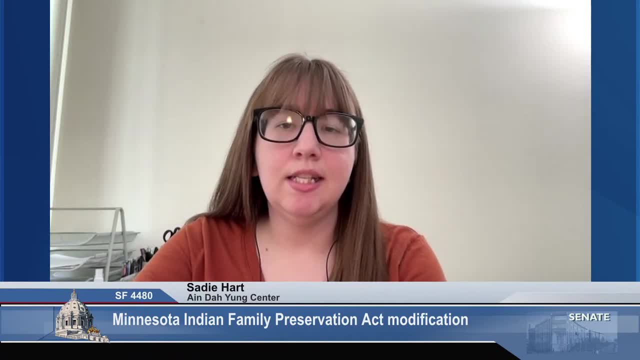 Identifying Indian children early in the process ensures that they receive the full protections of MFPA from the beginning, including active efforts to reunify the family and tribal involvement. Failing to identify Indian children can also delay the court process by needing to redo certain processes. 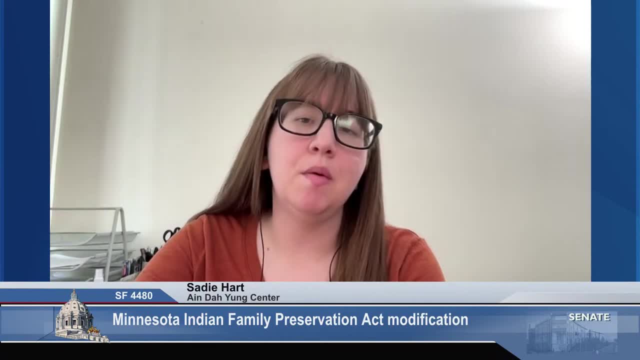 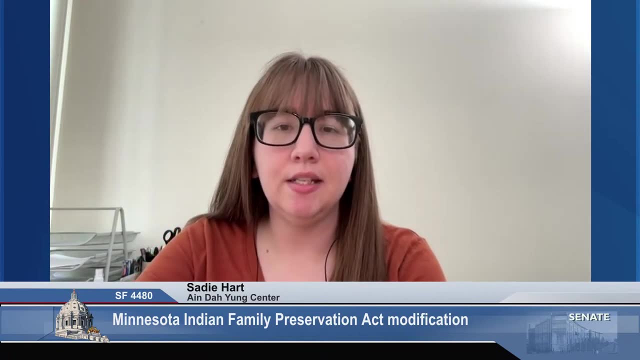 or invalidating the case. This inquiry is also required throughout the life of the case. so as new people, such as relatives, come to court, there's a clear obligation to ask about the child's potential tribal ancestry, to make sure Indian children are properly identified. 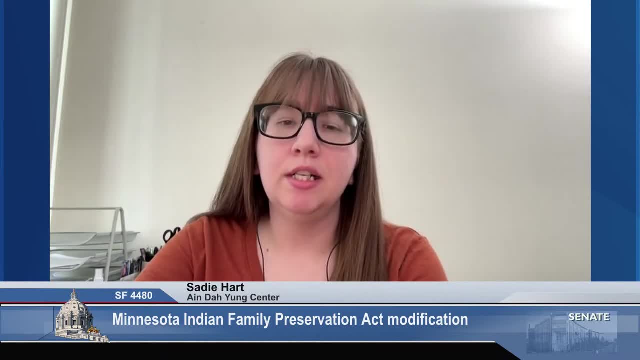 We frequently see these requirements being overlooked, so children don't get all of MFPA's projections and tribes aren't notified when their children are involved with the child protection system. The second issue is that we continue to see barriers that prevent tribal representatives from actively participating in the court process. 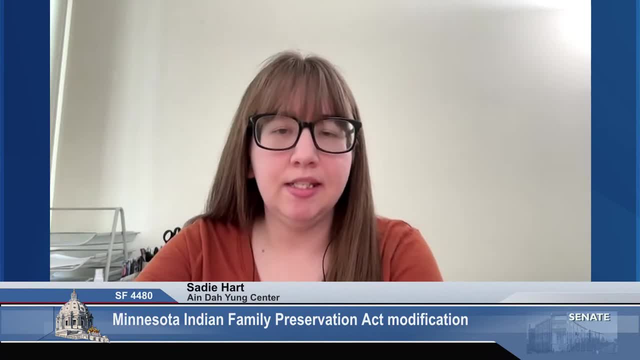 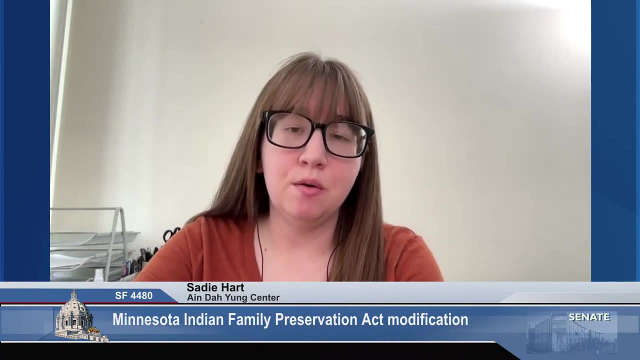 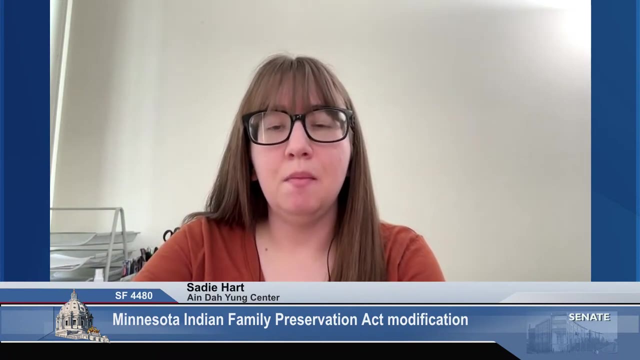 Tribes have party status in MFPA cases, but there is still a lack of understanding about the importance of their role, the valuable information they can provide the court and how they collaborate with other parties. This bill addresses that issue by creating a definition for tribal representative. 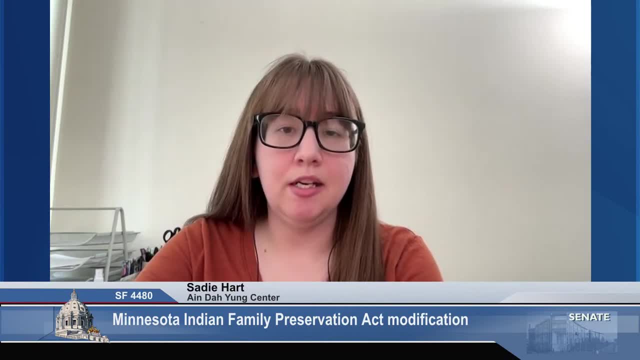 and clarifying that a tribal rep does not need to be an attorney. Many tribal reps are social workers and are at times not allowed to speak in hearings because they don't have legal representation. This bill also allows for tribal reps to participate in court hearings remotely. 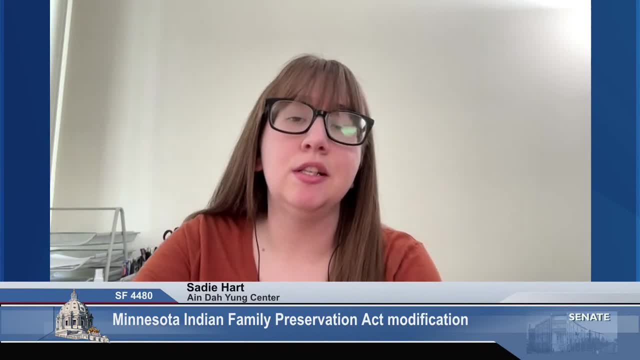 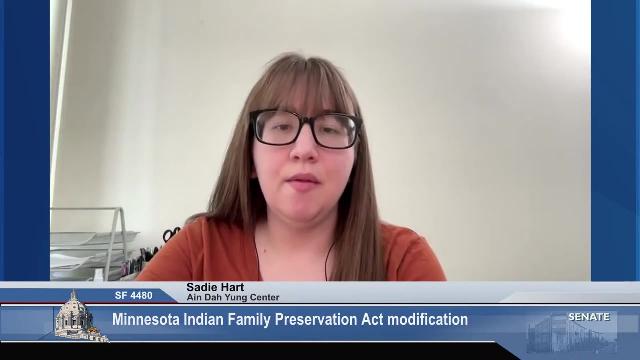 without prior request. Tribes have limited resources available to participate in cases and often have cases throughout the state and country. Making it easier for tribes to participate remotely means they can be more actively involved in the court process. These are just a few examples of how this bill 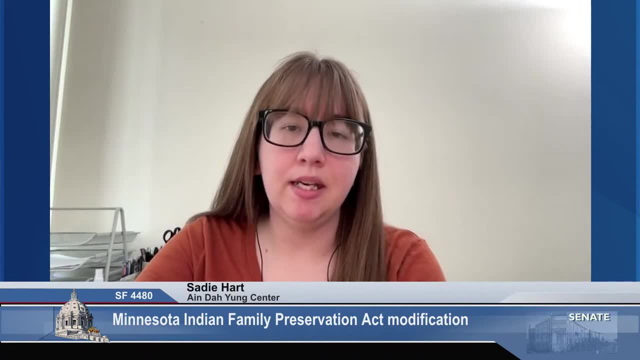 would improve the experiences for an Indian child and their family in the child protection system and ensure that tribes are fully involved in the court process. Thank you for your time and for considering this bill. Thank you, Ms Hart. Is there anyone else in the room? 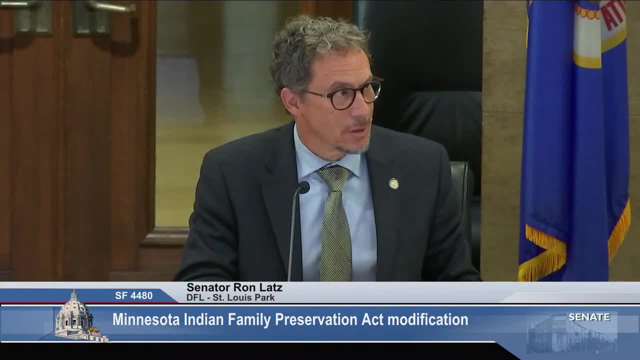 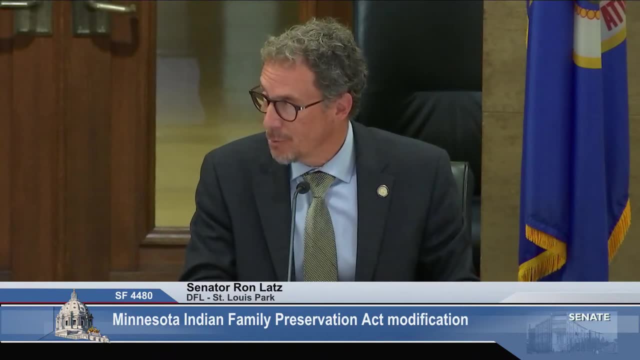 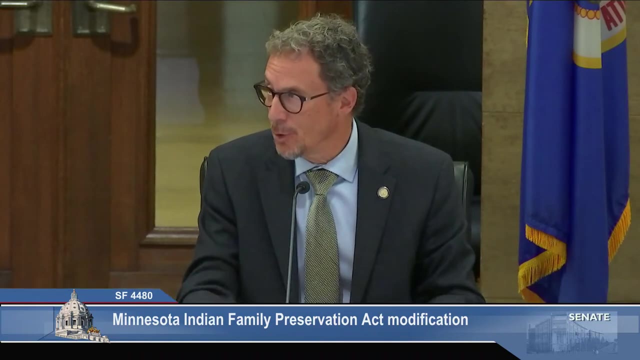 wish to testify in connection with this bill? All right, we will consider the A3 amendment. Senator Carlson moves adoption of the A3 amendment. Any discussion on that. All those in favor say aye, Aye. Opposed Motion prevails. 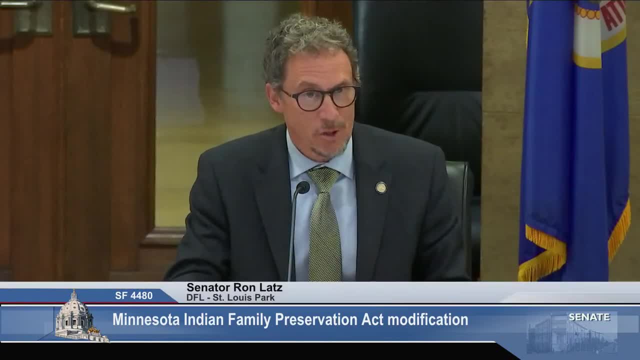 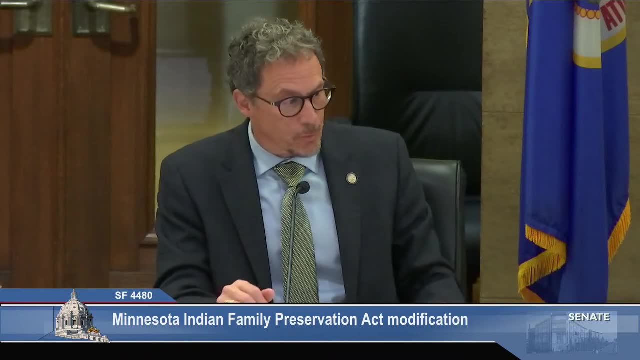 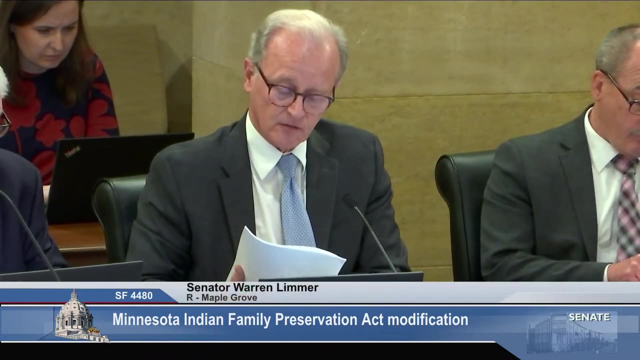 The amendment's adopted. All right members. any further discussion or questions about this bill, Senator Loomer? Thank you, Mr Chair. Senator Kroonish, I was looking over this packet. It was in our papers, entitled Resolution 54-24.. 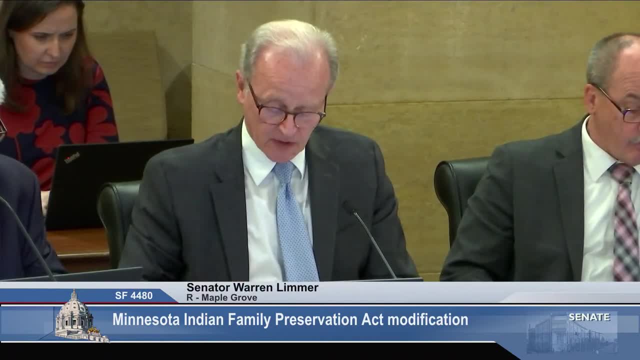 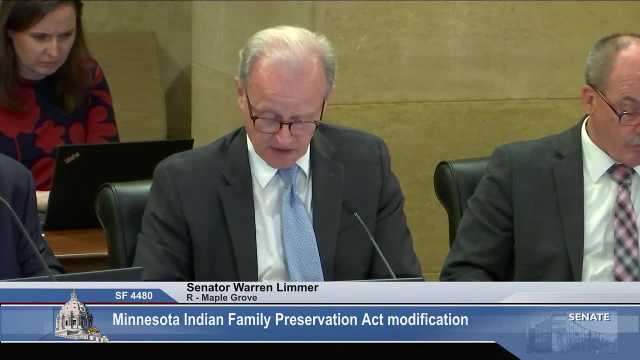 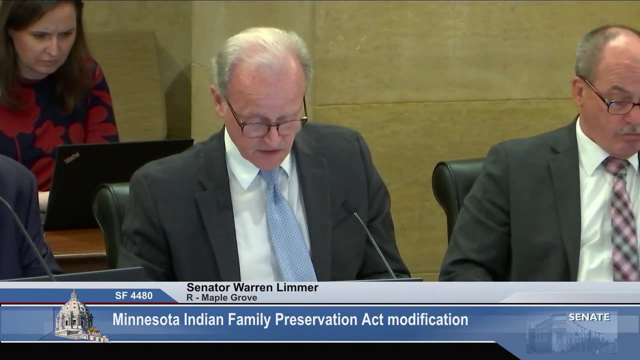 It's a resolution from the Chippewa Tribal Executive Committee That represents six tribal communities, I believe. As some may know, there's 11 tribal communities in the state of Minnesota. I flipped through this and I see there's a few Sioux tribes. 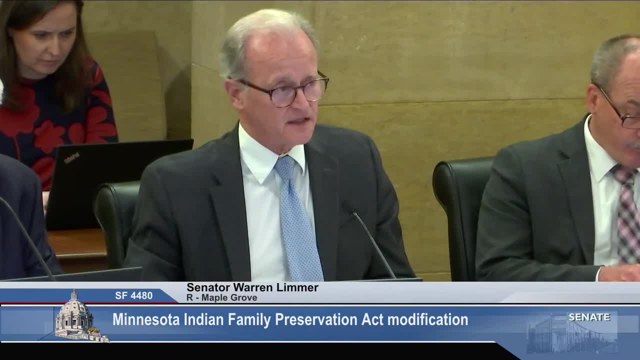 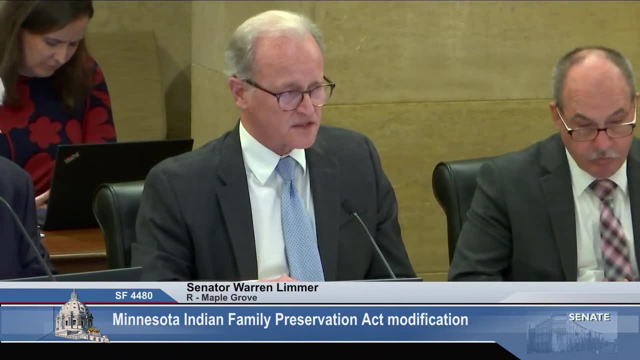 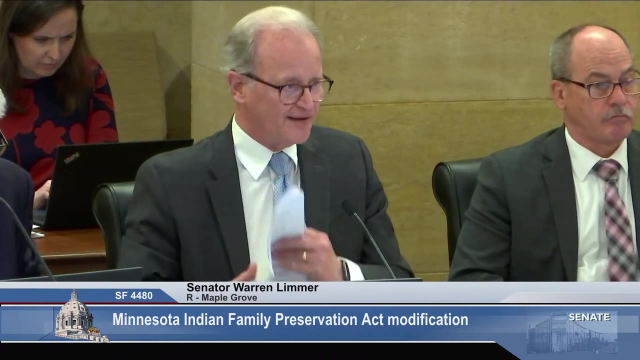 communities. I don't see any tribal communities in this packet, but are all of the tribes in support of this legislation, Because I couldn't find some of the tribal communities that I know are out there but not represented in this packet of paper? Senator Kroonish. 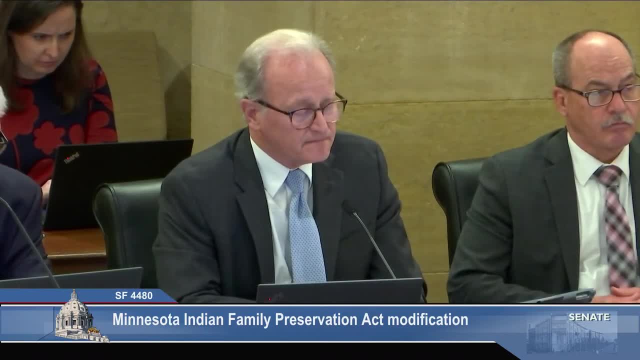 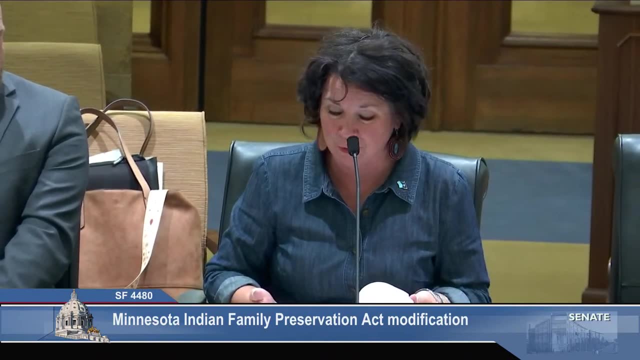 Thank you, Senator Loomer and Mr Chair. Yes, they are all in 100% support of this. They might have not gotten a letter of support in but a whole chunk nation who are not federally recognized. Minnesota tribe are part of this. 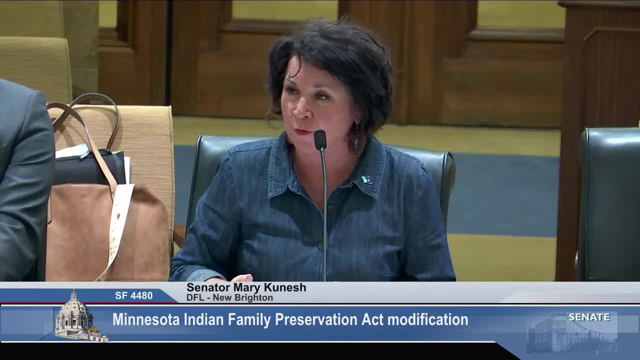 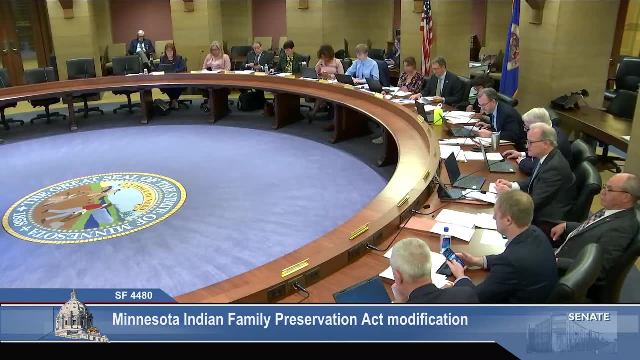 But yes, we do not have a single tribe that is not in full support of that and I'm not sure if you have anything to state to that, Mr Ryan. I don't have anything to say to that, but I would also turn to Judge McConkie-Green. 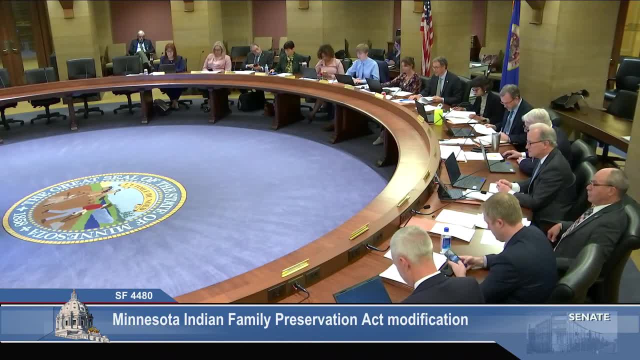 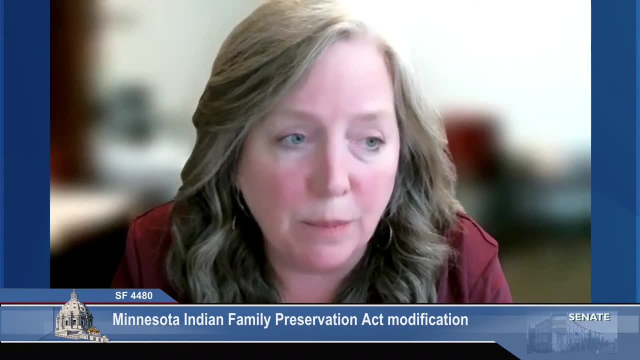 Judge McConkie-Green. Thank you, Mr Chairman. My understanding is that all the tribes in Minnesota are in support of it. For the most part. the tribes in Minnesota all participated very actively in the work groups and we came back several times, even throughout the amendment process. 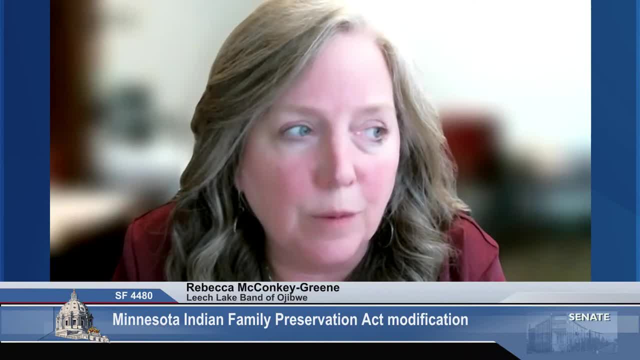 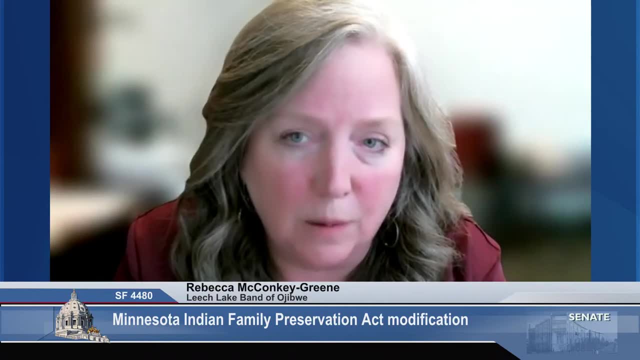 and checked in with everybody I have. one of the first tribes that provided a resolution in support was Upper Sioux, who wasn't able really to participate in the work groups themselves but did receive all the updates and when I had asked for resolutions in support. 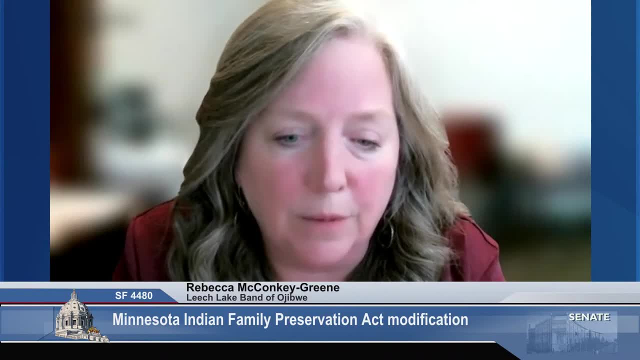 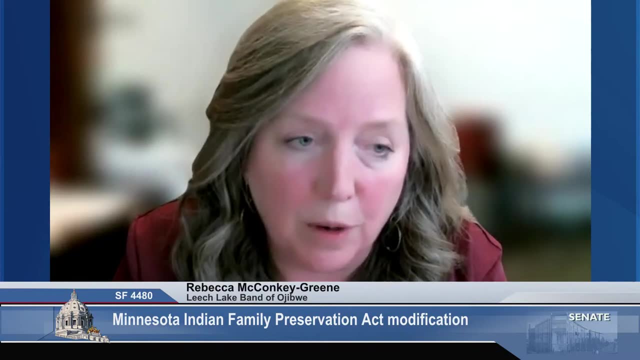 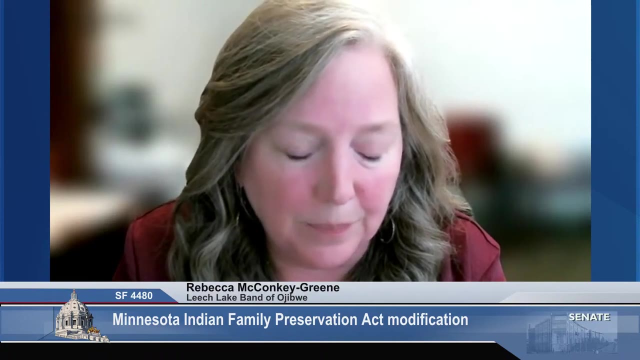 they provided one right away, And I'm also aware of support from Lower Sioux, who certainly has supported very heavily, as have Prairie Island and Shakopee-Midwakanton. I would also point out that I did take the bill to the MIAC. 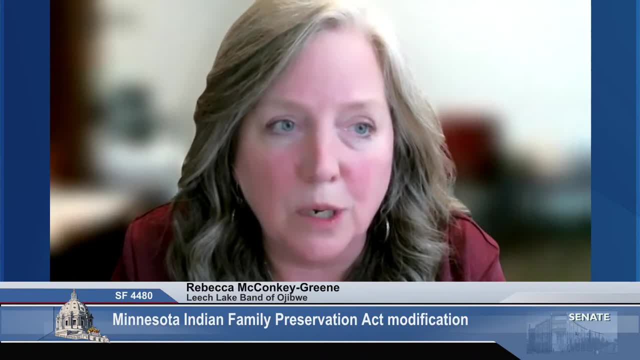 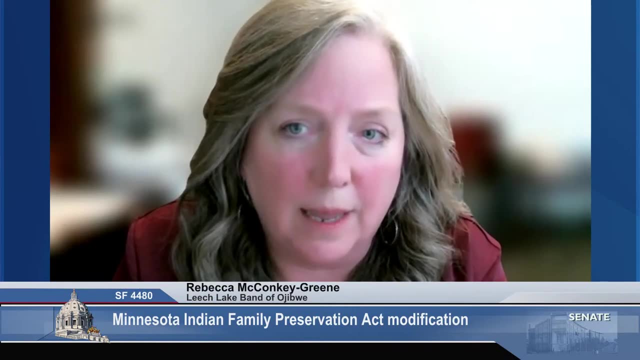 the Minnesota Indian Affairs Council and I believe with the exception of Upper Sioux, all of the tribes in Minnesota participate in that as well, and that was unanimously supported there at that group as well, And I think that's a good thing And I think there should be a resolution in the packet. 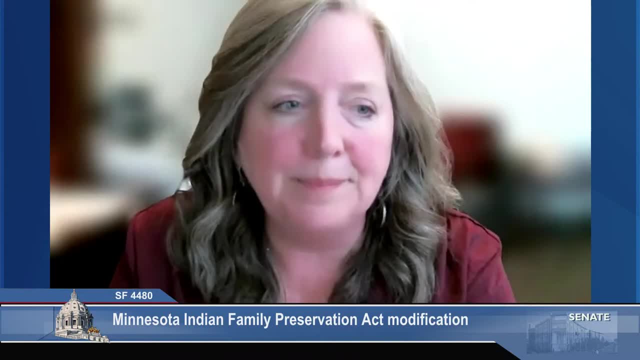 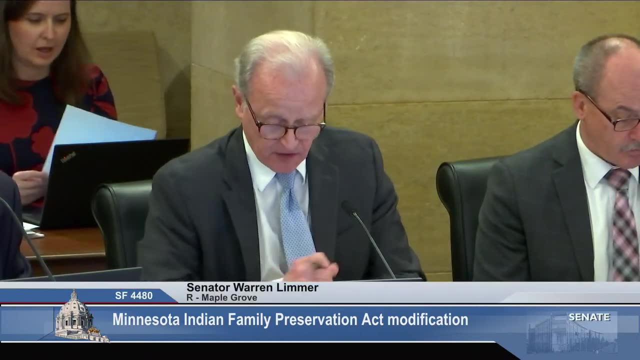 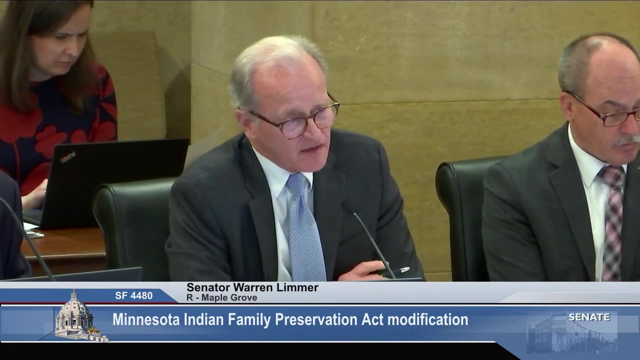 from them as well, Thank you. Thank you, Judge Chair, Senator Loomer. Thank you, Mr Chair. Having been here a while, I'm familiar with different requests over the years from tribal communities Sometimes, and the reason I raised the question earlier. 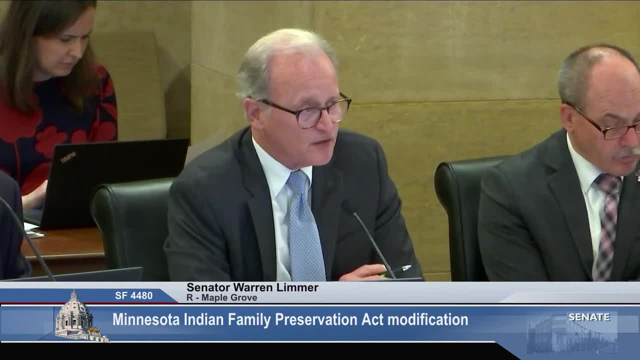 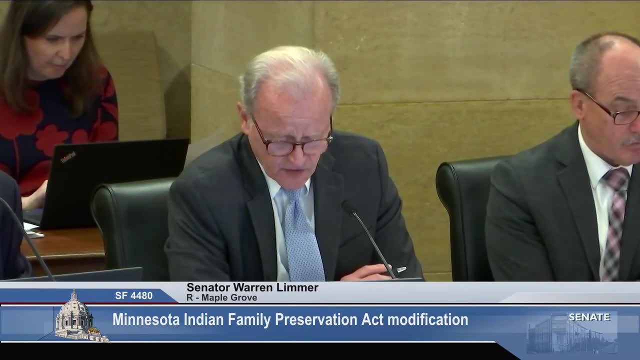 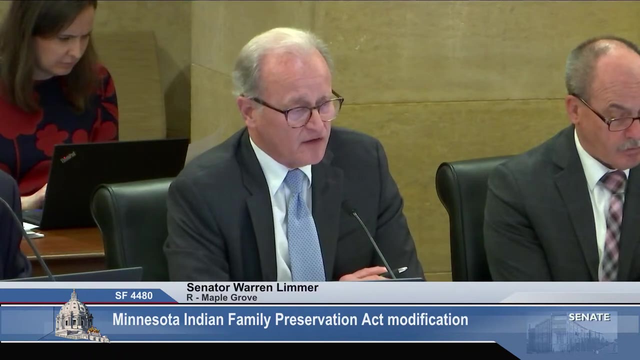 is that sometimes tribal communities don't always agree with one another, And so I think that's a good thing. I had to ask that question. However, I also know that different tribal communities have different amounts of resources. Some have a little more resource than others. 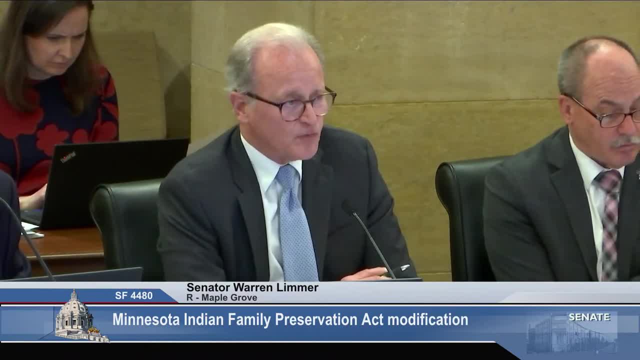 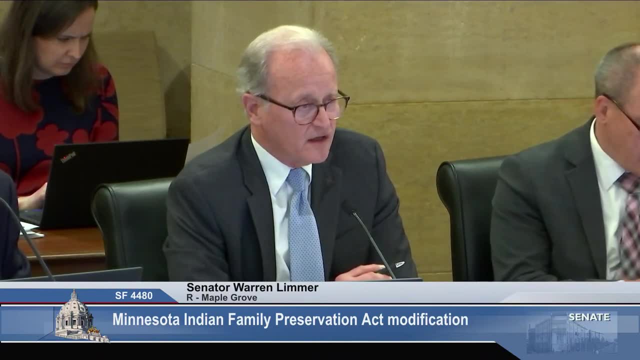 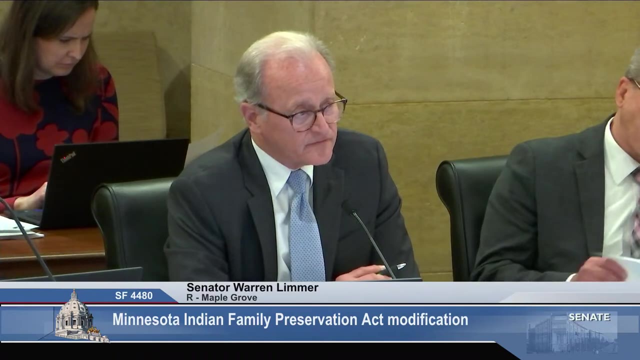 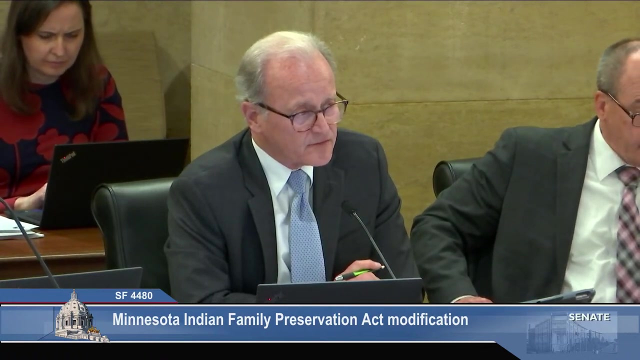 Does this trigger any inadequacies for supporting a child having been directed to a Native American community? Senator Koenig, Mr Chair, Senator Loomer: No, if anything, it actually bolsters their ability to look out for their children and for their families. 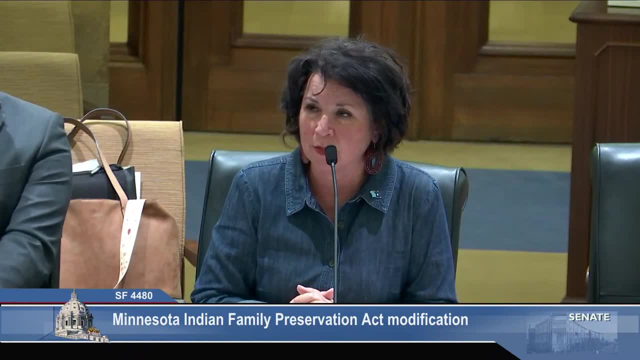 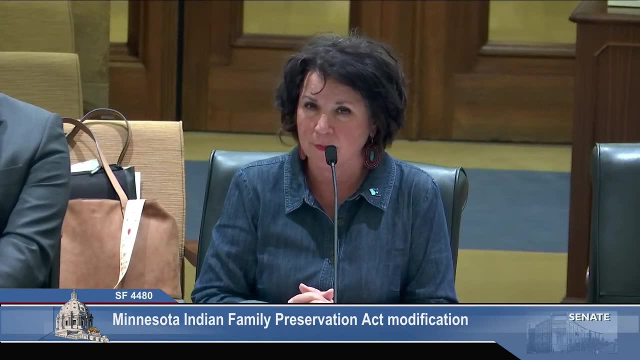 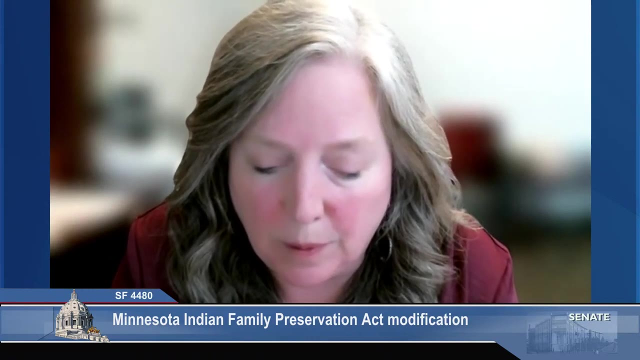 But again, perhaps Ms McConkie-Green would like to reply to that, as she's been so hands-on and the force behind a lot of this. Judge McConkie-Green, Thank you. So what I would tell you is that one of the people 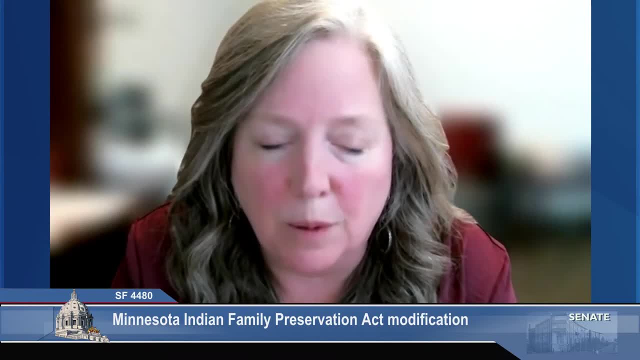 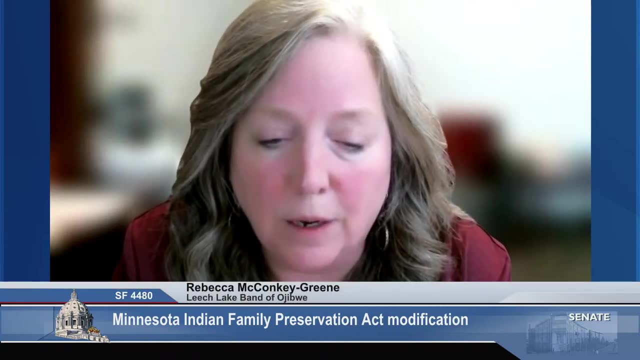 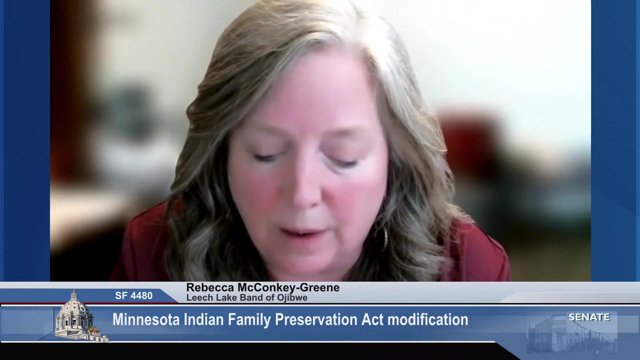 that was participating in the work group pointed out to us very early when we were forming committees that there is a problem that out-of-state tribes have sometimes with accessing their ability to participate in hearings and understand what is going on, And so there was a lot of that. 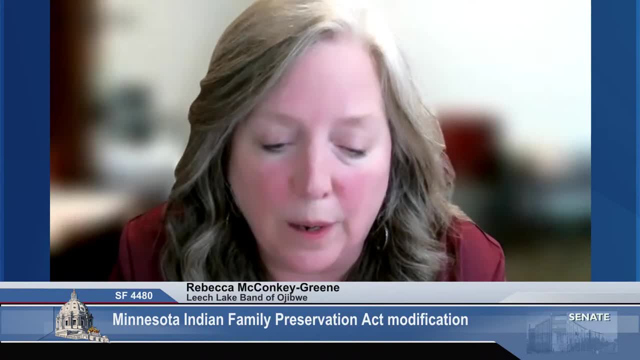 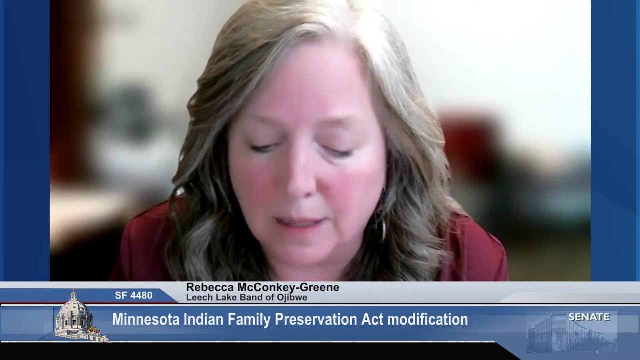 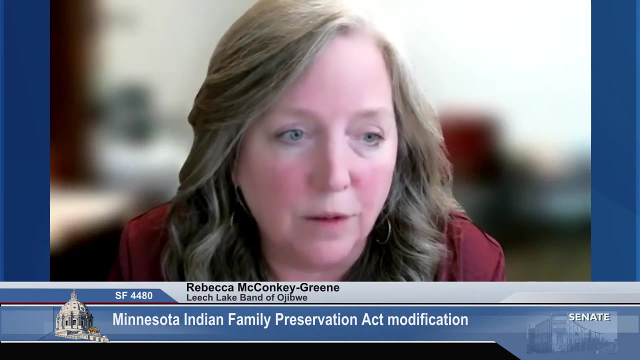 There was a work group that was formulated specifically to make sure that what we did supported access of all tribes, not only the tribes in Minnesota, but keeping in mind that, because of former policies of the US government, there are tribes that have citizens all around the United States. 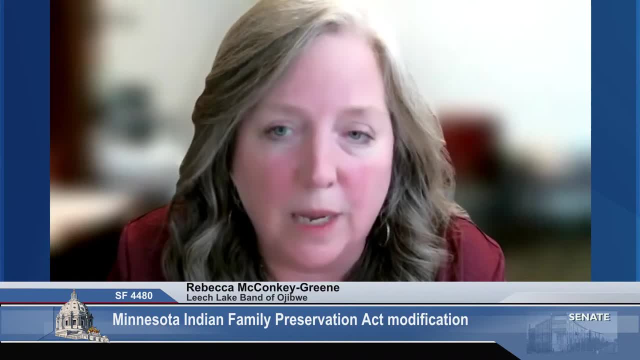 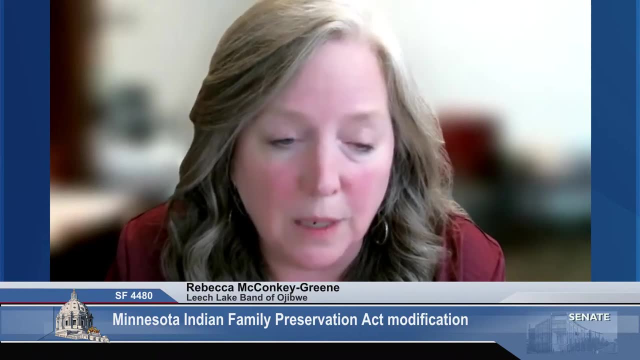 that need to be able to participate in hearings and advocate, And one of the things that we want to make sure that we're doing in Minnesota is making sure that tribes that are here in Minnesota, but also tribes that are not here in Minnesota, can attend the hearings. 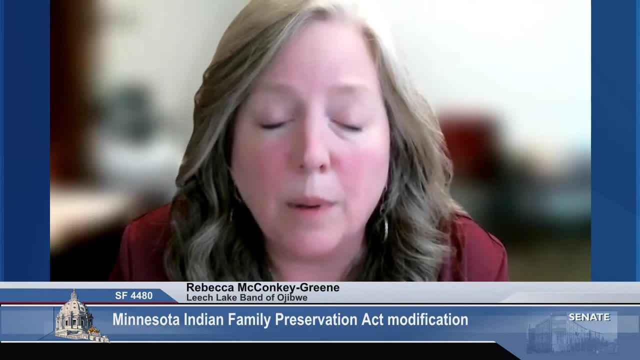 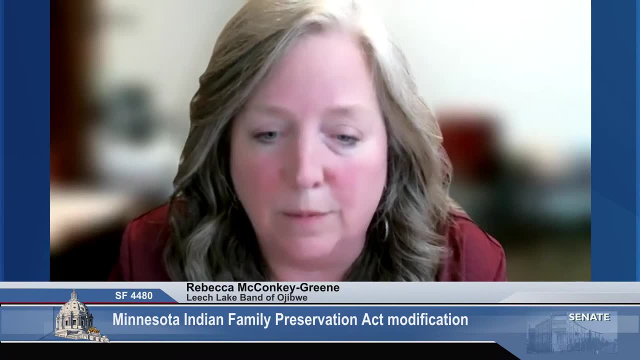 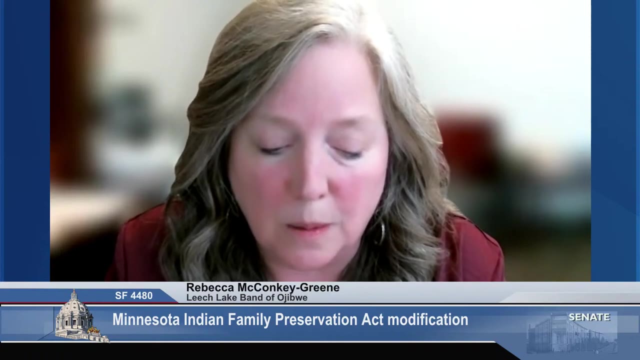 communicate with social workers, communicate with the other parties, but also being very heavily involved in proceedings that are not how we normally think of ICWA and MFPA or not the normal child protection hearings. So we wanted to make sure that those tribes could also participate. 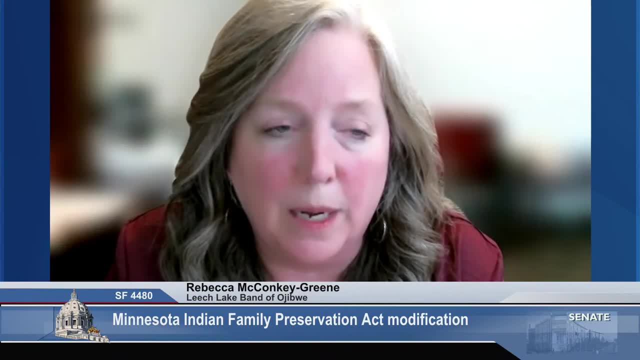 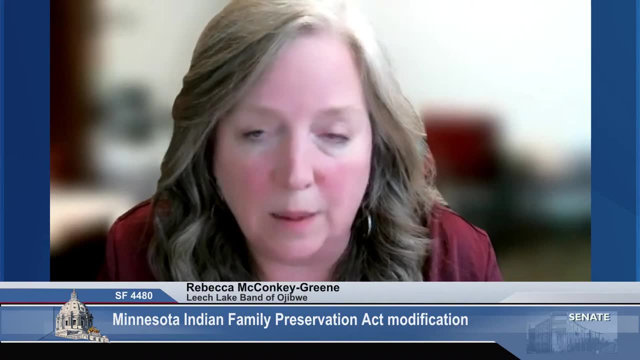 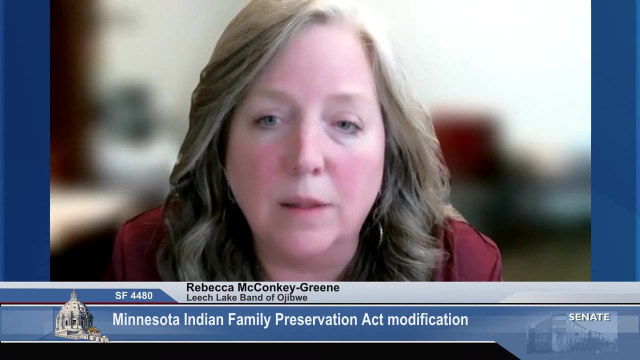 in family law hearings where ICWA and MFPA issues were coming up, and probate hearings and other types of cases. So some of the provisions that you see in the bill- for example, the appointment of counsel and the ability to appear electronically- those are the things, that those are the types of things. 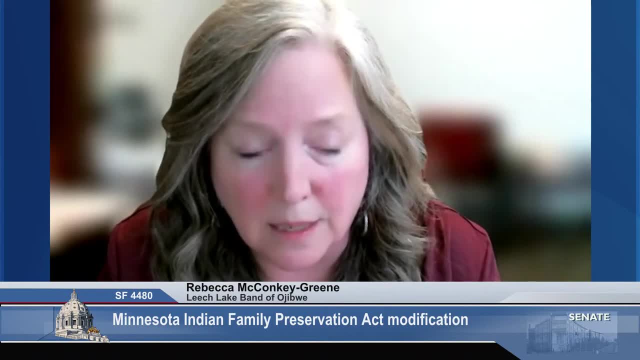 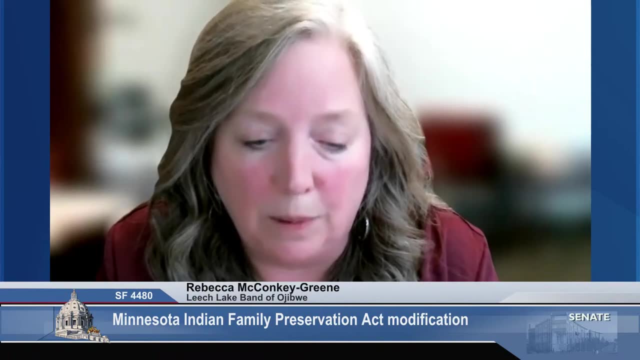 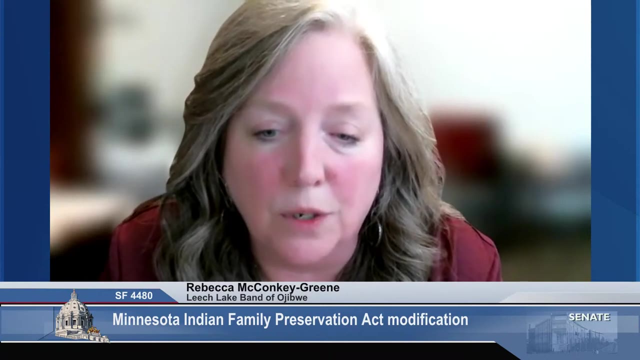 that already exist in Minnesota for child protection cases, but now we're making sure that there's language that is extending those protections to people that have ICWA and MFPA cases that are not traditional child protection cases. So, as Senator Kunish said, we're actually expanding a lot of protections. 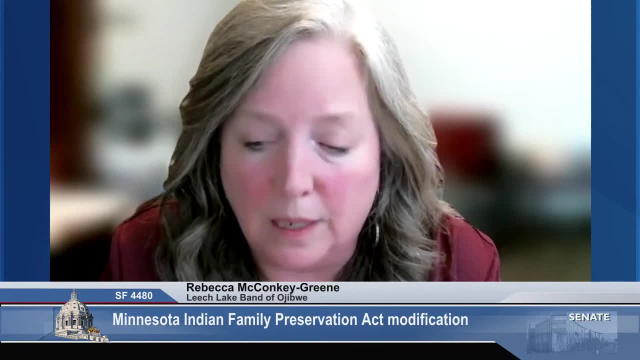 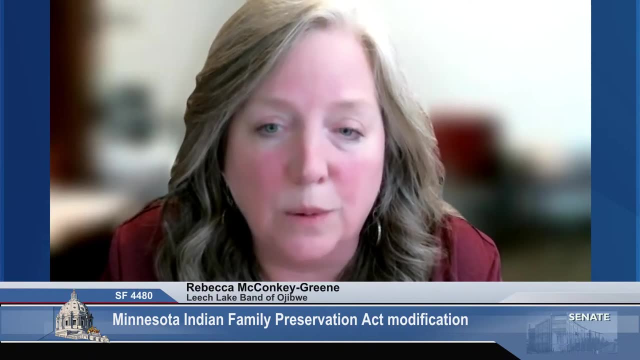 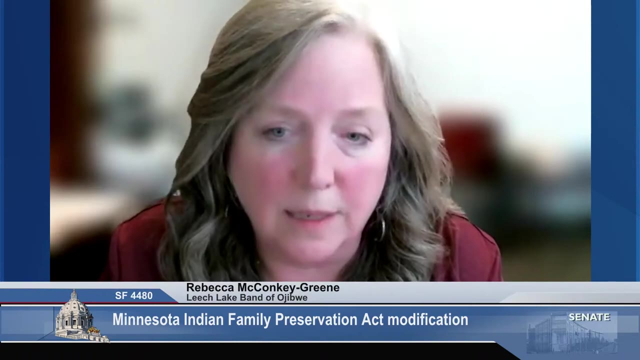 and making sure that people have a much greater ability to appear. It can be very expensive For tribes to have to fly people all over the country to appear in ICWA and MFPA hearings, and so hopefully this alleviates a lot of that pressure and cost for tribes. 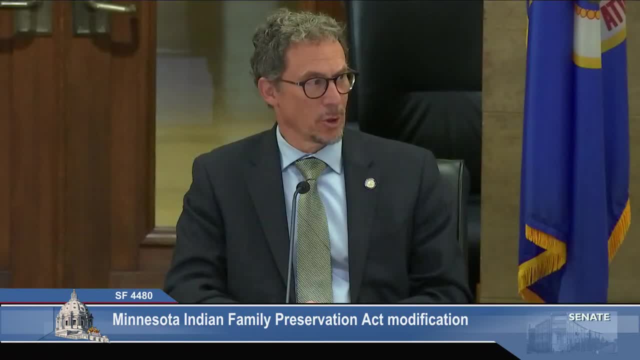 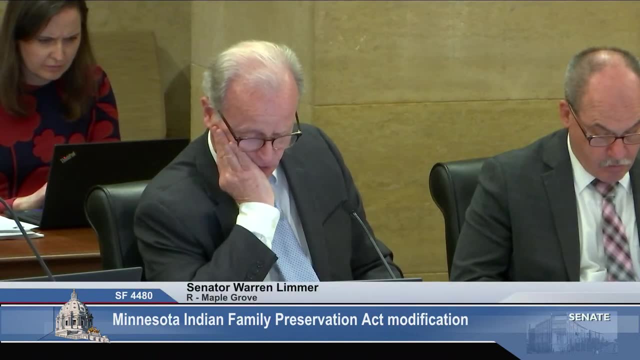 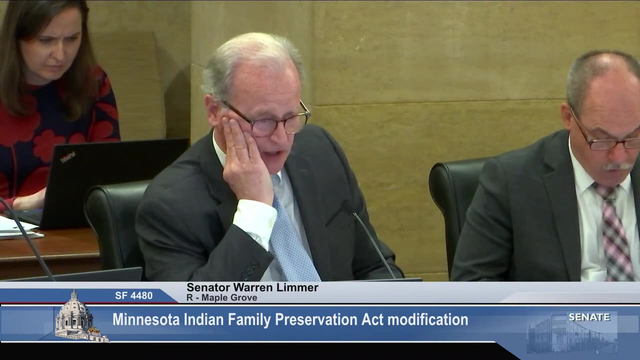 Thank you, Mr Chair. Senator Loomer. Mr Chair, thank you. I'm trying to recall when we've had discussions about this issue before and maybe, Judge, you could answer this question for me. Um, The child that may be subject to a child protection order. 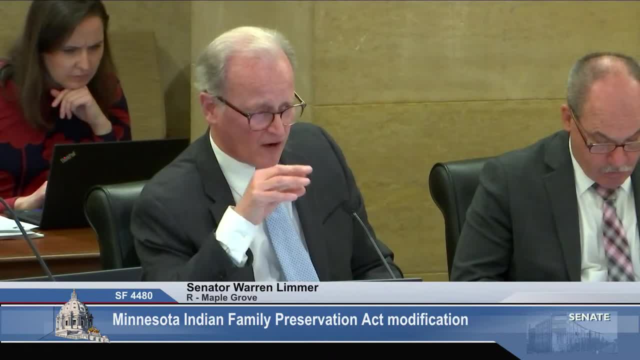 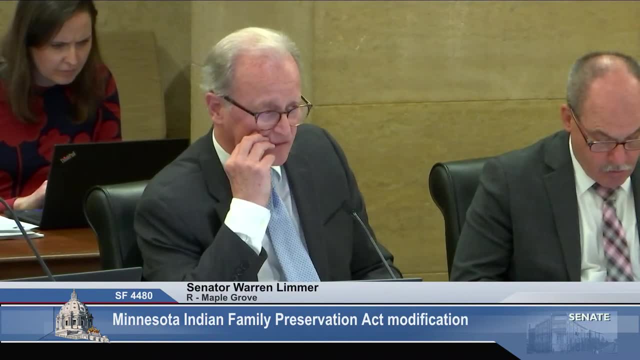 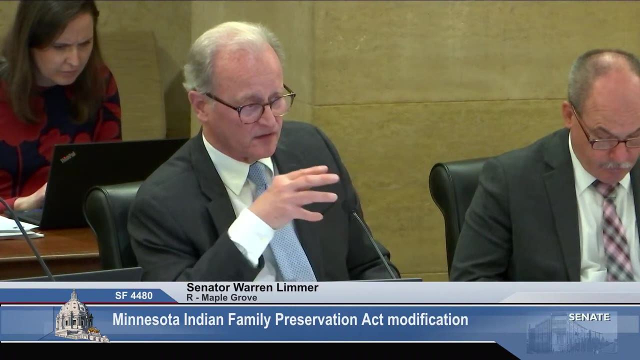 and not in a tribal community. where are they now? Are they in a foster home? Are they? could you just tell me the targeted child that we're and their settings, so we know where they are and where they want to be drawn from and to an Indian family? 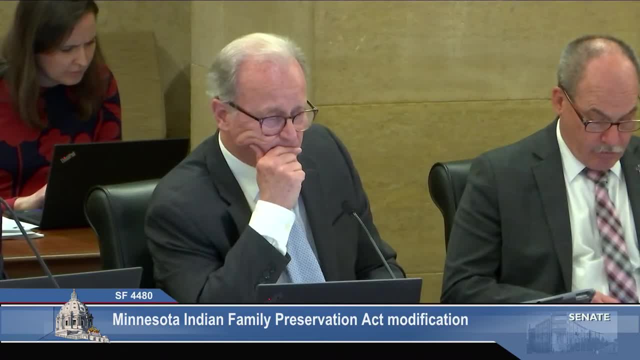 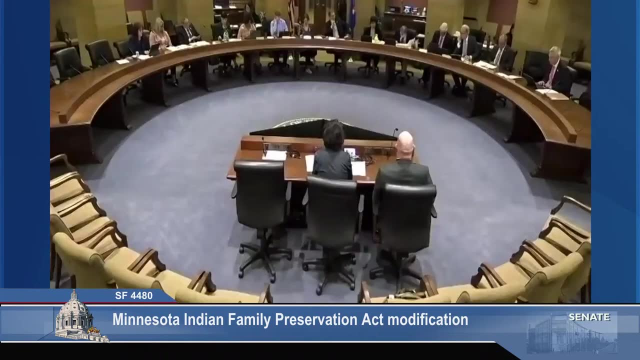 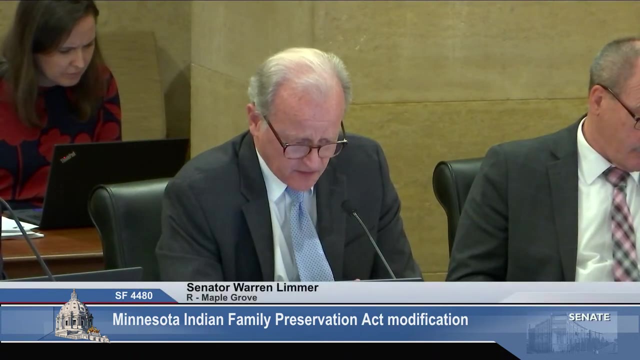 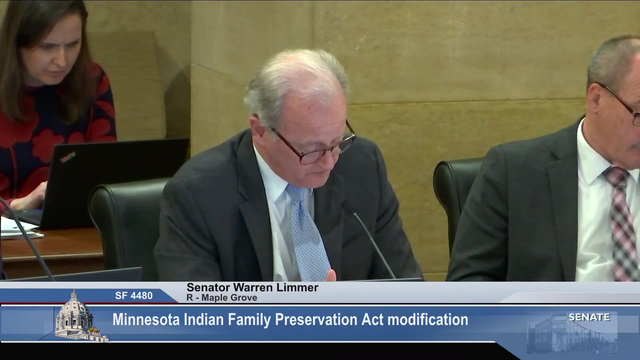 Okay, I just want to clarify, if I may, Mr Chair, to make sure that I understand the question. Senator Loomer, could you restate the question please? I'll try Judge where would be a typical child that would be a subject of seeking custody. 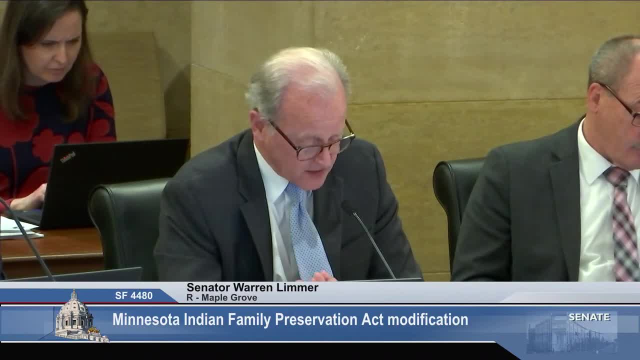 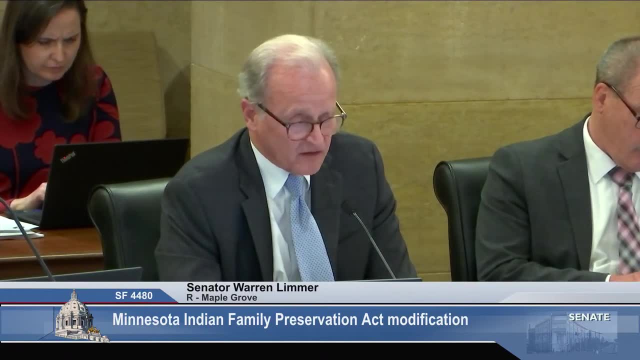 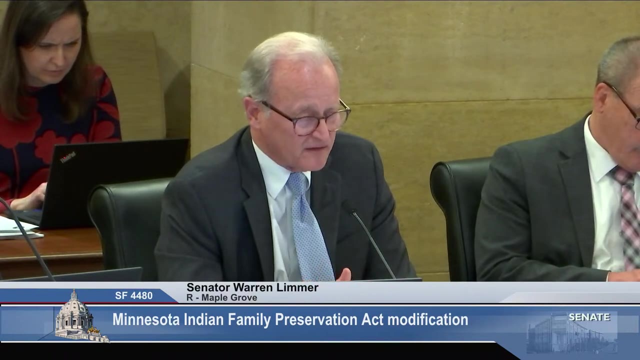 in an Indian would satisfy the Indian Family Preservation Act. Are they in a foster home? Are they in? do they have a criminal, minor criminal setting? Could you just tell me what and who they are in general, Judge McConkie. 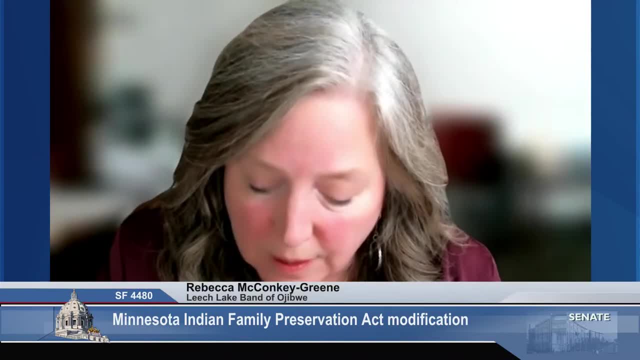 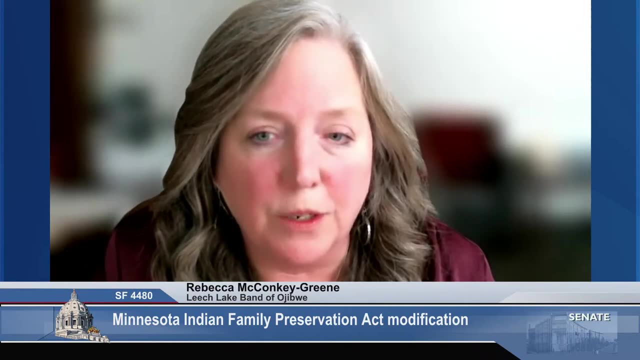 Thank you very much, Mr Chair, And thank you for the question, Senator. Yes, I'm happy to do that. So cases the Indian Child Welfare Act and the Minnesota Indian Family Preservation Act actually start protecting children, we hope long before they're actually placed out of home. 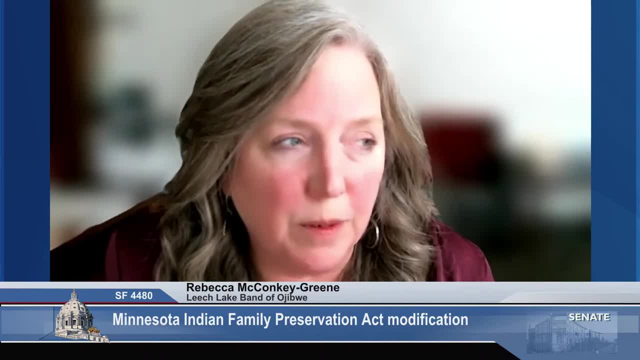 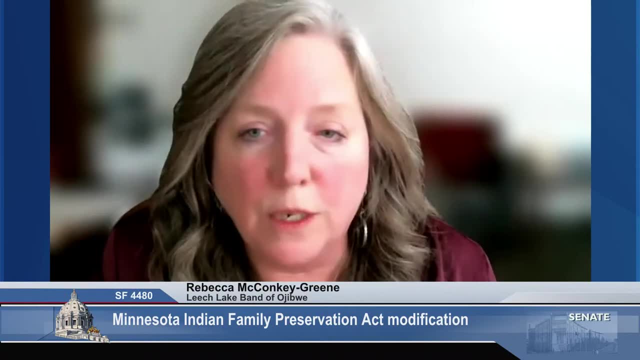 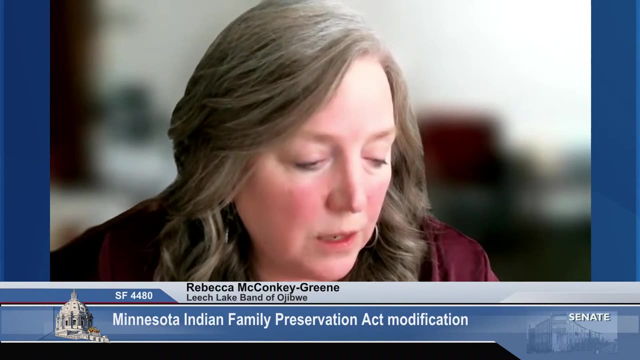 or even part of the court system. The Minnesota Indian Family Preservation Act back in 2015 was amended to require counties to reach out as soon as they were having contact with children- and I should say, instead of counties, petitioners- when they were having contact with Indian children. 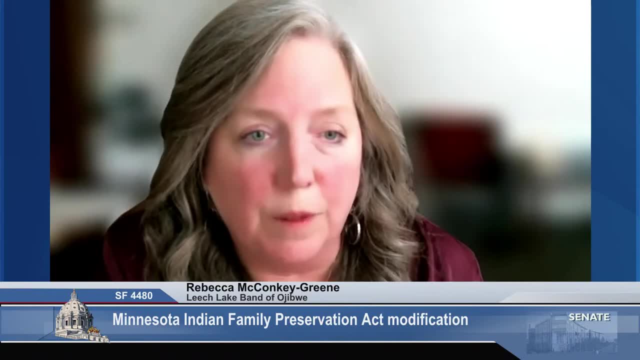 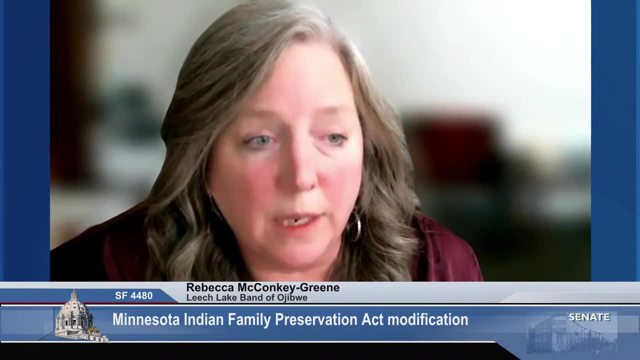 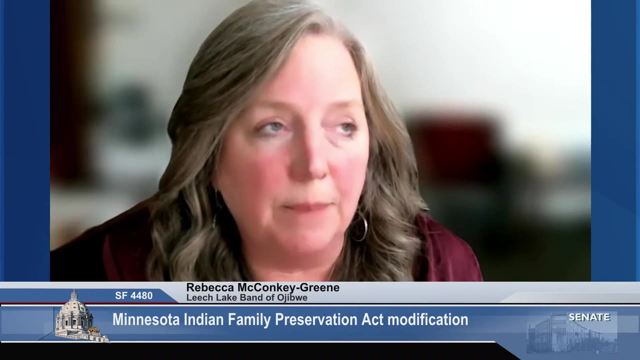 that may need to be removed from the care, custody and control of their parent or Indian custodian. The act in general applies to any such case where the child- where an Indian child- could be removed from their parent or Indian custodian, except for a couple of exceptions. 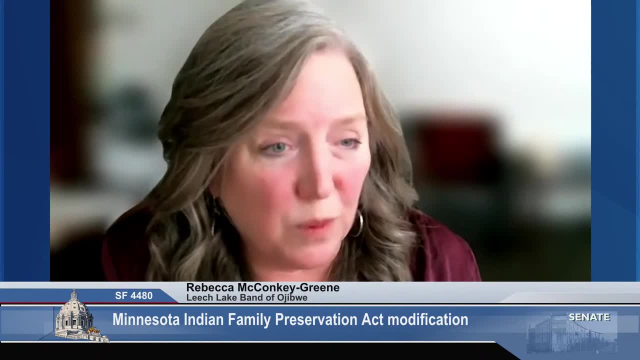 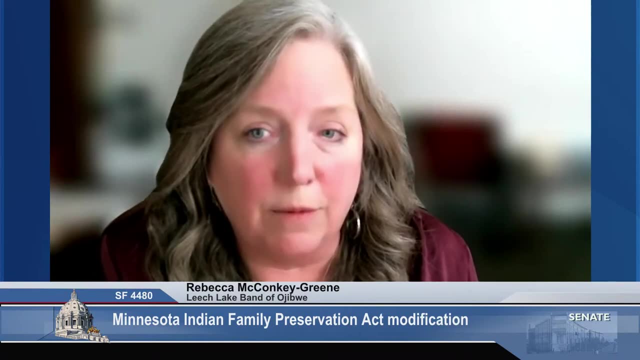 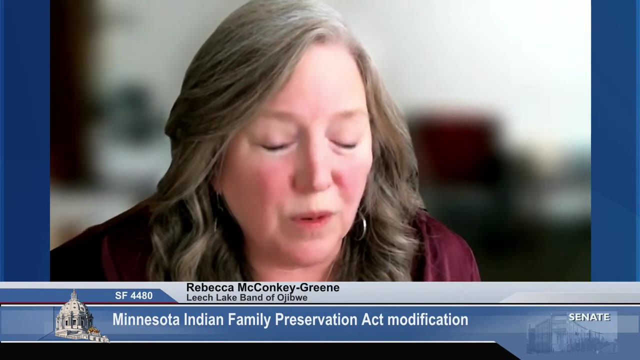 It does not apply, for example, when there's a custody action between parents, but it would apply if, for example, grandma felt that the child wasn't safe in the care of the child the child's parents and sought custody. It doesn't apply when there's juvenile proceedings. 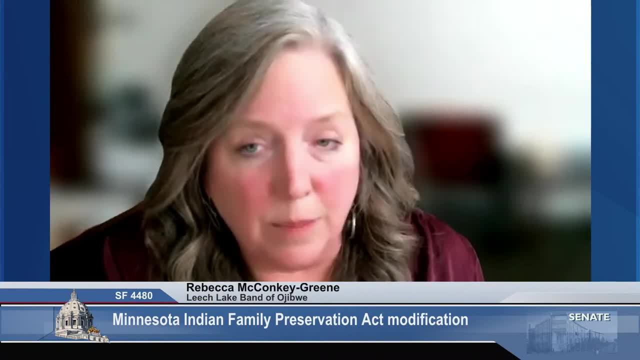 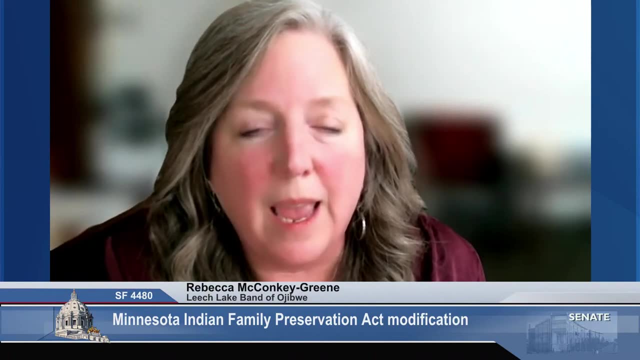 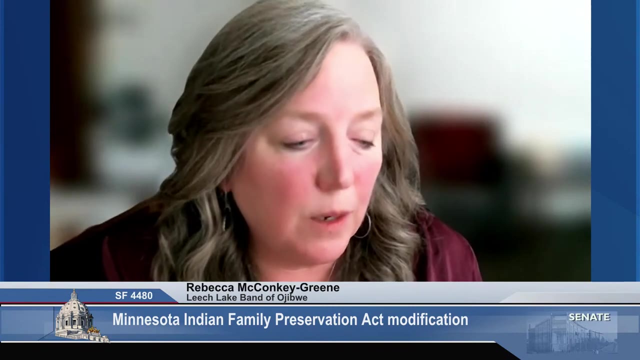 that are not status offenses, but it does apply in status offenses such as truancy and minor consumption types of things- although we don't usually see that in Minnesota And I feel like I'm missing one, But generally if there is somebody who is not a parent. 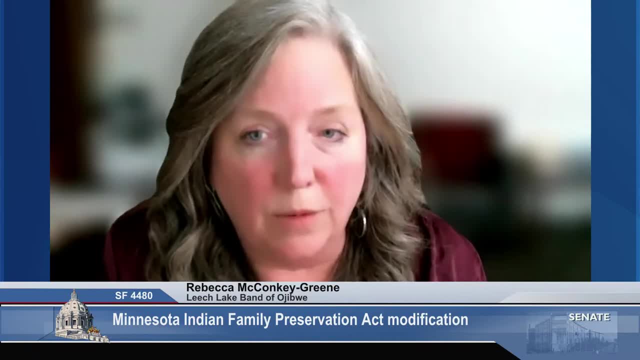 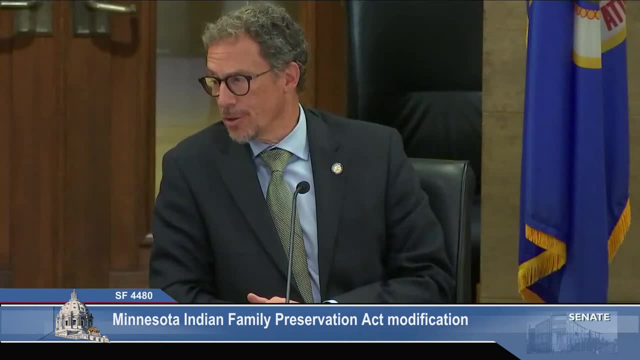 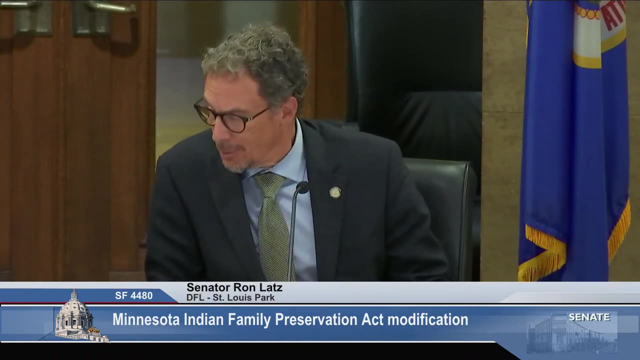 or an Indian custodian who is seeking to remove the child from the parents, then the act kicks in and applies. Thank you, Thanks. Any further questions or discussion on Senate File 4480?? I'm not seeing any Members. the appropriate move now. 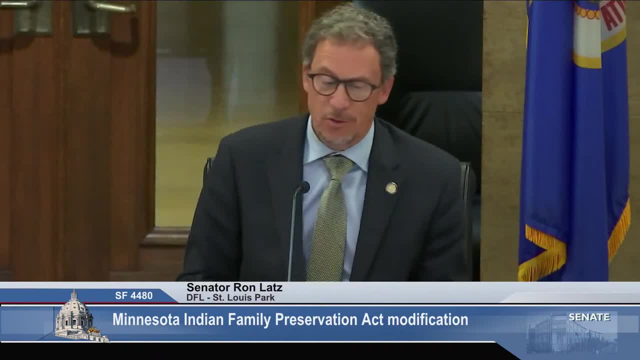 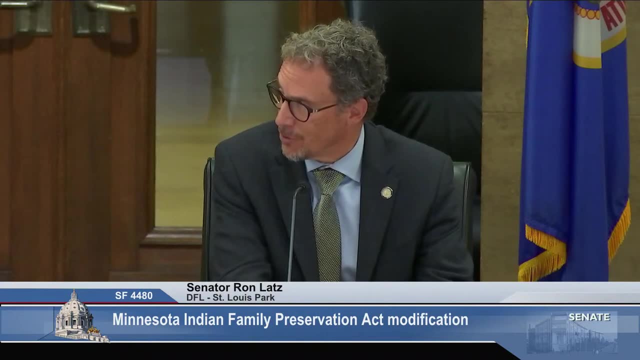 is to pass this bill on to the Finance Committee. since there is a fiscal note, It does not implicate our budget. So Senator Pappas moves that Senate File 4480, as amended, be recommended to pass and be re-referred to the Senate Committee on Finance. 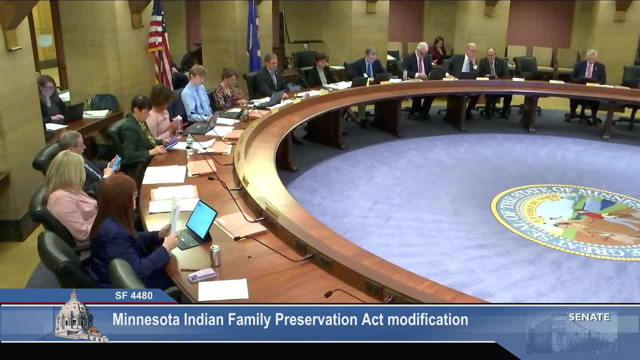 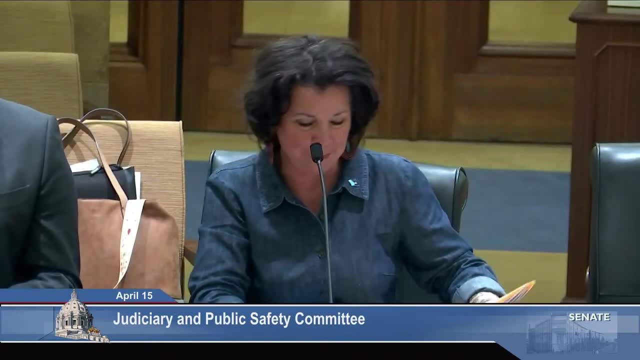 All those in favor say aye, Aye. Opposed Motion prevails. Thank you, Senator Kunish, Thank you Chair, and thank you all for meeting and getting this through for us. Appreciate it, Senator. Herr, we're going to fit you in here. 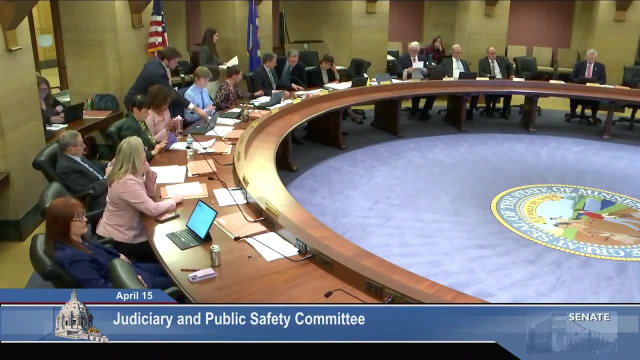 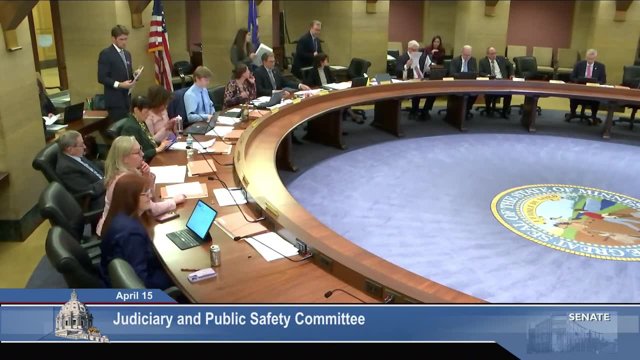 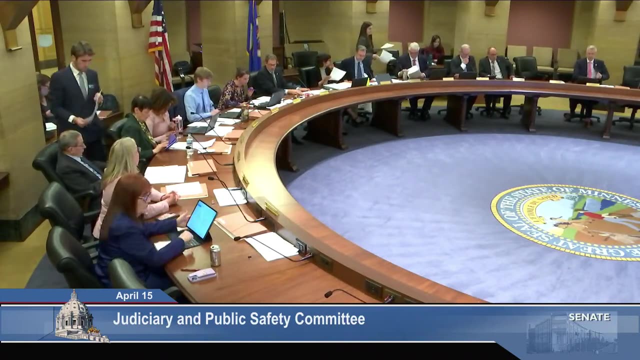 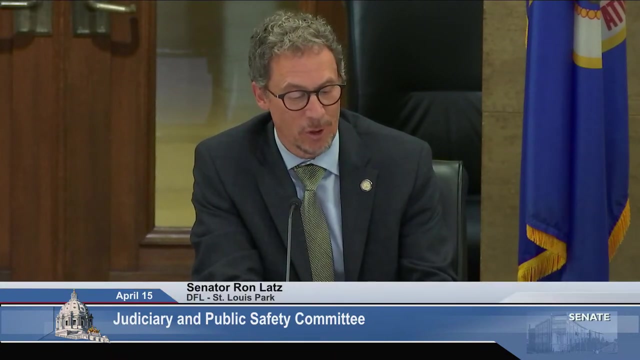 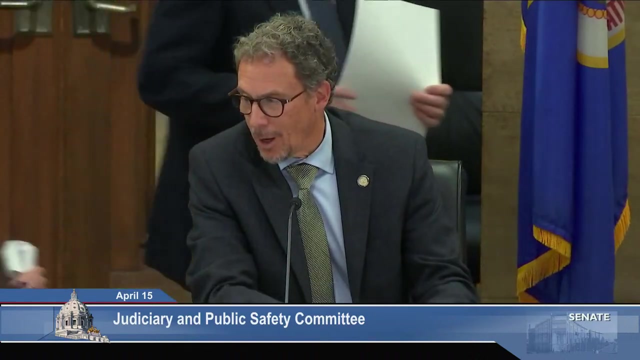 Thank you. So, members, we did send out an email indicating that Senator Herr's bill was not going to be heard because of the lateness of the floor. sessions Adjournment. This is a? Oh, sorry, There is a fiscal note. 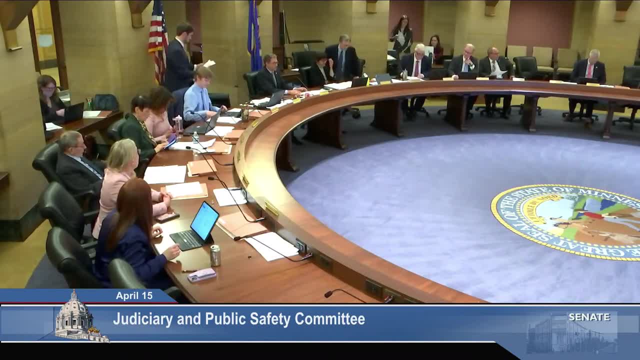 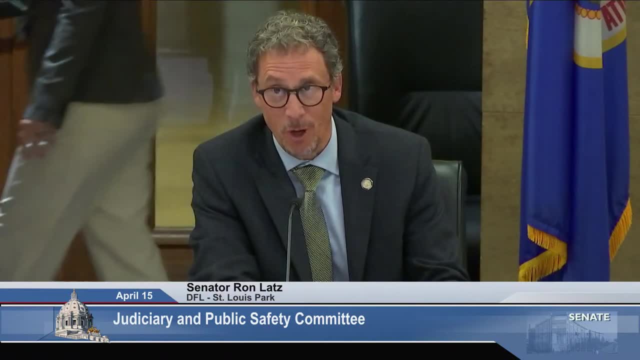 The idea is to give us some information as we decide what to do with regard to our limited resources. By the end of the week, we will have a budget bill out of this committee as well. So since Senator Herr brought some testifiers in, 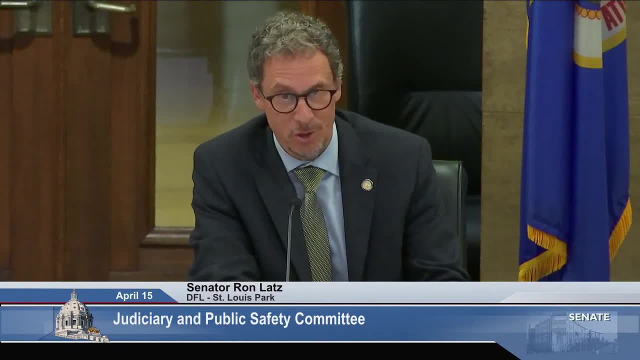 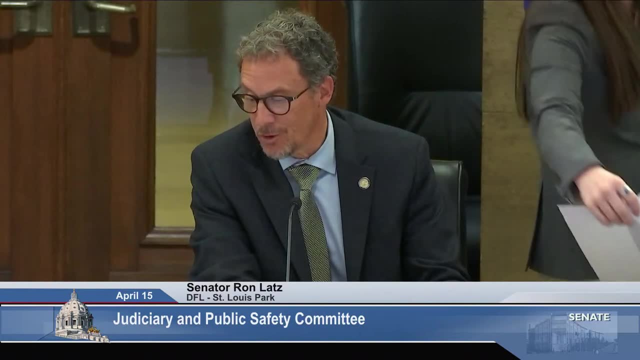 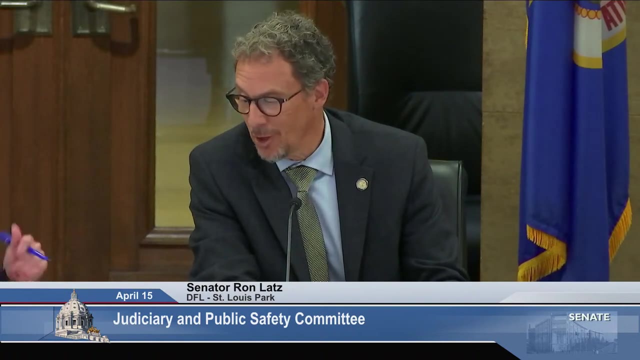 I'm going to take the prerogative of the Chair to have an informational hearing, And if there is anyone who wishes to share information with this committee that was not able to join us today because of the email that went out, then we of course welcome their input. 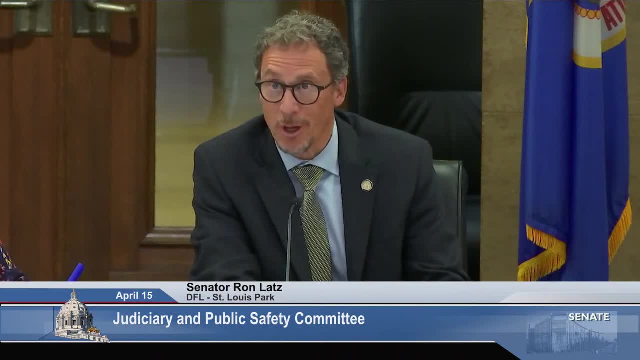 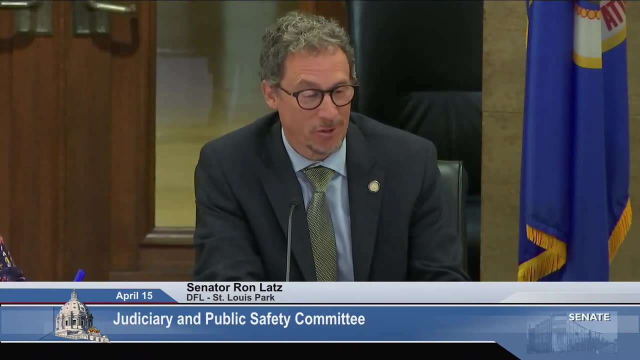 as we make our decisions. So, Senator Herr, we've got about 10 minutes. Okay, Mr Chair, I wanted to give an opportunity for your testifiers that you brought along here to share their information with the committee, Senator Loomer. 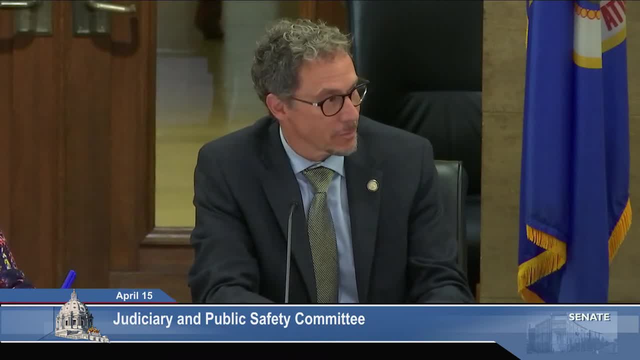 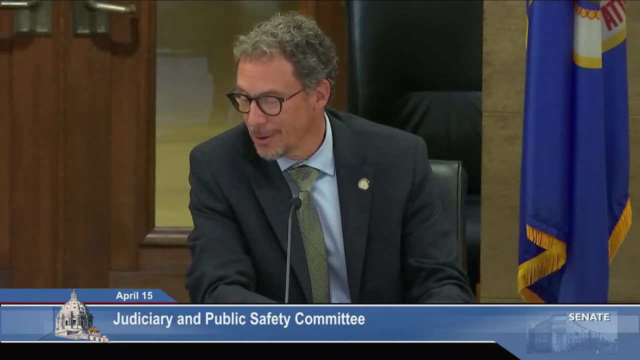 Mr Chair, I think your staff passed out the wrong bill. This one's on human breasts. Yes, Senator Loomer, the correct bill is being passed around now. Okay, Are we going to be hearing? We are. This is the only bill. 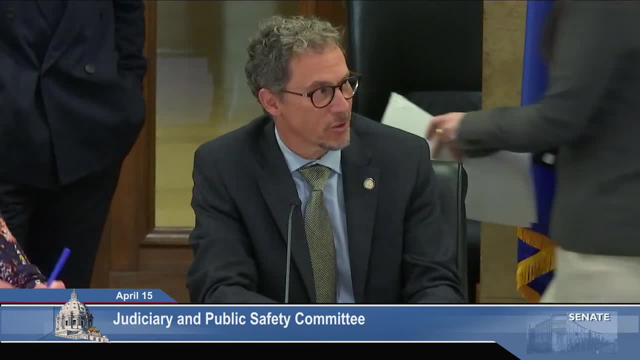 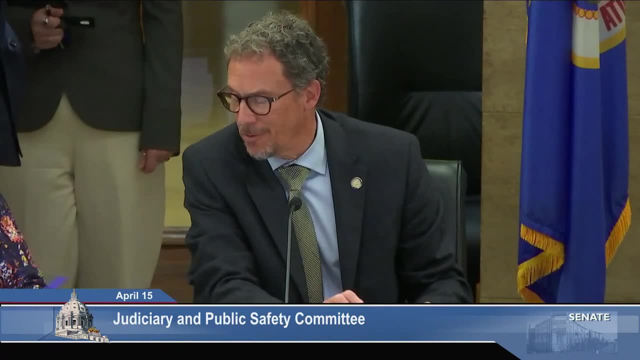 that we're going to be hearing yet today. Nothing else that was on the original agenda is going to be considered today. All right, Thank you. So Senate File 5243 for an informational hearing. Senator Herr, why don't you take a few minutes? 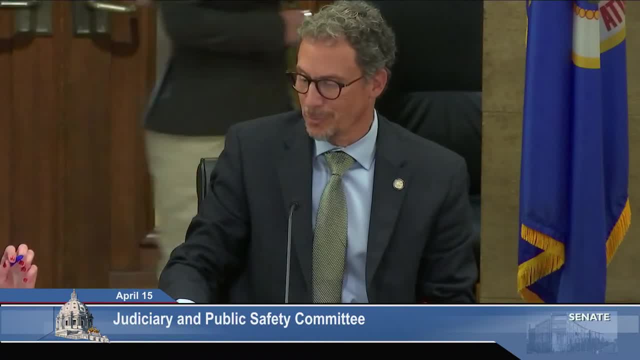 to tell us what this is about. Thank you, Chair Latz, for making it possible. I know Eastside St Paul is not far from here, but we have community members together and it's a little difficult to organize them to come back. 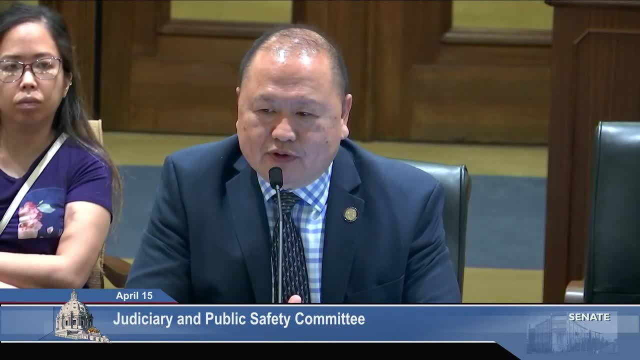 so we'll seek this momentum and thank you for allowing us the time, And I wanted to also thank co-author of the bill, Senator Ulmer Badum and Senator Limmer, And I think Senator Kroon just reached out to me that he'd like to be on the bill as well. 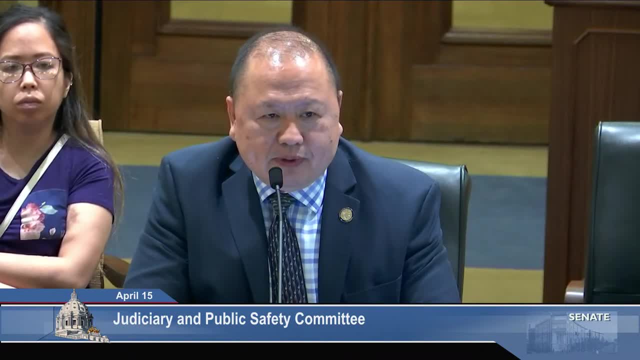 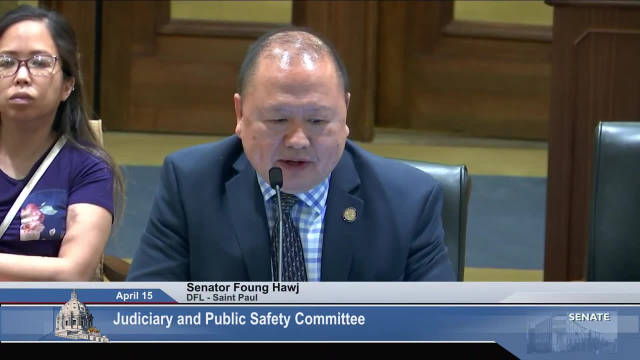 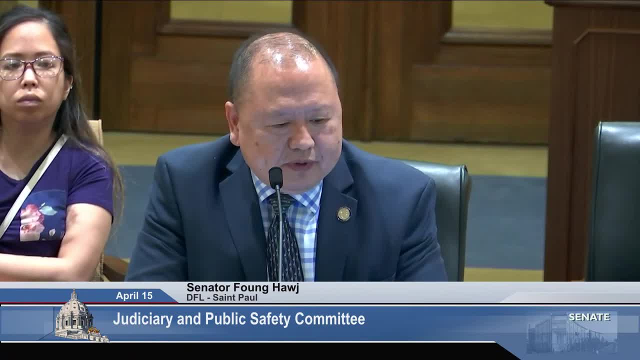 Thank you Great, I'll see if there is room. I think there is room. So this bill is asking for funding for fiscal year of 2025 from General Fund to the Department of Public Safety for a grant to the Hmong-American Mediation Center. 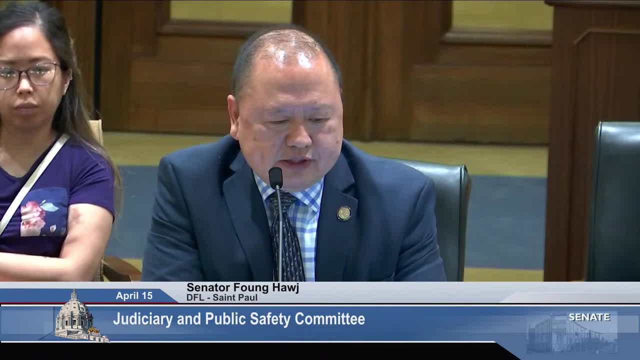 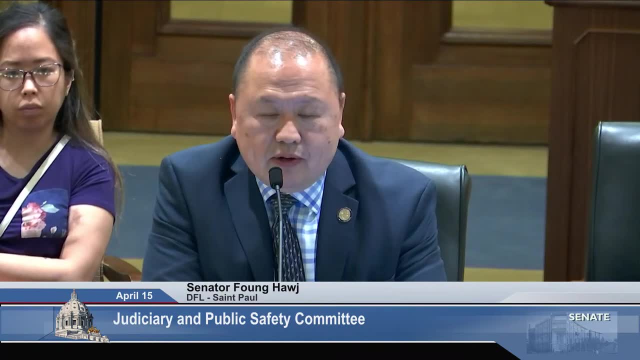 to provide mediation and restore the justice services. The Hmong-American Mediation Center has a long history of settling disputes in the Hmong community, both culturally but moreso following the referral and of our courts and guidelines, Their service on conflict and resolution. 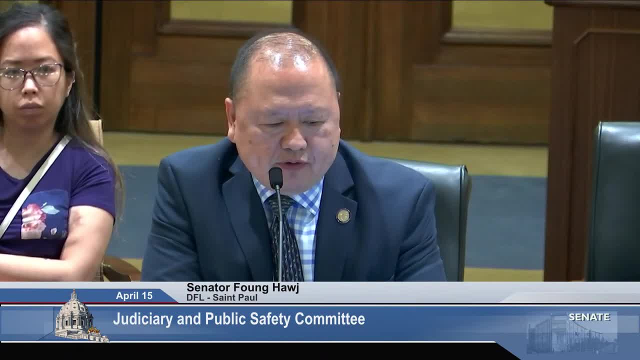 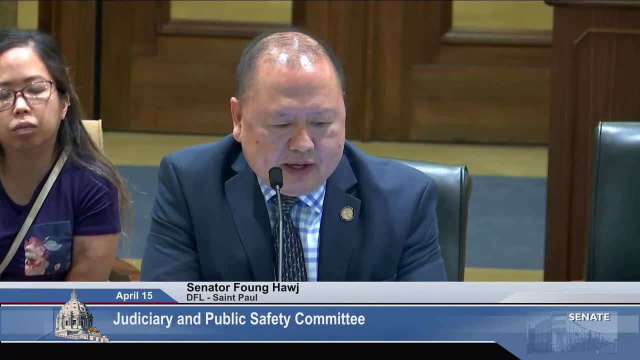 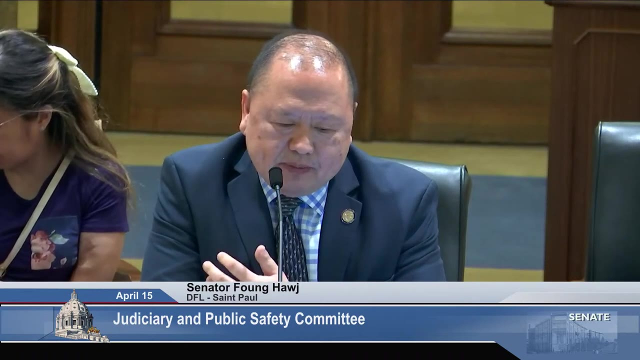 involve family dispute, juvenile and family restoration, family counseling and divorce mediation. When I testified here, Mr Chuvu came to me. Director Chuvu came to me with this proposal. He reminded me that still in our culture, in my Hmong culture, 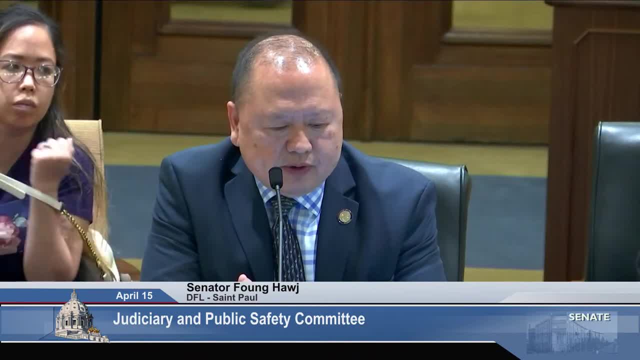 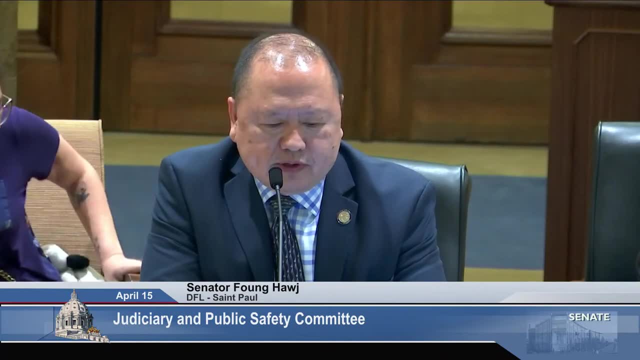 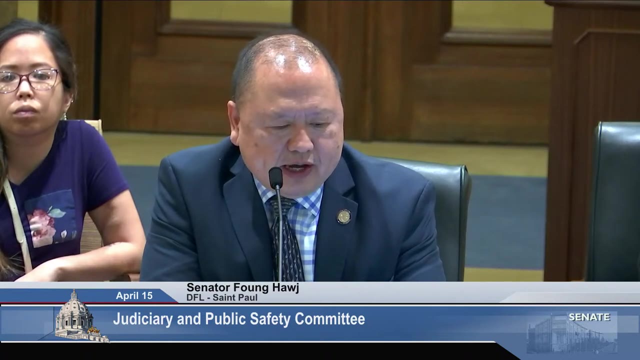 when two people are married, they're not married within themselves, but they're married two families together. so resolving dispute within culture could be a little complicated. So a center like the Hmong American Mediation can be a good resource to the community to resolve dispute. 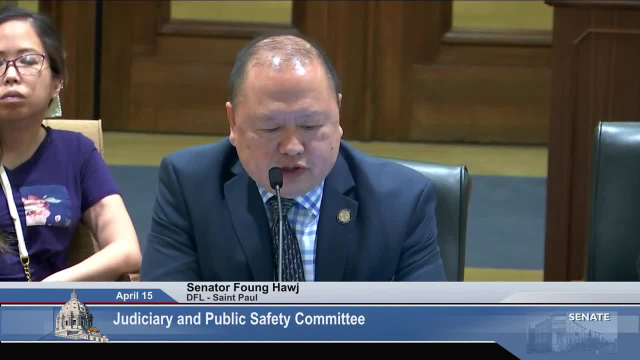 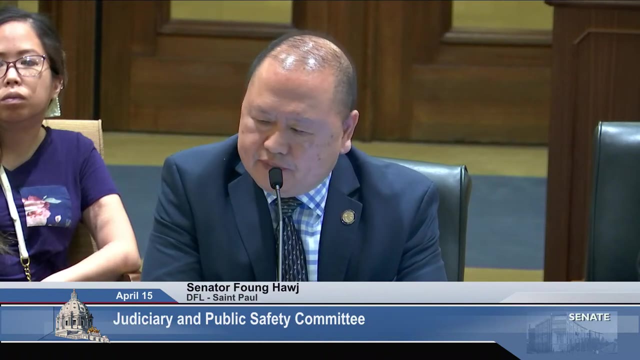 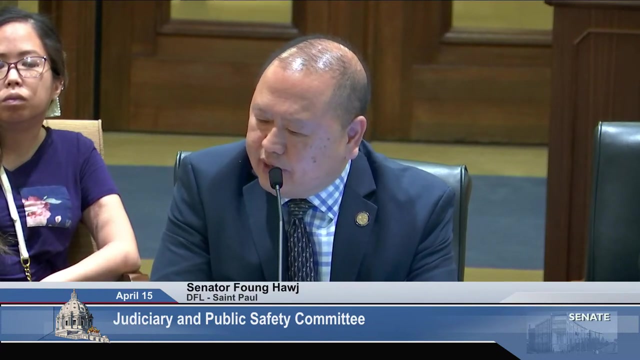 Their backlog continues to grow. In addition to small foundation dollars that they have and event fundraising toll operation, the Hmong American Mediation Center is asking for state support to get them going so they can reduce the backlog that they have. And so I have with me. here is Executive Director. 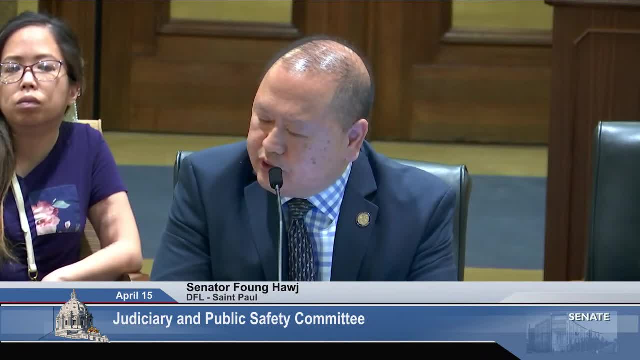 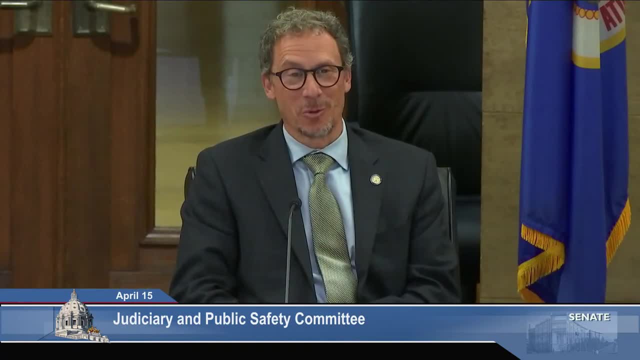 or also President of the organization, Mr Chuvu. Mr Chuvu, welcome to the Senate Judiciary and Public Safety Committee. If you could go ahead and state your name and present us with your testimony? Good afternoon, Chair Lutz. 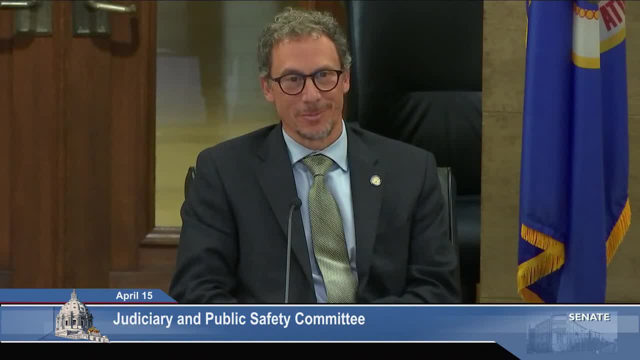 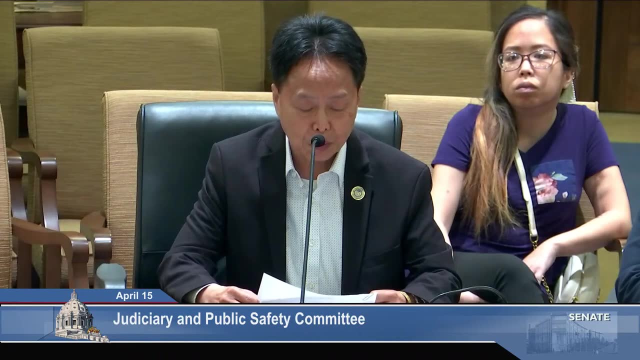 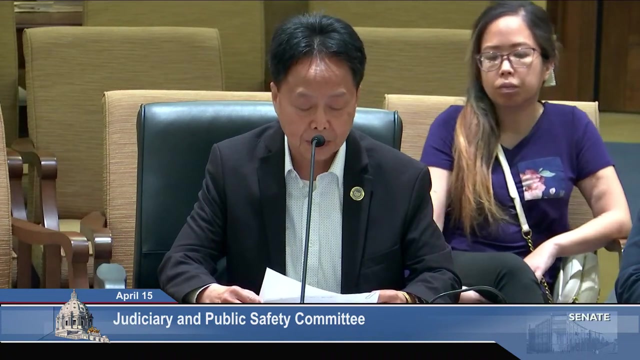 and members of the committee, And thank you, Senator Hull, for authoring our bill. My name is Vu Chu. I am the founder and Executive Director of the Hmong American Mediation Center. Thank you for the opportunity to share with you my testimony. 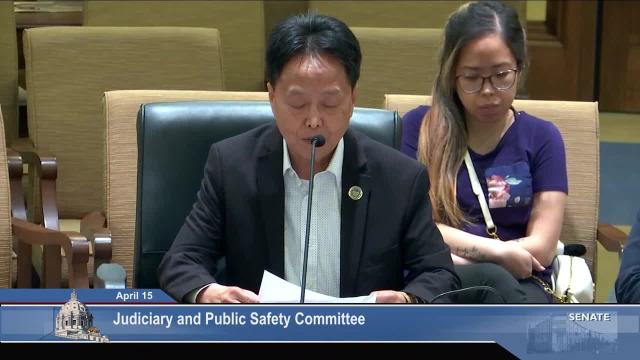 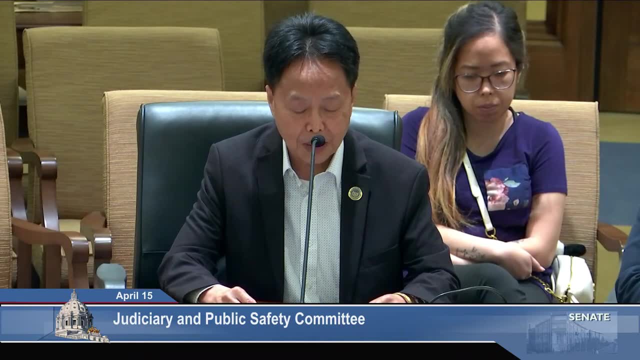 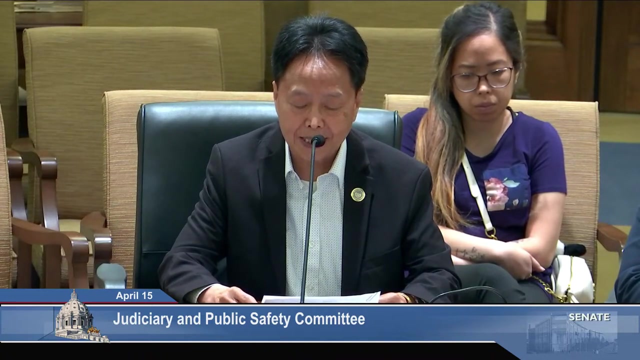 In support of Senate File 5243,. through the direction of the late General Wang Pao, I was appointed as the founder of the Hmong American Mediation Center. I am here today to ask you to support this organization because it plays a vital role in the Hmong American Mediation Center. 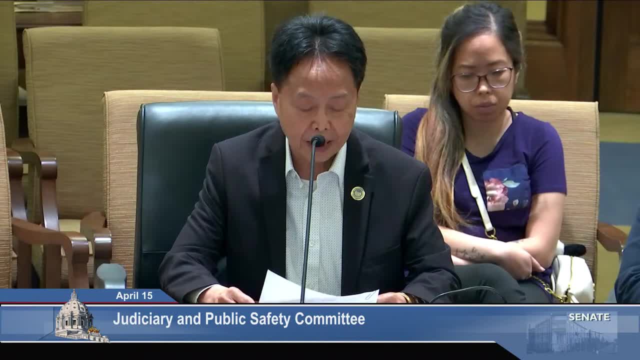 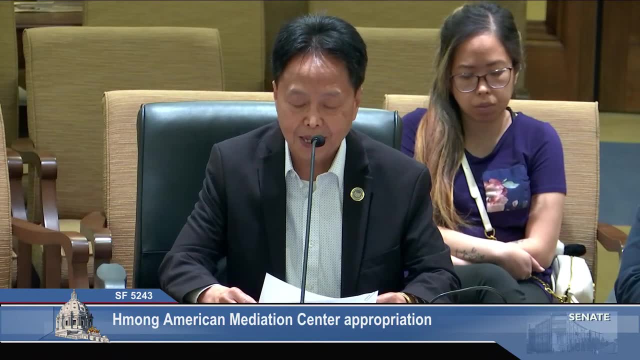 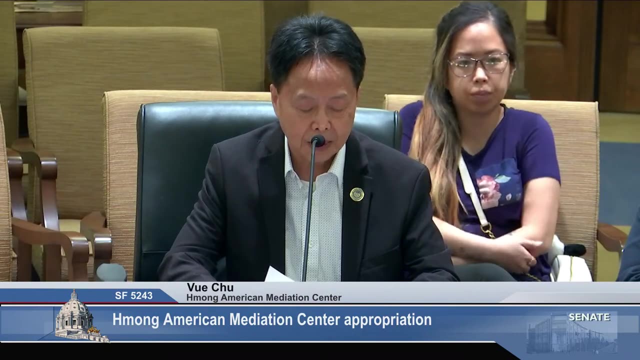 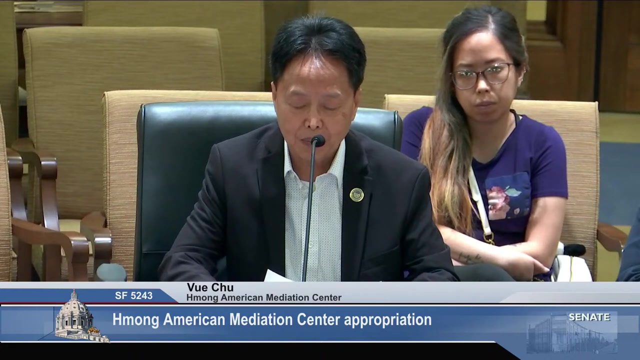 Thank you. Thank you, Senator, in the Hmong and on the Southeast Asian everyday life experience as they are dealing with our legal and law enforcement system In 2010,, when Hmong clan leaders started declining to help mediate family and clanship conflicts. 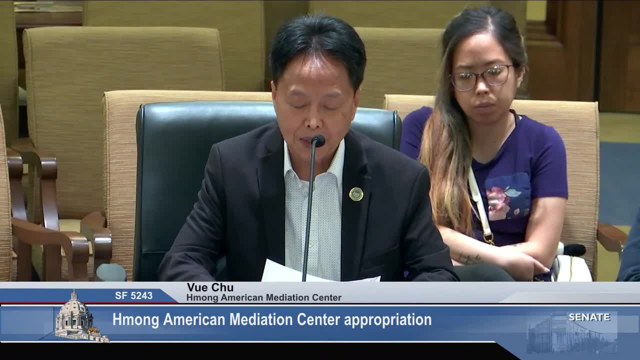 and problems within the Hmong community. the conversation of how to bridge the gaps between cultural and ideological differences and legal mediation began dialoguing To address this issue, the late General Wang Pao appointed me to develop a means to help mitigate the issue. 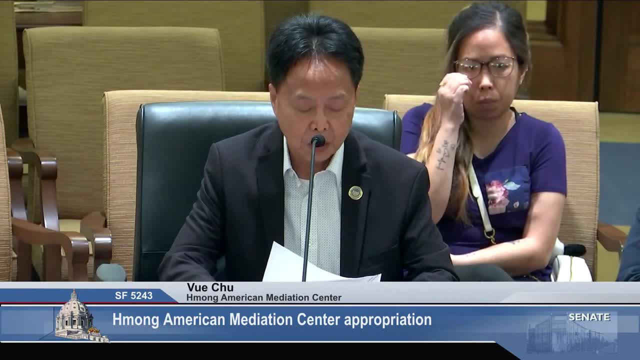 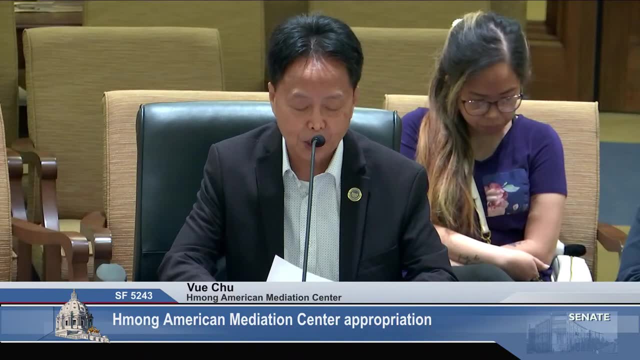 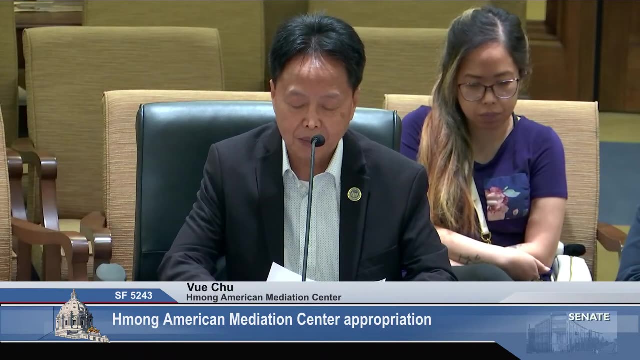 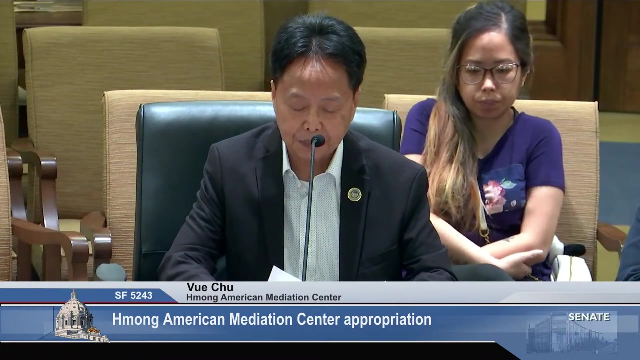 The issue facing our community. With the cooperation and support of our state and local law enforcement agency, Ramsey County judges, State Judicial Department and the professor at Hamlin University School of Law, as well as Hmong community leaders, the Hmong American Mediation Center was organized. 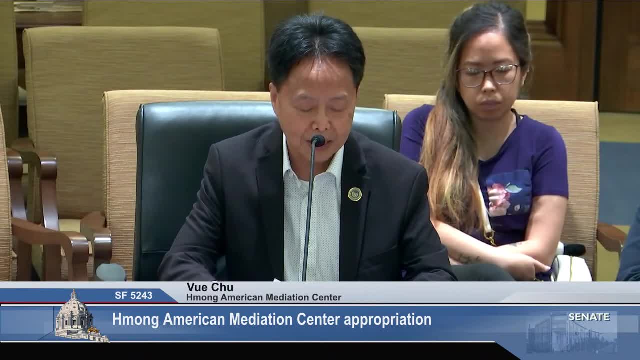 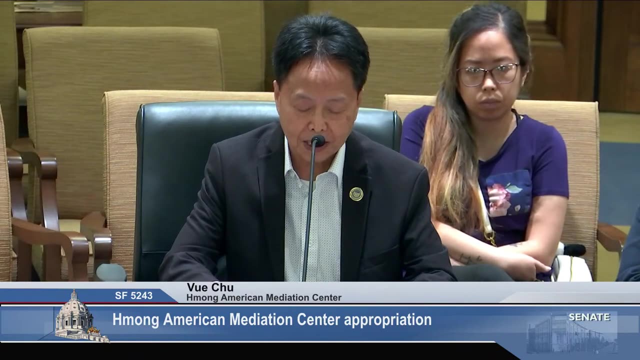 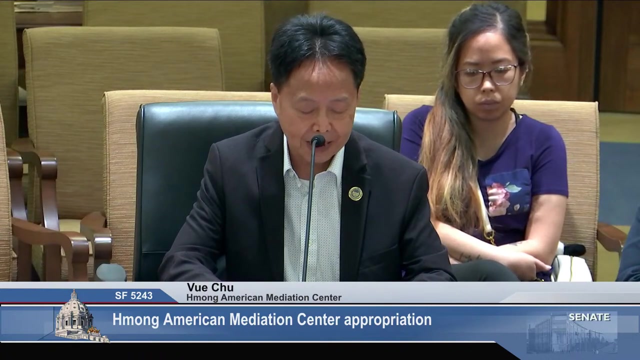 to provide cultural-specific family conflict resolution for Hmong and later include all the Southeast Asian community. At first the Hmong mediation and arbitration was incorporated as a program for the Mediation Center at Hamlin University. Training for meditators started immediately for Hmong leaders. 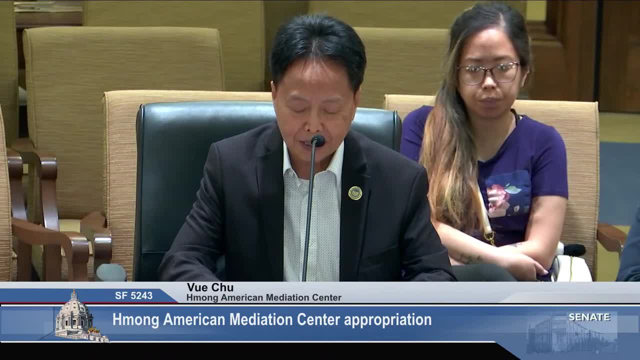 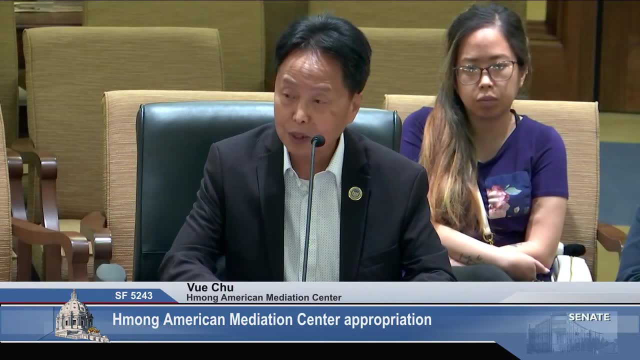 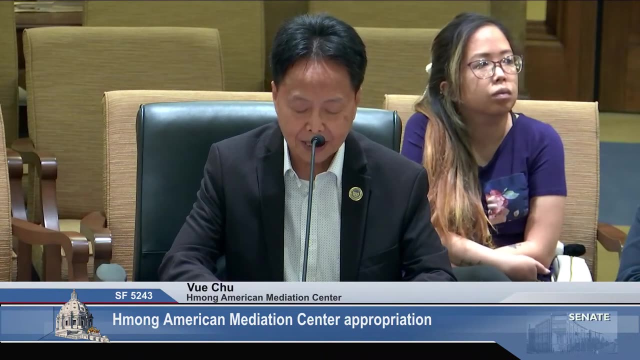 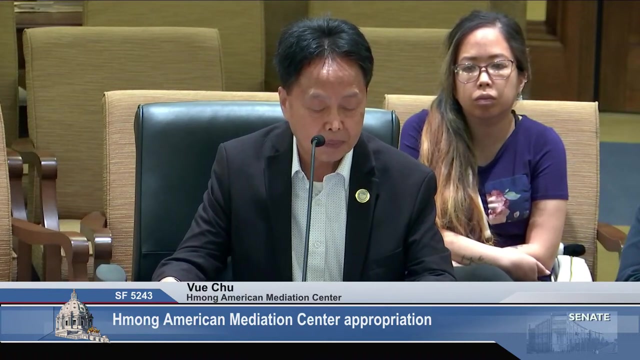 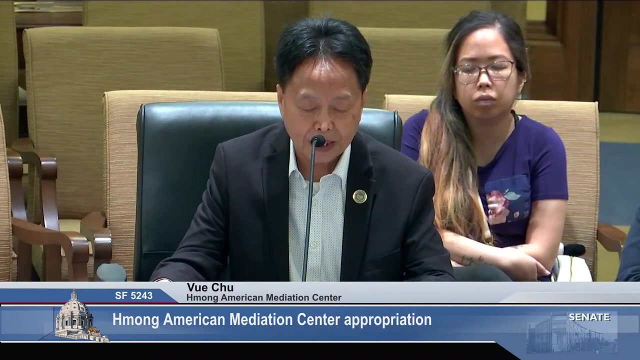 Hamlin University professors and attorneys and judges. The Hmong American Mediation Center officially launched on November 23, 2011,, when it was fully incorporated as a non-profit organization. Hmong American Mediation Center mission objective: offer alternative to going to court for Hmong and other Southeast Asian. 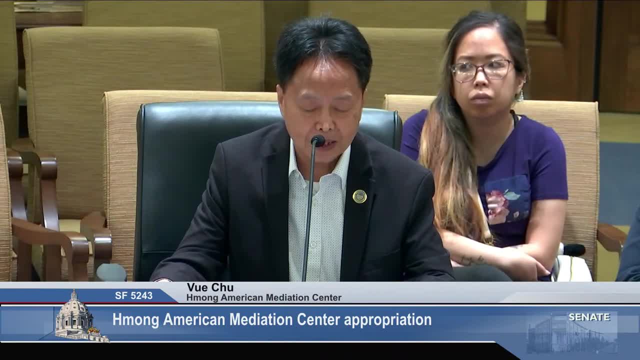 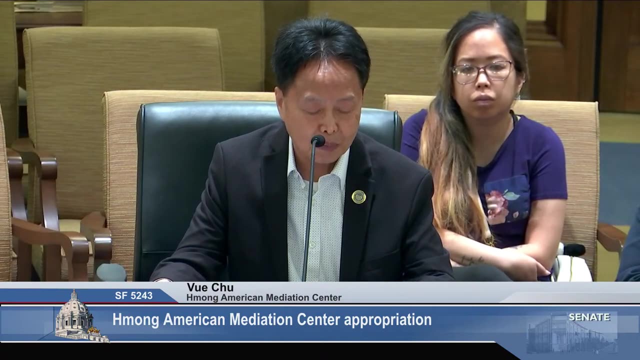 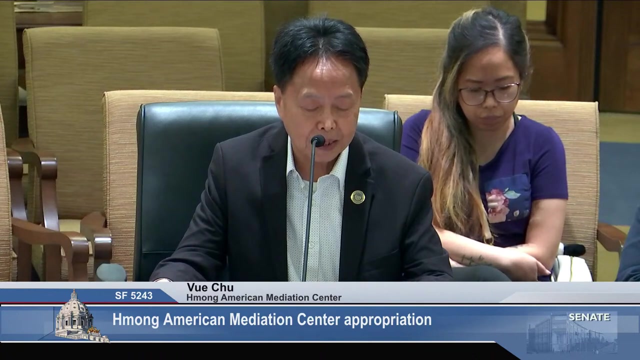 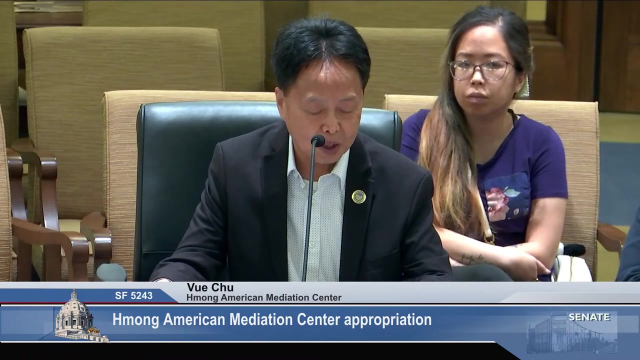 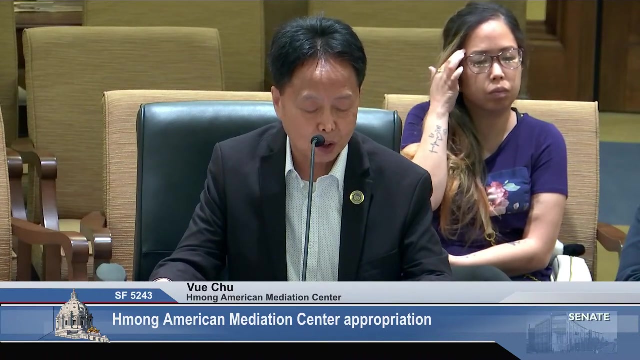 strengthen Hmong and other Southeast Asian family through cultural connection to reduce divorce, reduce domestic abuse, reduce tragedy happening to the Hmong community and reduce juvenile crime. Provide education to the legal and law enforcement system about traditional versus court system. Assist Hmong and other Southeast Asian to work within the Minnesota court system. 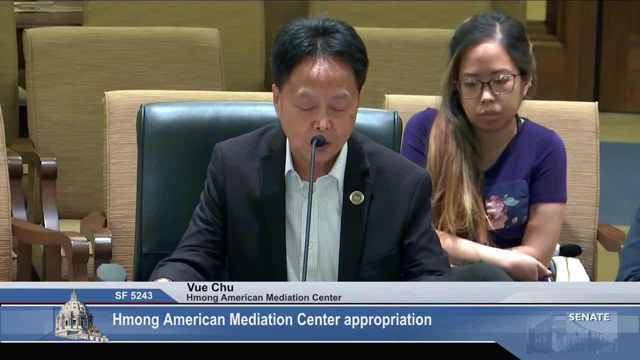 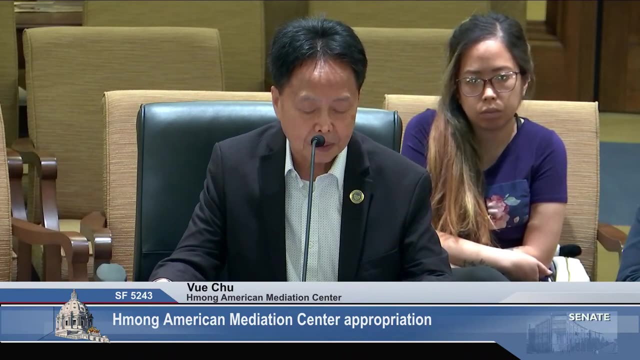 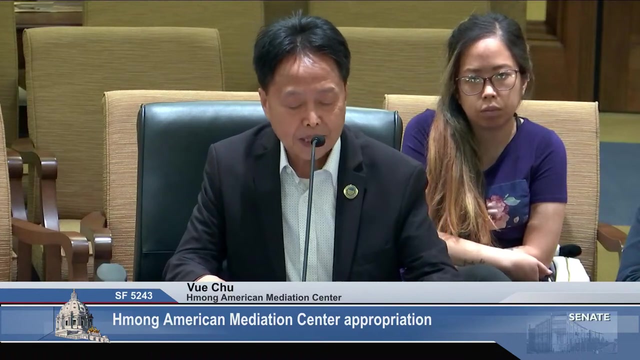 To preserve Hmong and other Southeast Asian cultural value, building bridge and partnership between Hmong and other communities. Hmong American Mediation Center provide the following service: family mediation, civil mediation, arbitration, juvenile and family restoration case management. Hmong American Mediation Center serves hundreds of family conflicts. 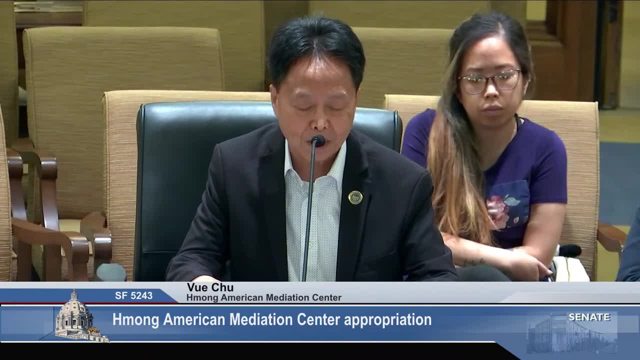 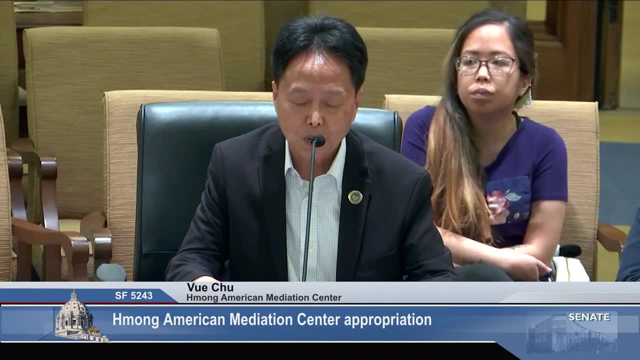 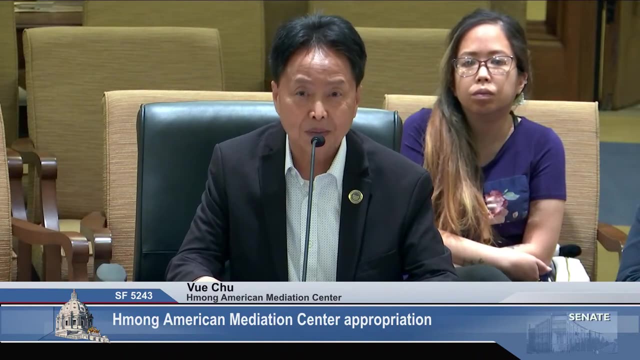 and restorative of justice service for juvenile in each year. Thank you for your time today and hope for your fully support the organization, Thank you. Thank you, Mr Chu. Senator Hurt, do you have another testifier? Do you have another testifier you want to present? 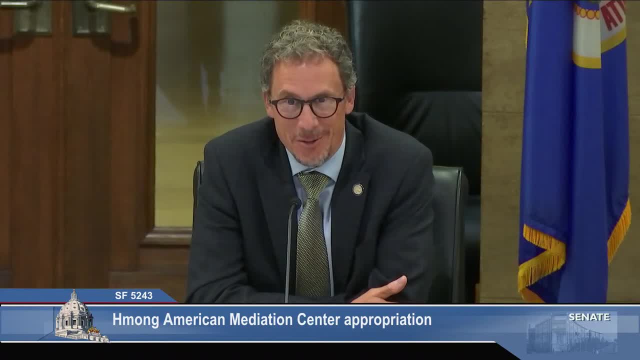 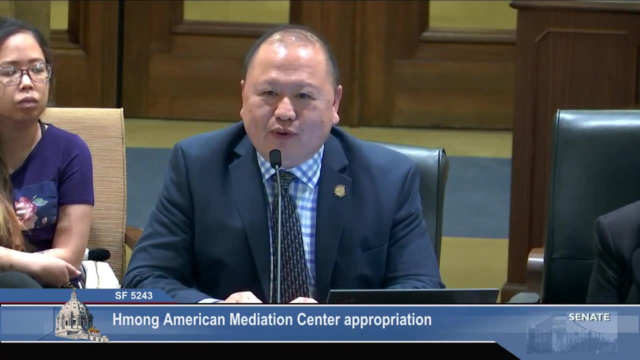 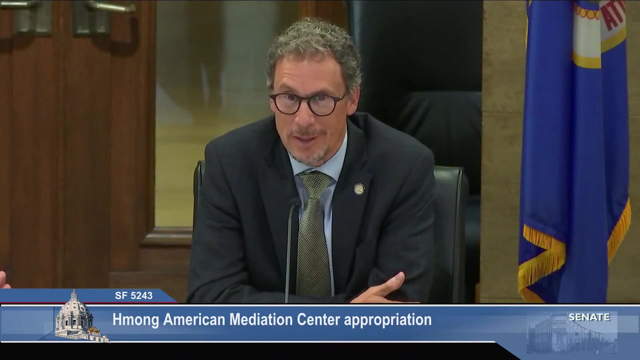 Or is she just available to answer questions? Ms Hurt, here is fine without testimony, but if a question arise, she will be happy to answer. Thank you, Is there anyone else in the room wanted to testify in connection with this proposal? Any questions or discussion from members of the committee? 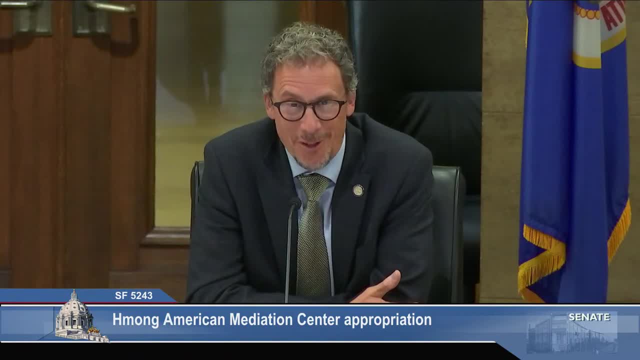 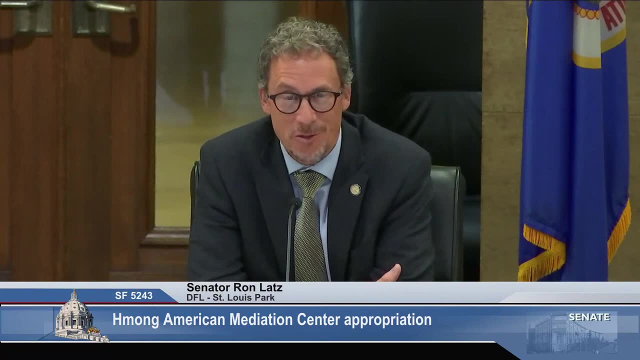 I'm not seeing any at this time. Well, this is sort of a general announcement or statement. As Senator knows, we've been given very limited supplemental funds for this spring session. here We have very limited money available to us. There are certainly going to be worthy causes and organizations that are not going to be able to be funded this year. 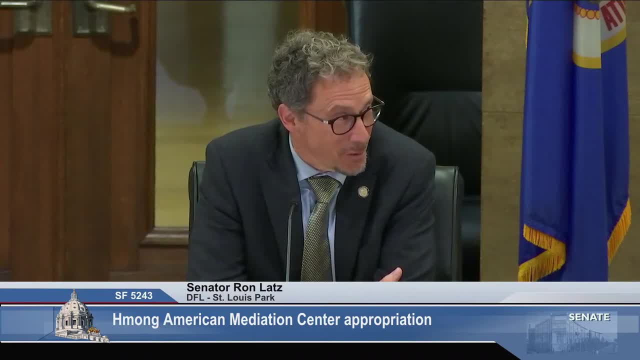 We have not made those decisions yet, but we will be by Friday. We'll be passing our budget out. So it's been helpful to me and I appreciate you coming forward to share the information with us. Thank you, Senator Letts and members. 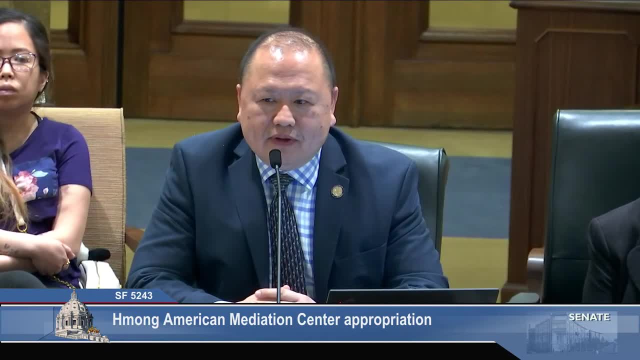 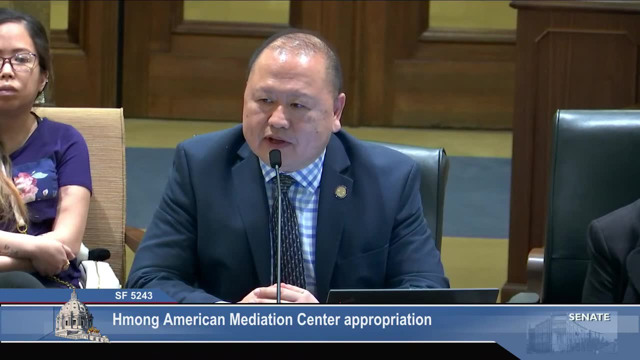 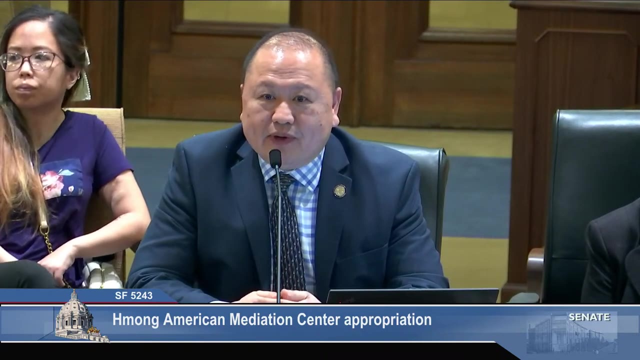 We are at your discretion on this. I have seen the progress and the effectiveness of the Mall of America Mediation Center, and so I know this is late in the game, but it doesn't hurt to submit a request and see where it goes.